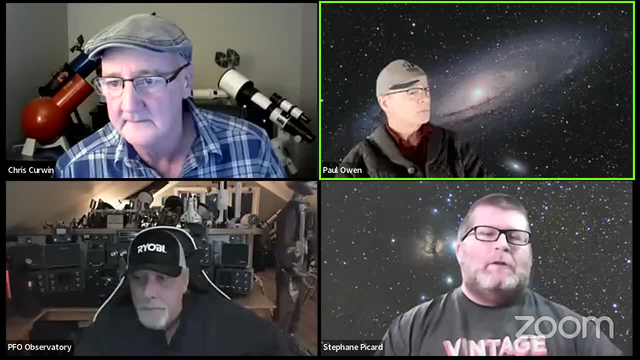 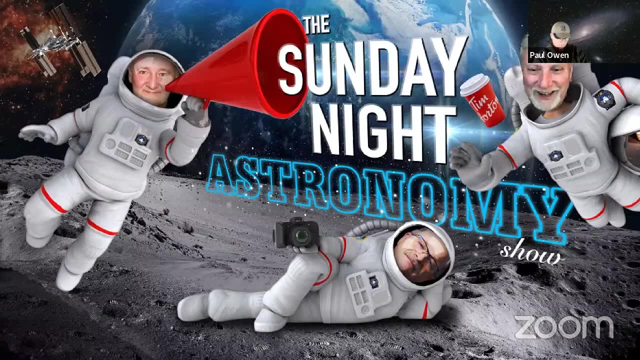 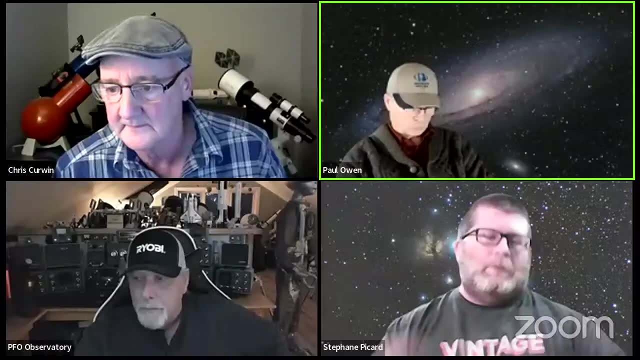 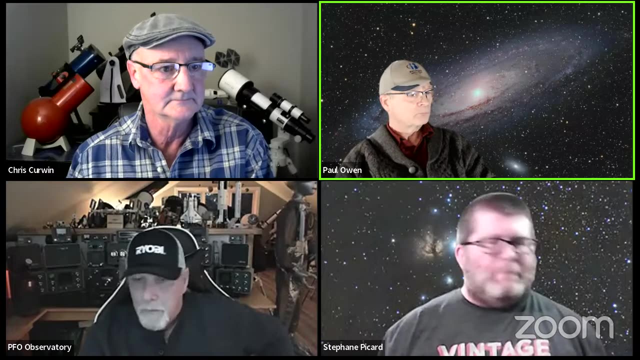 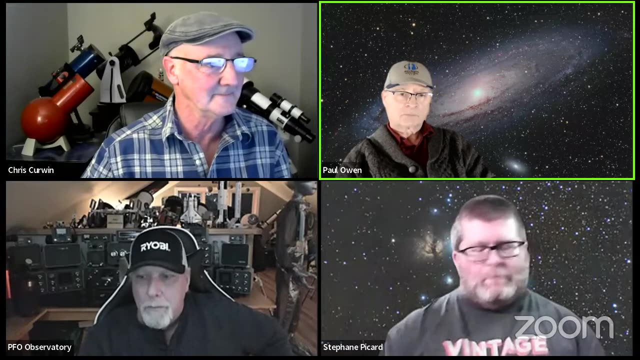 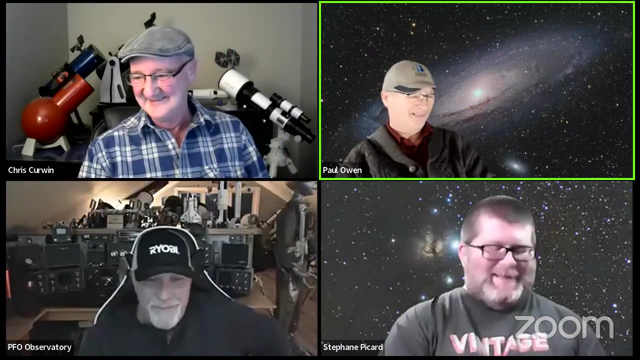 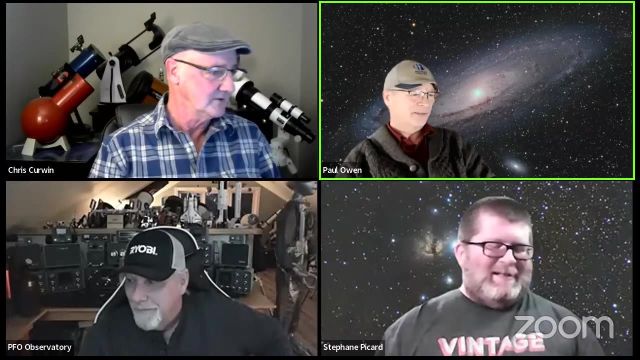 Right now. Okay, go ahead, Paul. Thank you. Okay, let's try it again. Are we live? Thanks, Thanks, Term number three. Let's try that. Okay, Hey, we're back. I don't know. 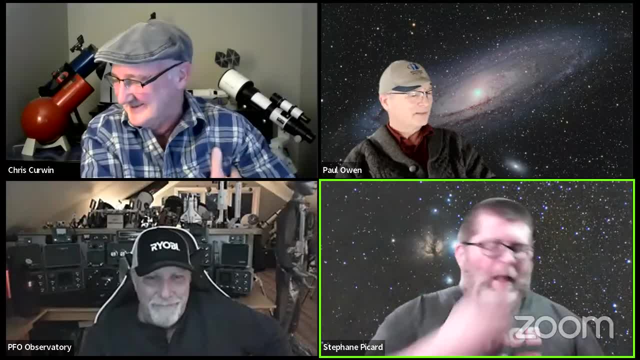 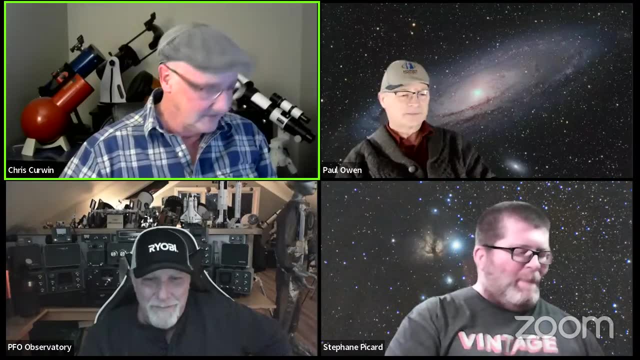 Have we ever left? I hope we did Very good cursing going on there. It looks like we're up and running now. Okay, Good evening everybody. We're a little bit late but we apologize for that. But that's technical glitches and that's what happens when you go live. 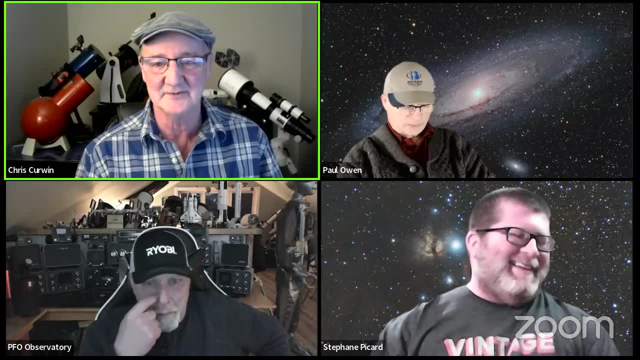 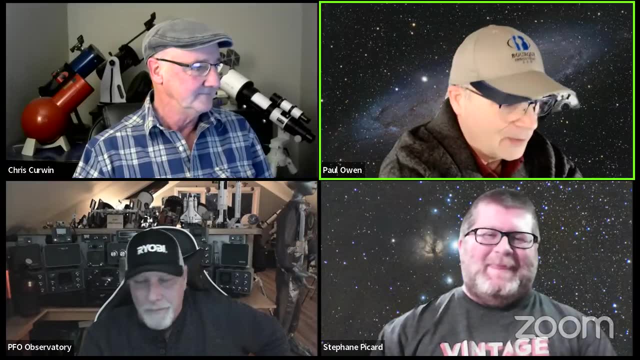 Sometimes, Not always, but maybe we should record the show from now on, Wouldn't be a bad idea. I think sometimes It's mostly me, but We're here, That's the main thing. We're here, That's the main thing. 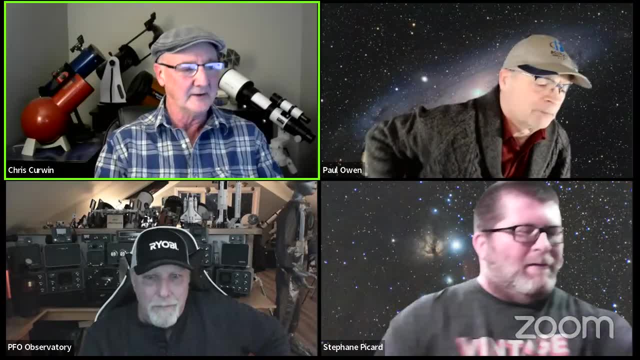 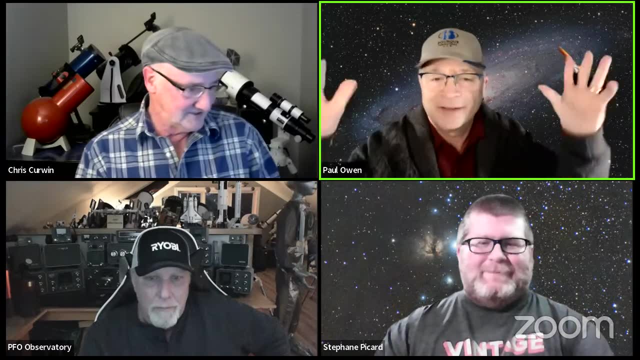 We're here, That's right, Okay, Well, good evening everybody and welcome back to our Sunday night's offering of Astronomy Outreach for March the 26th: the Sunday Night Astronomy Show. Yay, Yay, Yes, right along, Derek. 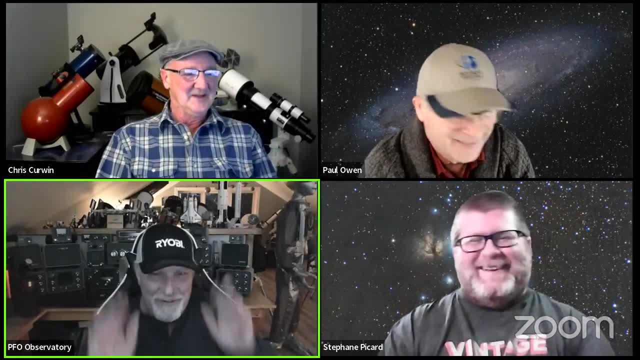 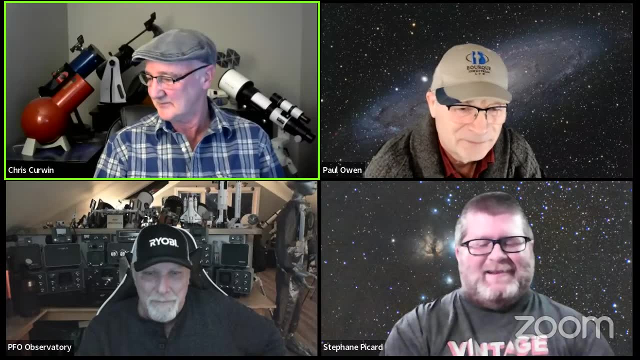 I have to go back in the league with those old ones. Okay, My name is Chris Burr and I'm your host for this evening and creator of the social media channels known as Astronomy by the Bay. I'm an amateur astronomer and a member of the Royal Astronomical Society of Canada. 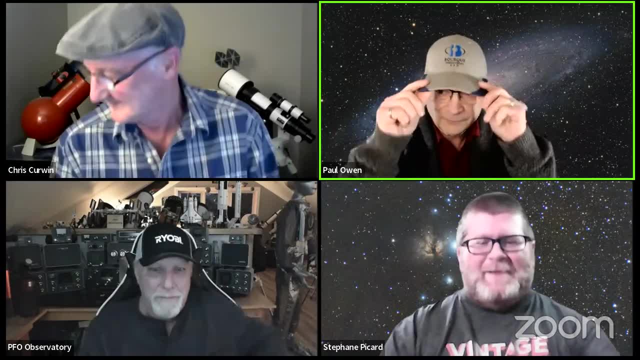 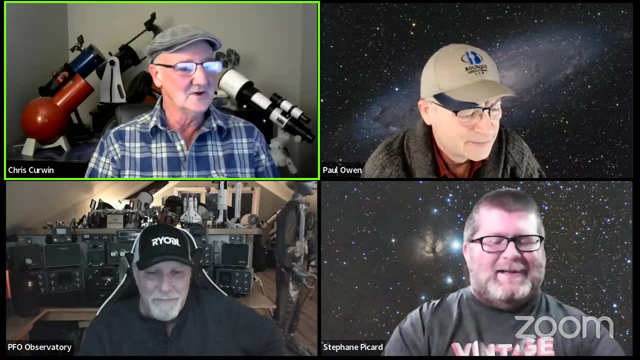 And the St John Astronomy Club. Yay, Yay, A little solar player activity. That might have been the reason. First of all, I'd like to welcome back our two regular co-hosts for the Sunday Night Astronomy Show: Mr Paul Owen from the Moon Shadow Observatory here in beautiful Hampton, NB. 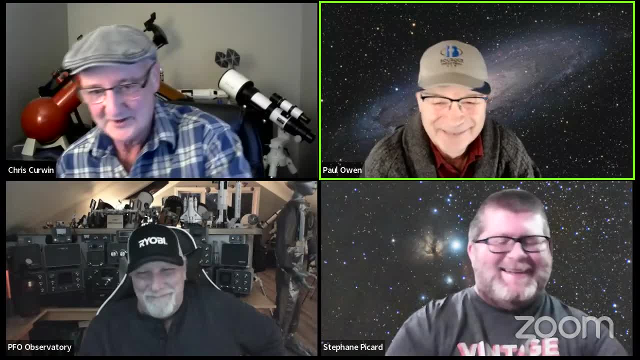 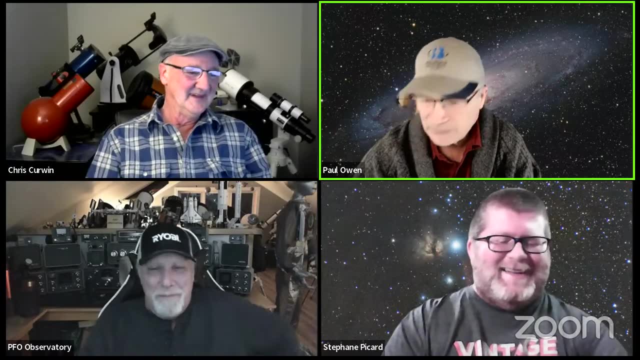 Well, there in beautiful Hampton. Hey, Paul, Time for another drink of coffee. Yeah, me too. I think you need more coffee. I love to drink coffee. And our other regular co-hosts- Our co-host for this evening here in the program, Mr Mike Powell from the PFO Observatory here in beautiful St John. 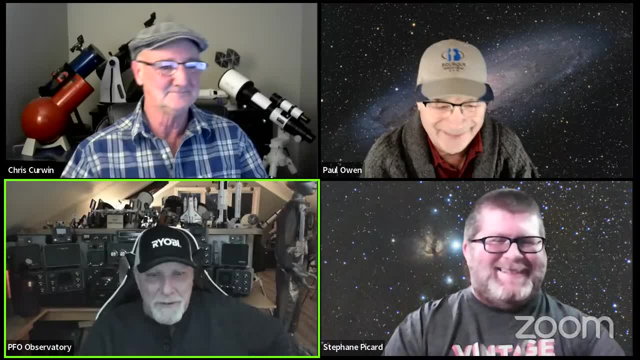 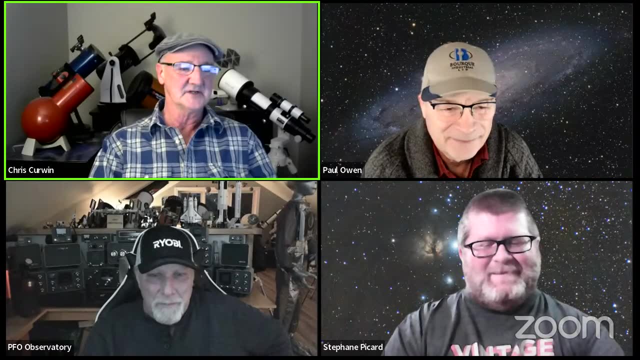 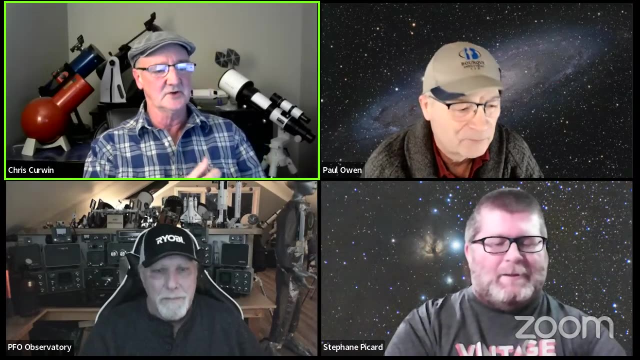 Welcome, Mike. Two hands Okay On tonight's episode of the Sunday Night Astronomy Show. today's modern astronomers have made significant discoveries, helping us understand the true nature of our universe, From their explorations of dark matter to their quest for determining the age of the universe. 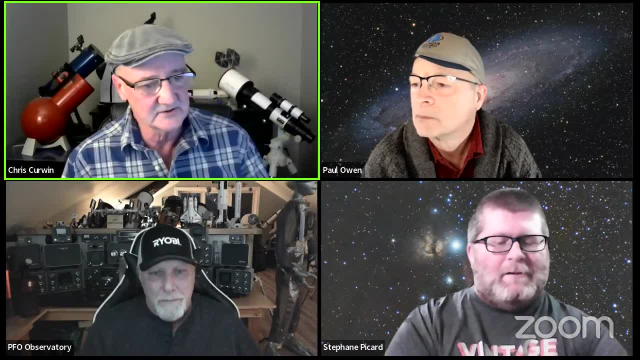 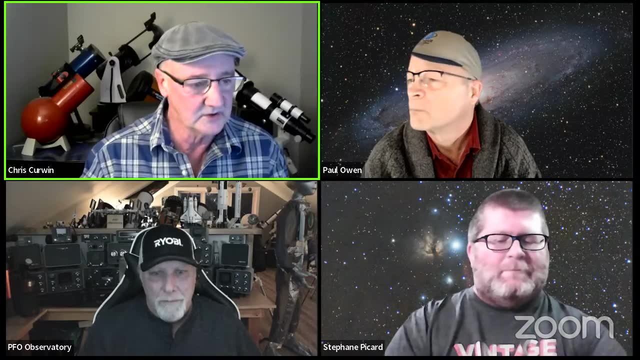 and like many of those in other professions, today's astronomers stand on the shoulders of giants. Today we're going to pay a tribute. We're going to pay a tribute to a couple of them and how they helped influence what we know about our universe today. 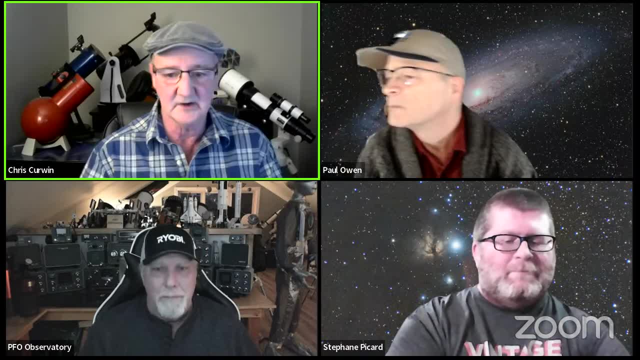 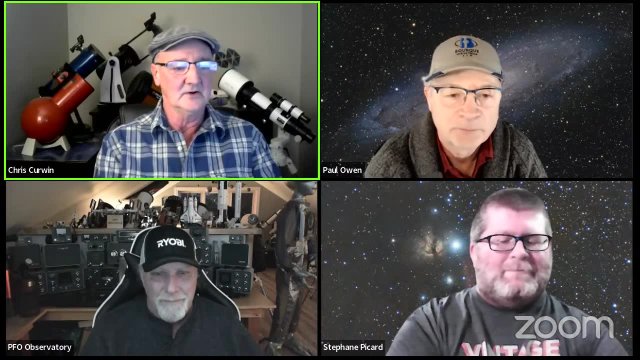 Also tonight, Mike will be bringing back a vinyl bud for another fine binocular target of the week. Paul will be introducing another Rosanna's fun fact for us to enjoy. Yes, Okay, I'm going to have a quick look at what to watch for in the coming week and we'll have all of your wonderful photo submissions to share. 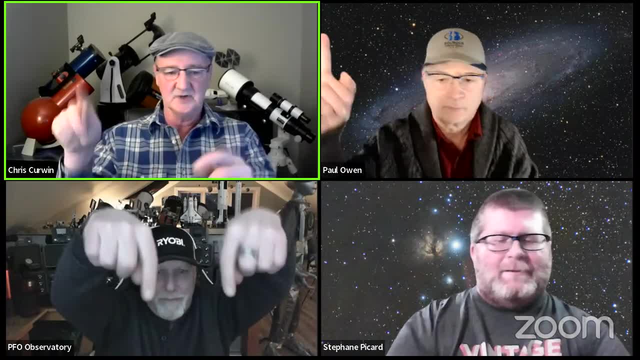 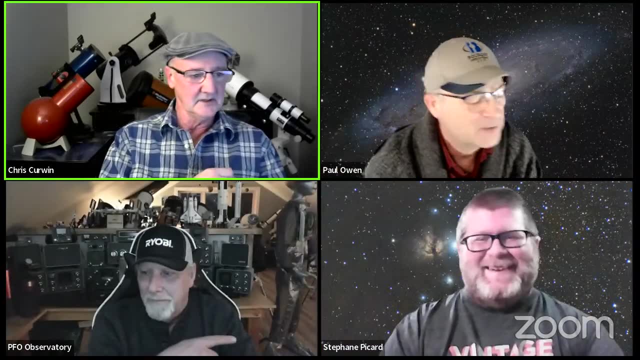 And also today we're going to be checking in with Stéphane Picard of Cliff Valley Astronomer. Hey, Stéphane, Hey guys, Hey, He's going to give us an update On his ventures into astrotourism and in the area, and also his 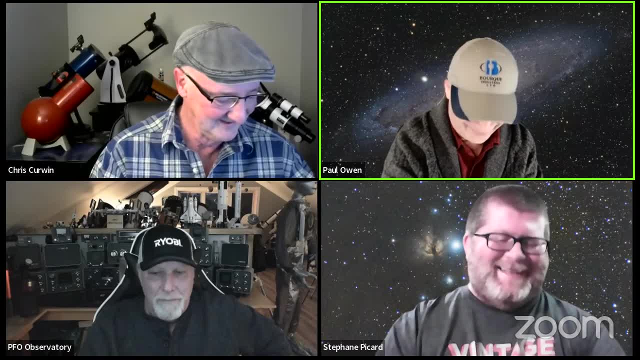 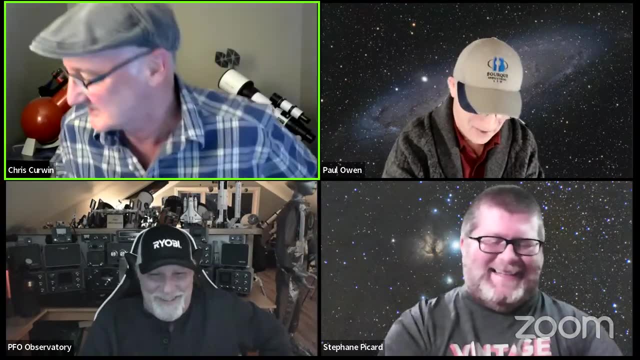 Hmm, I'm sorry, I'm just Nothing. Also, I have pills for that. His sky experience 2024.. We've talked a lot about that tonight. Oh, my goodness. Okay. So this is a family-friendly interactive live broadcast. 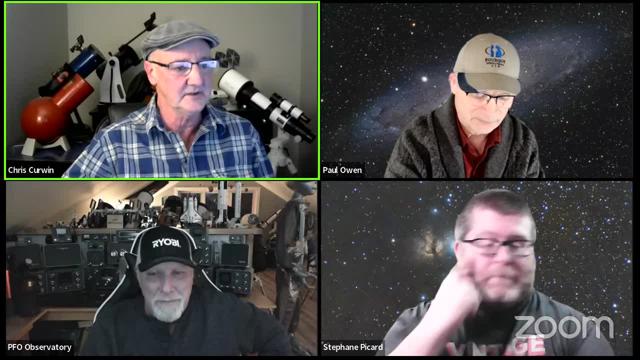 So, for those of you joining us from my YouTube channel or Facebook page, we are happy to try and answer all of your astronomy questions here in real time as well. Stéphane's going to answer them because he's a new guy, So we're going to have a little bit of a chat with him tonight. 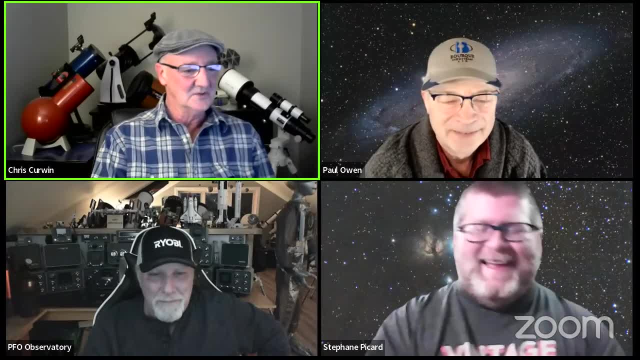 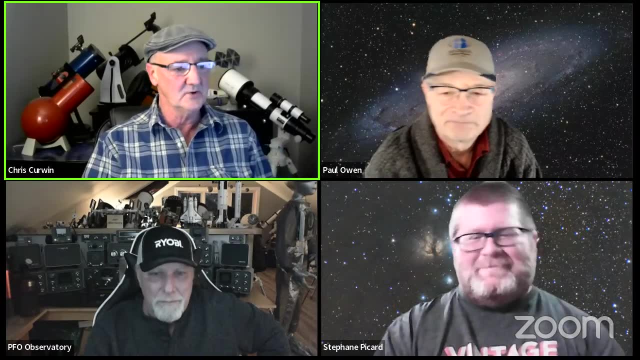 And, of course, we'd like to welcome back all of those who have been joining us through the local Rogers TV network. Thank you for your support, everybody. So let's get started, then, with tonight's program and a look at some of our favorite giants in astronomy. 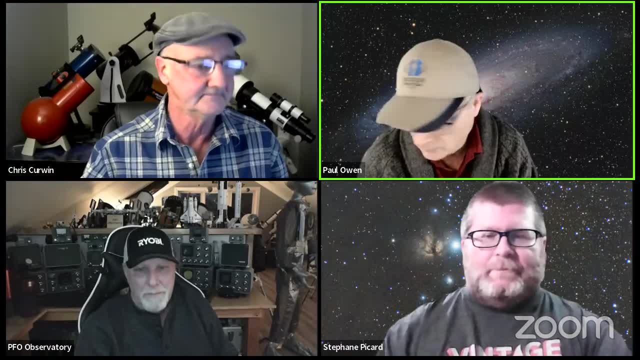 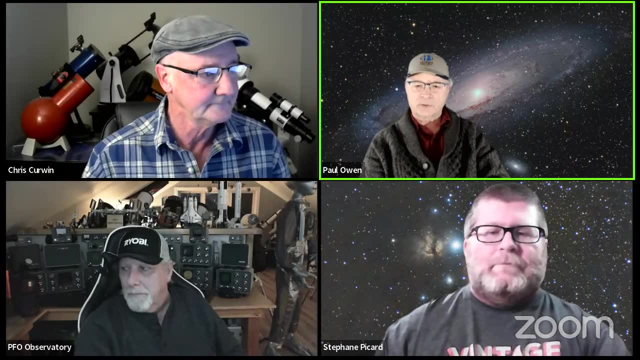 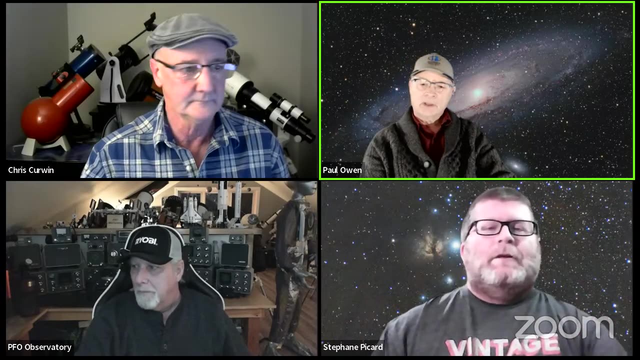 Paul, you're going to take up the first. All right, I will. I'm actually excited to talk about this gentleman. This guy has done so much for astronomy and it's unbelievable. And as I read more and more about this gentleman, it amazes me how much he's done. 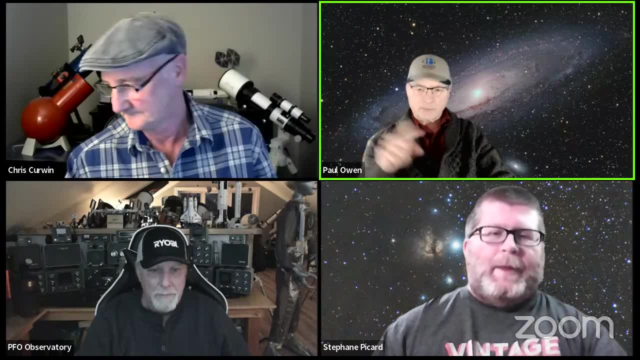 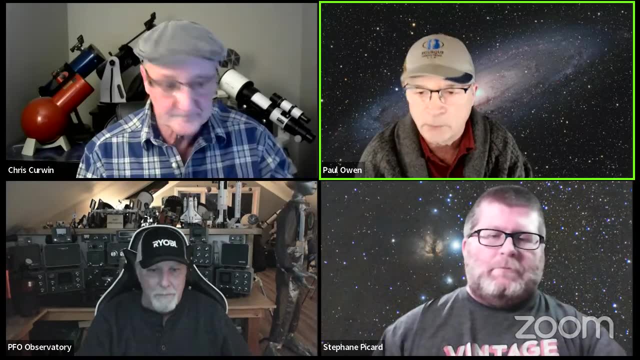 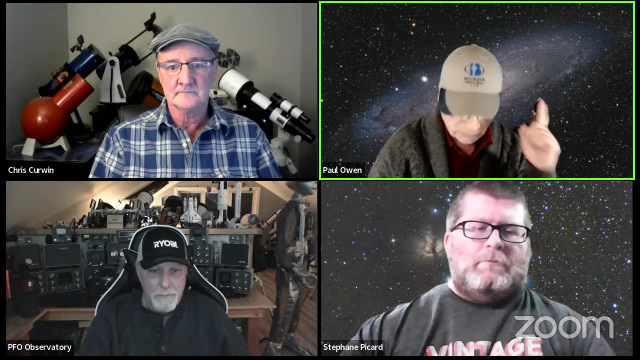 and how much we've seen him in his name but not realized who he is and what he's done. So I thought it'd be fitting, because last week when Kurt did his thing, we actually talked about who had the longest-running television show, And actually the actual title is who hosted the longest-running television. 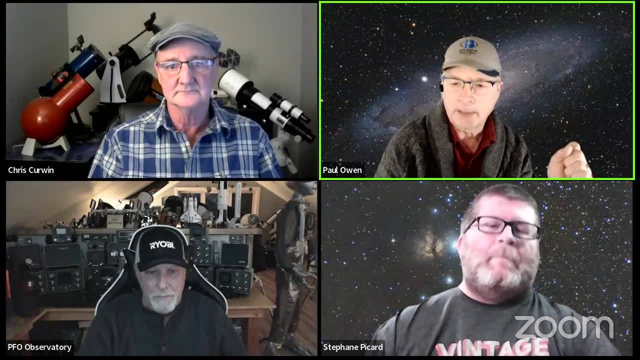 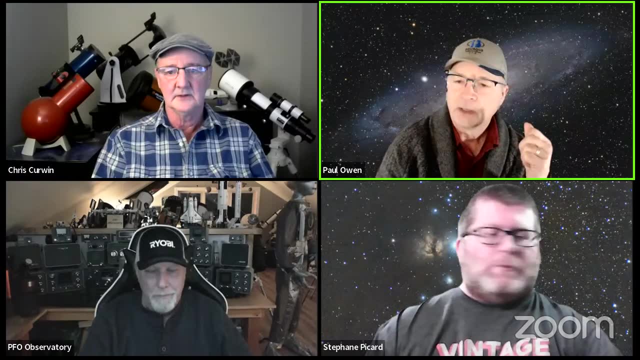 And it was Sir Patrick Moore, and he did it for 55 years. Wow, unbelievable 55 years, Can you imagine? No, Anyway. so I'm going to show a couple of pictures of him, just to kind of just have him up on screen. 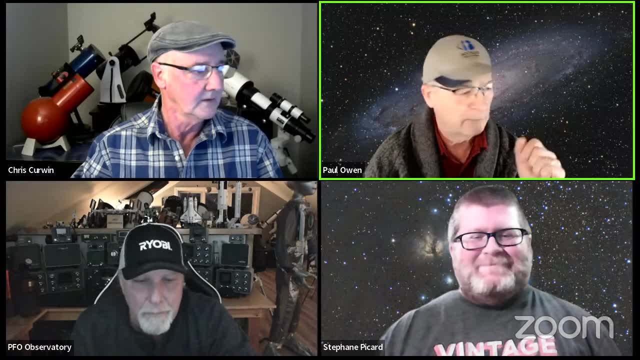 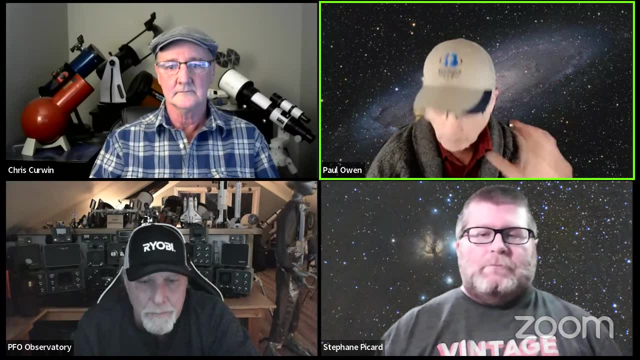 So instead of looking at us, you can look at who we're talking about. And then I'm just going to read some stuff from the Royal Society Publishing and all about Patrick Moore And they have a whole bunch of different. They have a whole bunch of different segments on them. 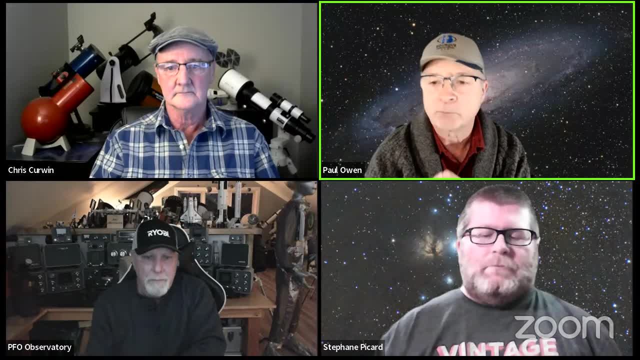 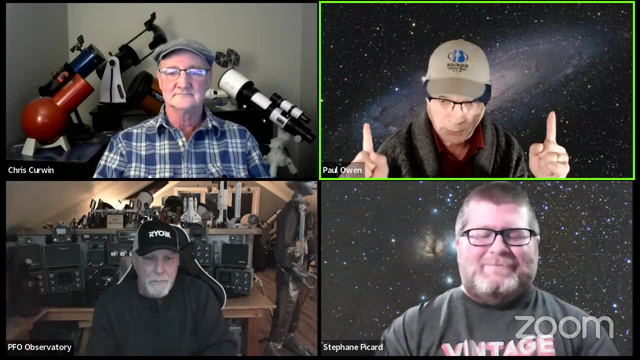 I'm only going to read a few, but the ones I think that are important And I told Chris earlier. I said, Chris, pay attention to this because you are going to see similarities in what Sir Patrick Moore did and what you're doing today. 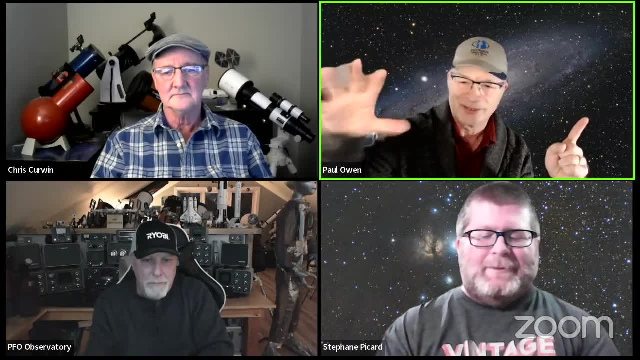 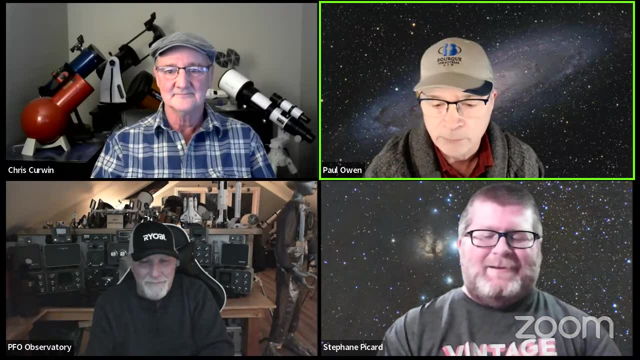 And the more I read about it, the more I could see Chris Kerwin throughout this whole thing. So, anyway, so this is really quite a story and I'm quite excited to talk about it, So let me just share my screen, That one there. 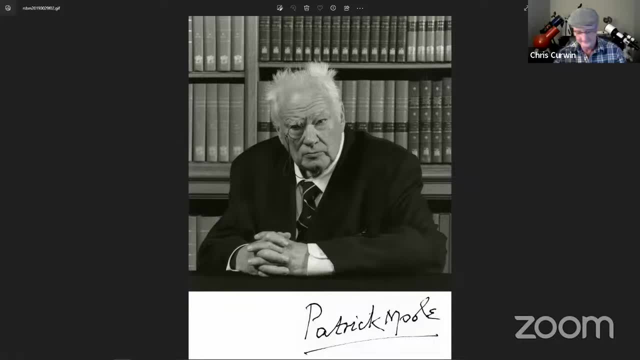 And let me know if you see Mr Moore on the screen. You do. I see Chris. Well, you might be. He's got to get a monocle, That's right. So this is Sir Patrick Alfred Caldwell Moore. He was born in March, the 4th, 1923, and he passed away in 2012.. 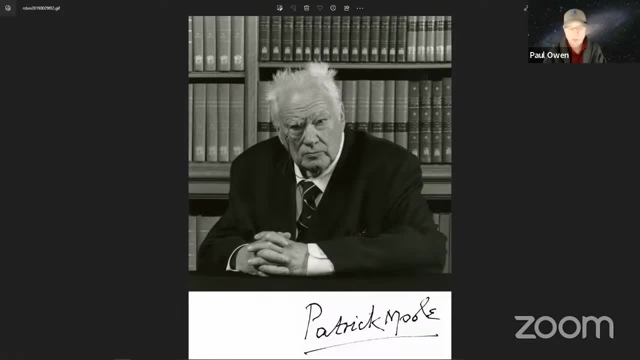 This guy has done so much. I'm just going to read you just a little Something that I found interesting. So here we go. Patrick Moore was the art, Yeah, the archetype of the English eccentric bringing a passionate enthusiasm for astronomy to the general public, principally through his long running television series the sky at night. 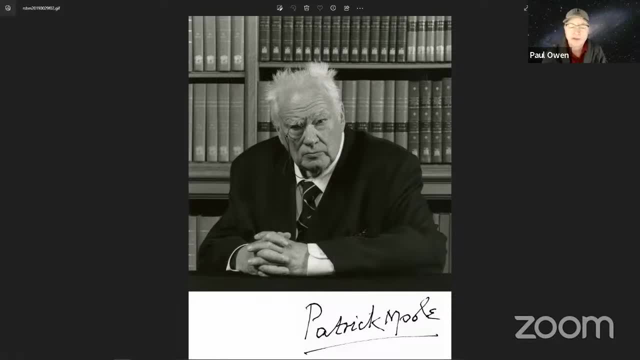 He was inspired. He was an inspired amateur who made no pretense at being a professional, but who had the extraordinary ability to communicate in simple, articulate and direct language the significance of the advances in astronomy and astrophysics to the general public. He inspired generations of young people to take 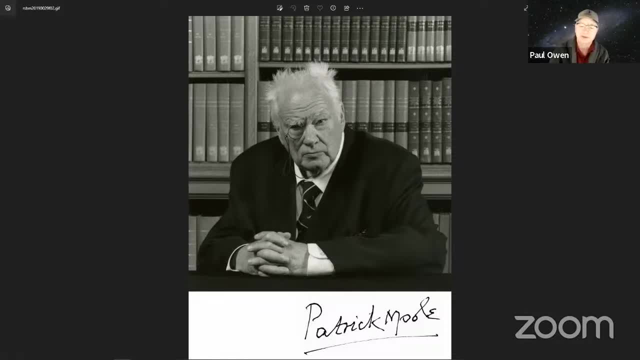 an interest in astronomy and in science in general. His passion was combined with a love of everything English, especially cricket. he was a great cricket player and political views which might have mildly described him as an extreme right wing, but anyway, in his early life, he actually was born on March the 4th 1923.. His father was an accountant and who had served in the in the 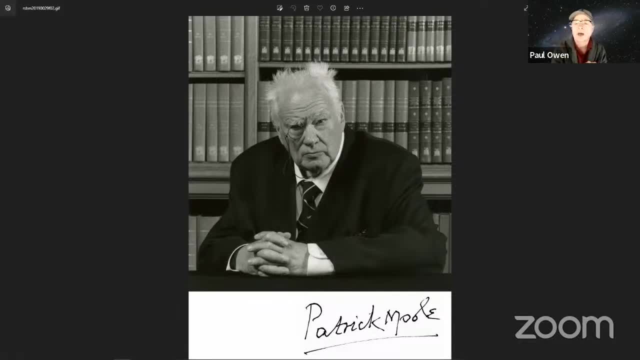 first world war and he got numerous medals for doing so- and his mother, Gertrude Lilliam- she was from London, she was actually a wealthy London solicitor and actually an amateur opera singer, which was kind of cool. maybe that's where Patrick or Brian May got his like for this guy, I don't know. but Patrick was baptized Patrick. 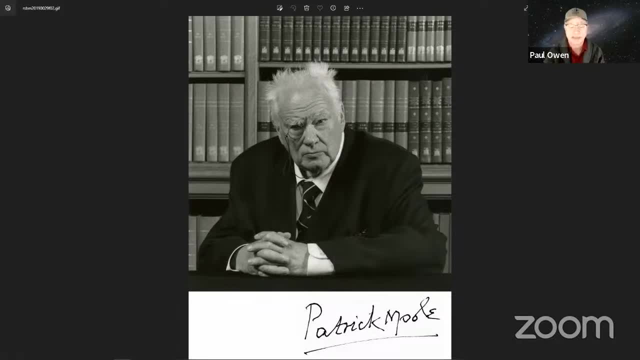 Alfred Moore. at some point in adulthood he actually added the name Caldwell- and I'll explain a little bit further the significance of that: initially as a middle name, later as part of a double-barreled surname, and also began giving his father's name as Captain Charles Caldwell. 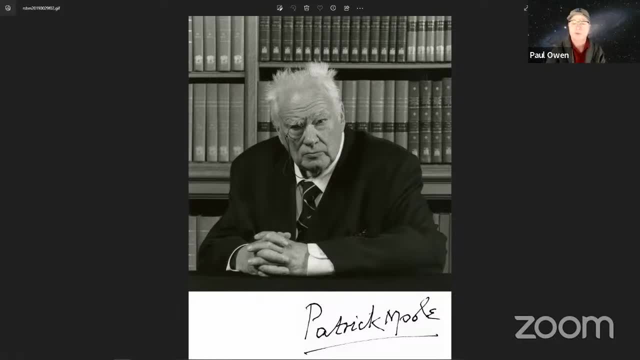 Moore, And Caldwell was actually his parental grandfather Williams middle name. so Patrick was also an only child and a solitary one. and, by the way, this guy never married. he stayed a bachelor his whole life. so I won't get into the war year stuff, but I do want to say that, and I didn't know this until I- 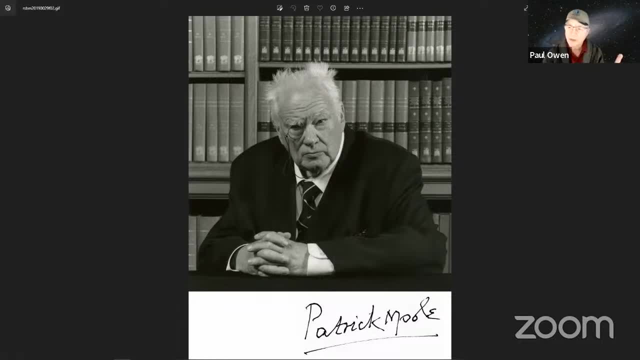 read this article that Sir Patrick Moore did some of his military training in Moncton, New Brunswick and that looked kind of it's like wow, I can't believe that he was actually in Moncton, New Brunswick training and when he was just a little fellow young guy when he, when he 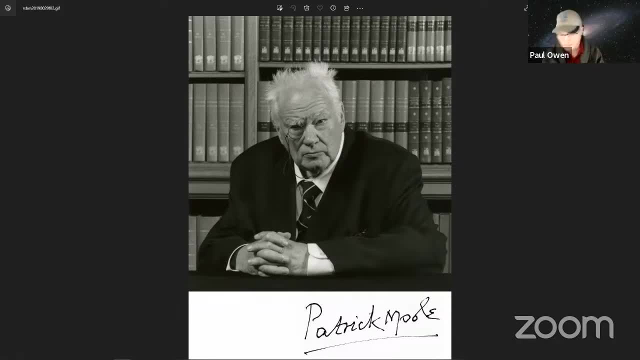 joined his services. he tried a whole bunch of stuff, but he didn't have the health to do certain thing. you want to be a pilot, so they had him go into navigation instead, and he did a whole bunch of different stuff in his younger years. so let me just see now. okay, let's get into the professional 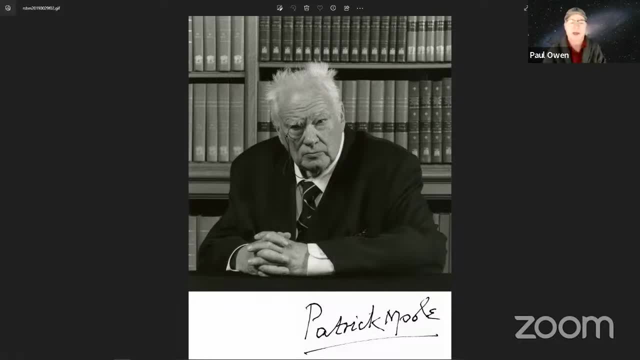 amateur astronomer. So after his father's death in 1948, he taught history and French at Holmwood House Preparatory School near Tunbridge Wells, when he was remembered as an enthusiastic teacher. but he left teaching in 1952. from the time onwards he made a living as a freelance copy editor, author and broadcaster. 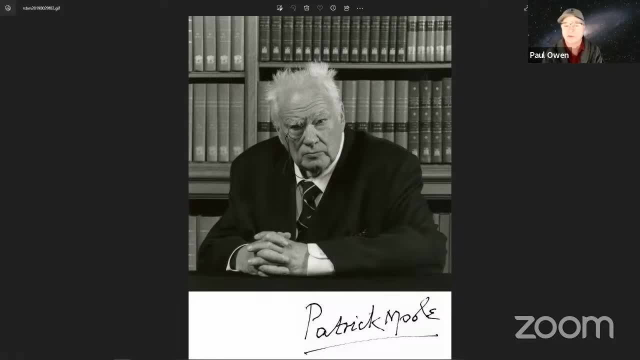 through briefly, though briefly. serving as the first director of the ARMA planetarium. living in the elegant Georgian house nearby with his mother, he oversaw and the planning and construction of the planetarium, which took three years and it was- I think it was- finished in 68 but left that the day. 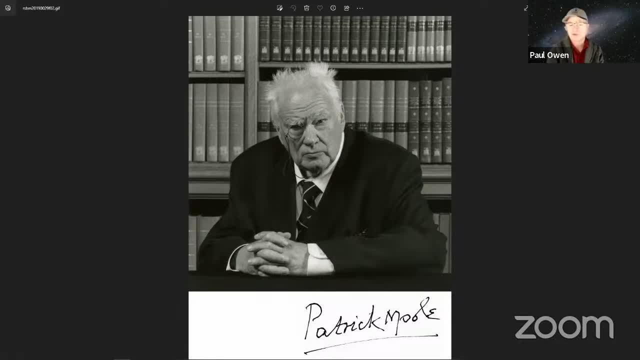 it was open to the public. the reasons for the abrupt departure aren't altogether clear, but they were cited that there were some religious things that were going on. so anyway, so he left for that reason. so Moore started that. he- or Moore stated rather, that he had written over 100 books. 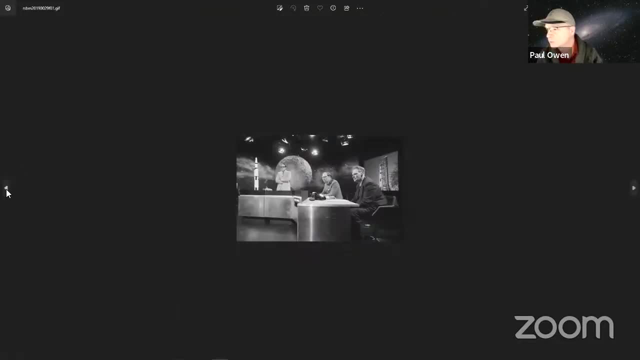 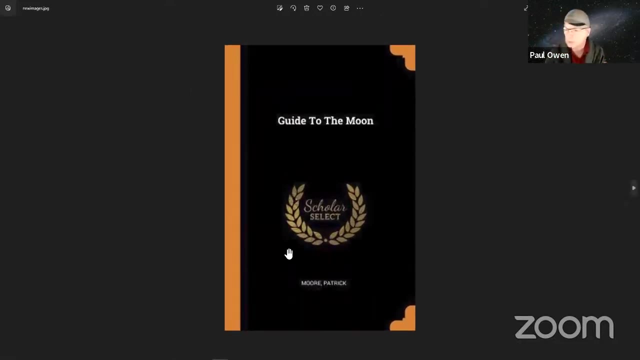 and while we've got his picture up- I don't know if I can sift through some- I'm going to show you some of them. this is just a couple and these ones he actually was quite well known for the guide of the moon Patrick Moore was. you could call him a professional moon chart fellow and a lot of people used his work. 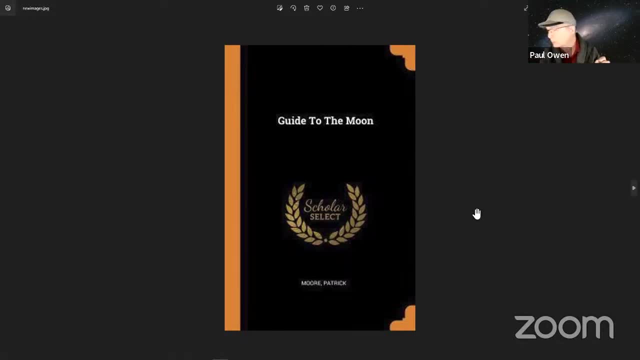 to study the moon. he anyway, that's one of his books. the other one that I will highlight is Patrick Moore's book The Guide to the Moon. The other one that I will highlight is Patrick Moore's book The Guide to the Moon. The Guide to the Moon. 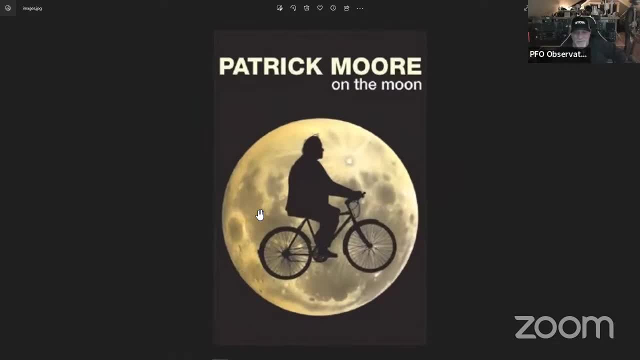 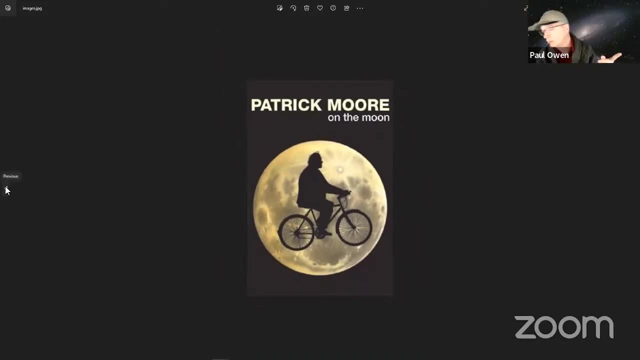 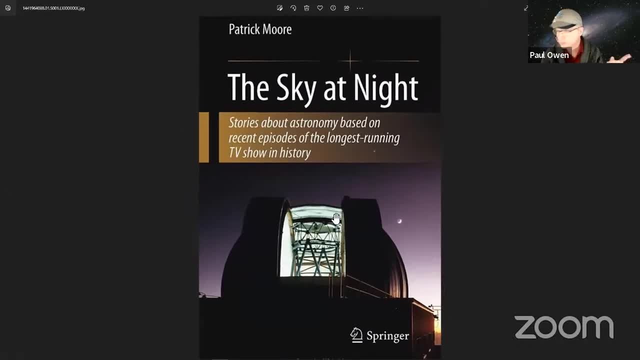 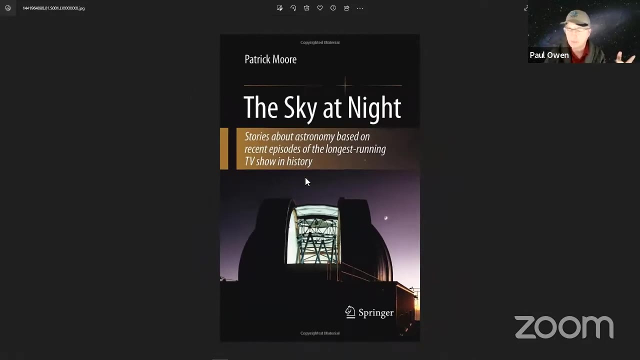 The Sky at Night, which is actually the stories about astronomy based on recent episodes of the longest running tv show in history. so that's actually a really, really interesting read. and the magazine that you guys may see called uh um, the sky at night. uh king comes from over there too, oh, and this one here is probably his. 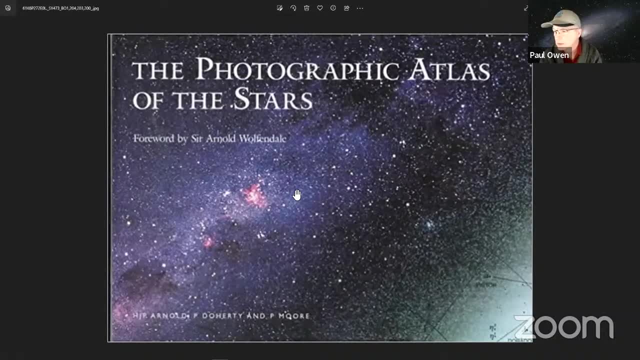 most famous, the photographic atlas of the stars, and uh. a lot of these books have been redone many times but never rewritten the way that he wrote them, because he was so articulate as a writer. they never had to be rewritten, only if it was a long, long, long long time ahead and they were 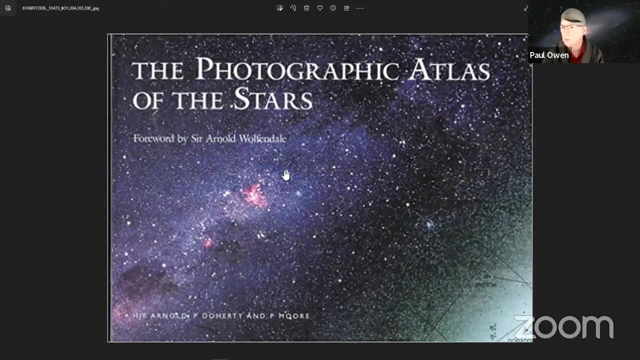 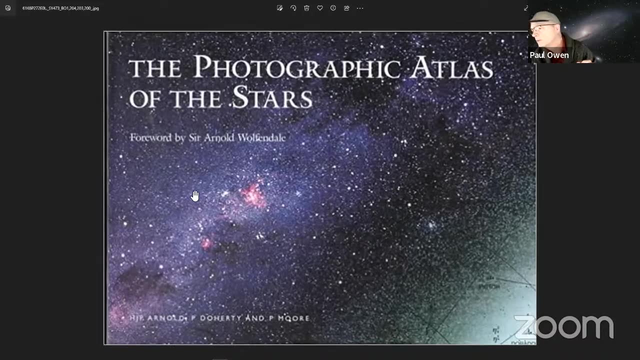 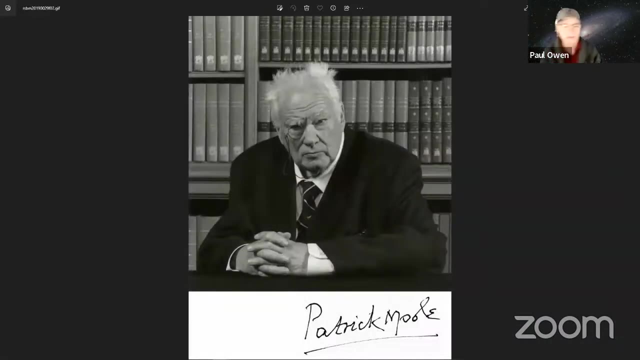 going to do a rewrite and there was something a little bit more interesting that had to go in. and they're not. nothing was ever changed or corrected. i'll go back to his photograph is hang on here now. oops, where's the sign? oh, there he is. okay, let's go back to patrick. okay. 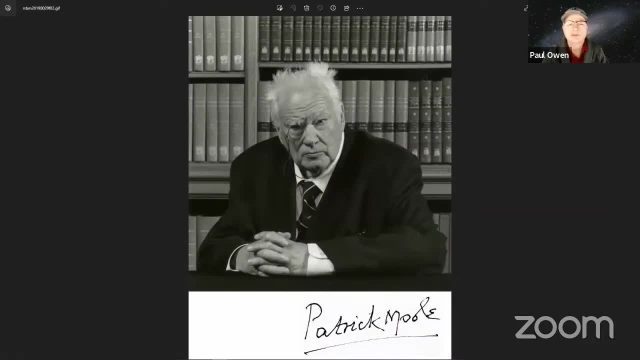 so, um, uh, okay, yeah, so this this entirely plausible. this is entirely plausible, the 100 books that he claimed uh, from the list of titles given in the in the uh bibliography uh, and recalling that From 1962, he edited the Yearbook of Astronomy, published annually. 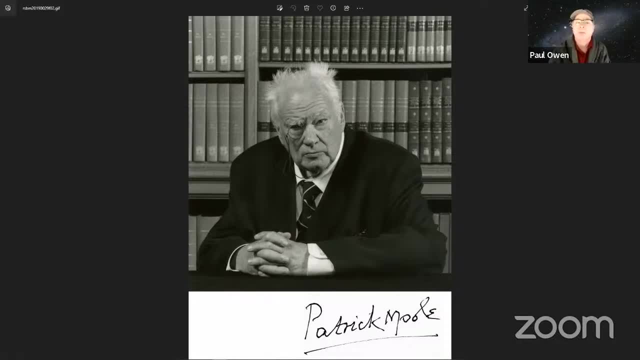 Indeed, his biography, Martin, his biographer- sorry, Martin Mauldy- counted 300 books, included revised editions and a yearbook. He scored an early. he scored an early success in 1953 with A Guide to the Moon, which was followed by A Guide to the Planets, A Guide to the Stars. 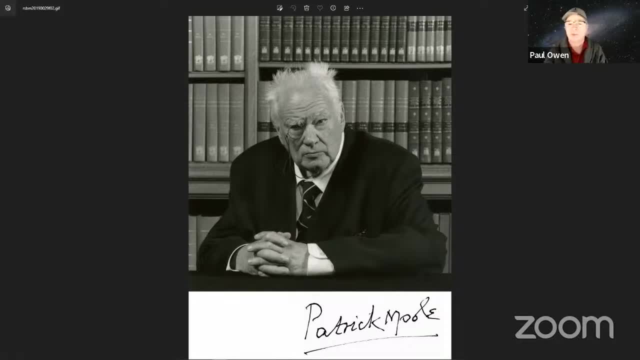 Other representative titles included The Picture History of Astronomy, Astronomy Quiz Book, Armchair Astronomy, Explorers of Science- I'm just naming these because these are the relevant ones- and The Guinness Book of Astronomy. And his most commercially successful book was The Atlas of the Universe, which went through several editions and was translated into many languages. 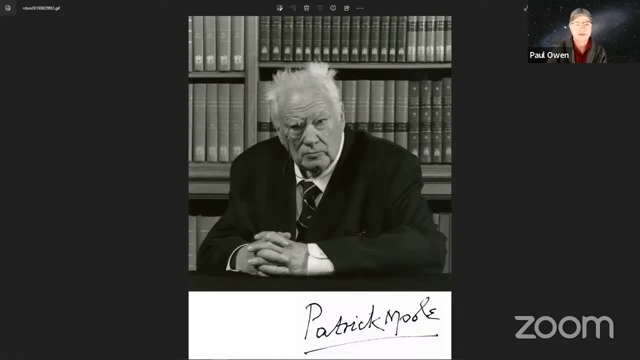 But the prolifogy of book production, in addition to numerous newspapers and magazine articles, can be attributed to his extreme fluency in the use of the English language, and he told one of us from MSL that he never revised any of his writings. So that's I mean without those books. that's unbelievable. So most of his books were aimed at children and the general reader, but he developed a particular expertise of the moon and collaborated with amateur astronomer Hugh Percy Wilkins on refining the ladder's map. 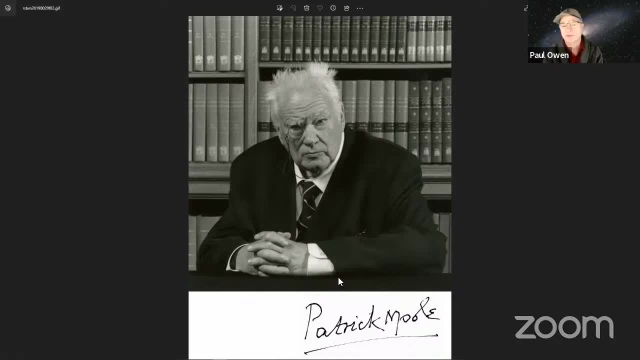 of the Lunar surface for re-publication in 1955.. In the moon, a complete description of the surface of the moon. the 300-inch diameter map was used by NASA to shortlist possible Apollo landing sites And in 1995, he published a Caldwell catalog, thus the name Caldwell. 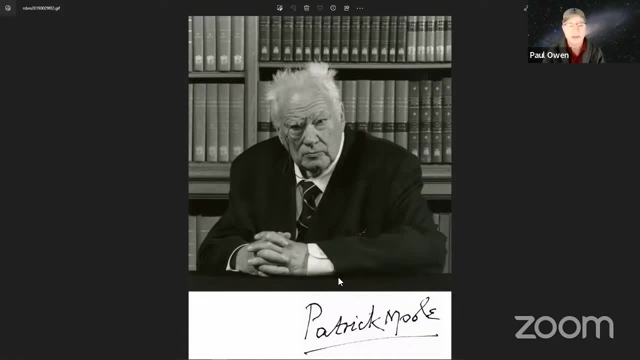 That's where the name came from. in the magazine Sky and Telescope, A list of 109 of the world's largestbut usedkt um ratio of creation data was found in in 1995.. The bok the British Abbey handbook for the New Year livro wasived into covered ibyp bereit primero. 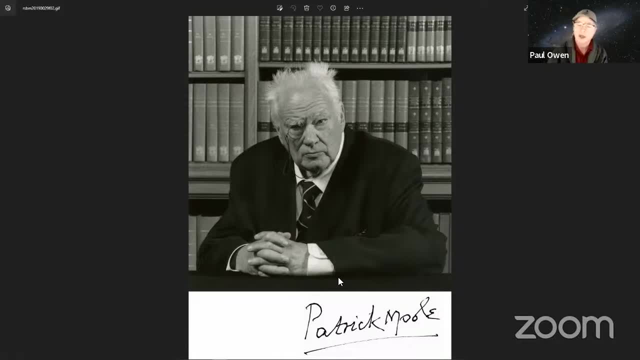 That's the Nupillera Prado, And this summer there was an inter polsk catalog en el tempo to enjoy the bullet quiz, published unceremonious chronology as a 112Miss Colmcuy Aramco title telescope a list of 109 of the brightest deep sky objects, such as star clusters, nebula. 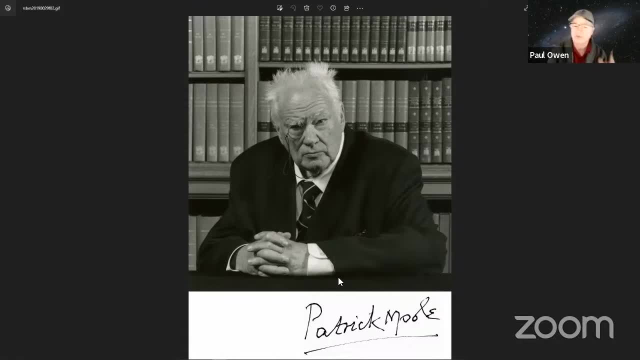 and galaxies which had been left out of the famous Messier catalog, compiled by, of course, Charles Messier in 1771. So the Caldwell list of catalog came from this gentleman unbelievable. He also wrote several science fiction stories for children, including five novels set on. 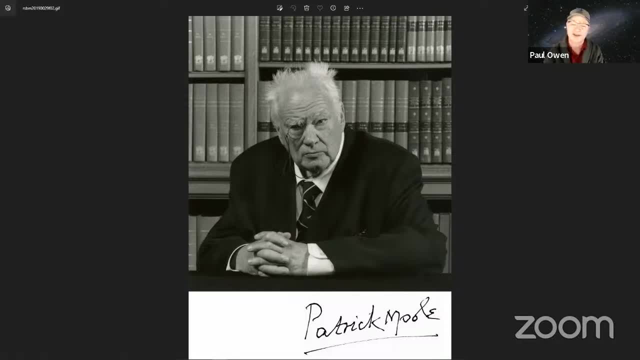 Mars featuring an orphaned 16 year old, Morris Gray, and another six featuring the young astronaut Scott Saunders, And he published two humorous works under the name RT Fishall- How to Annoy Them and the Twitmarsh File. The former contained the suggestions, such as demanding replies to letters that had not 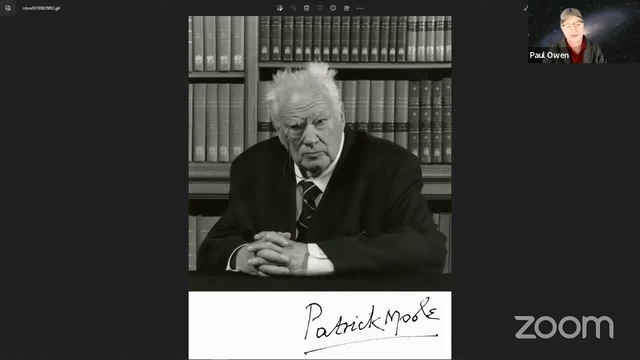 been sent on rubbing candle wax on areas of forms of which said do not write here. He was a great lover of pranks and spoofs. Okay, so let's get into his broadcasting career. So Moore's first television appearance was in December 1956, in a program on unidentified 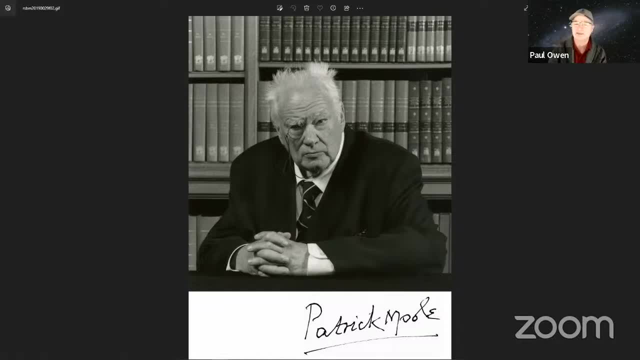 flying objects as part of BBC's firsthand series in which he represented the skeptically skeptical position. So obviously he was the guys that we are today about certain things. Anyway, So, despite the very late- Oh sorry- And it was launched in on April 24 1957, as an extremely low budget, around the midnight. 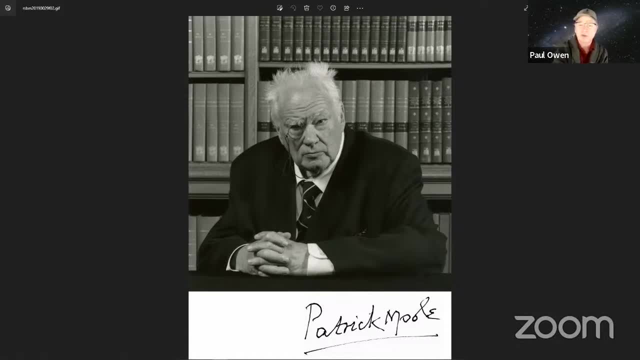 monthly half hour program. So despite the very late billing, it was an enormous success. the opening cyberless music being immutably imprinted on many of our minds, you'd have to listen to the show, to listen to the start, to get what he's talking about there. 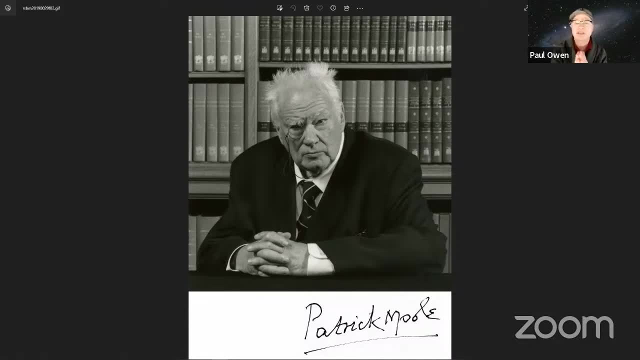 For many years. it was filmed live. Okay, So he was a very conceivable topic in astronomy, as well as what was happening in the sky At the time. each program was broadcast. He always made it completely clear, however, he was an amateur astronomer with no pretensions. 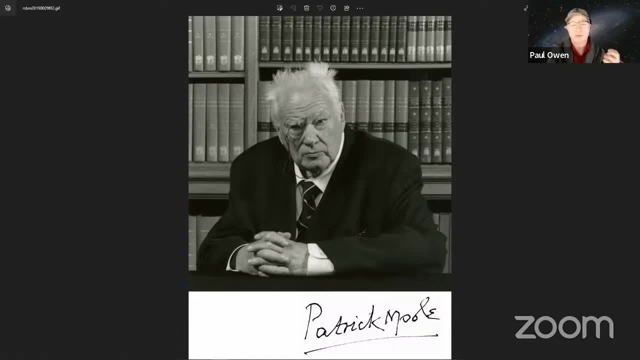 to professional expertise. He had the inviolable ability of drawing the best out of his professional colleagues and making the topics perfectly accessible to the large non expert audience Sound familiar. Those of us who appeared on the program remember with affection that the amateurish but compelling 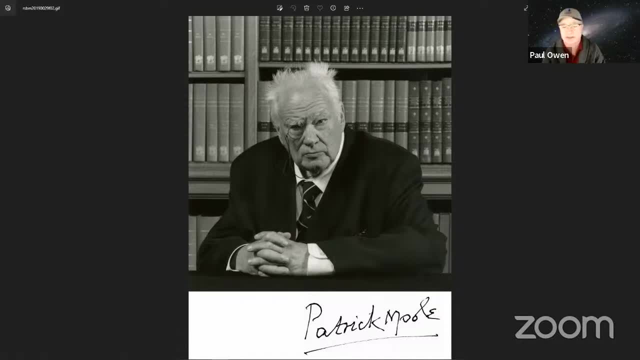 enthusiasm he brought out and even some of the trickiest aspects of astronomy. perhaps the most amazing aspect of his role as anchor of the program was his outstanding ability to speak at an extremely high speed, with complete fluency and immaculate articulation. So if you ever just watch him, just watch how fast he talks, and once you get into his groove, 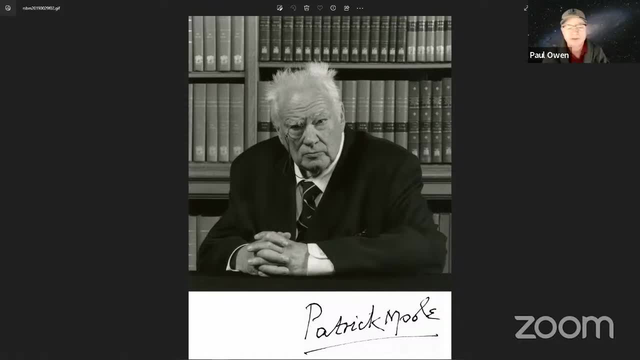 you can understand what he's saying. There was never a stumble. He told one of us that he always knew the end of the sentence when he started it. That's amazing. So Moore presented the sky at night for more than 55 years, missing only one episode through. 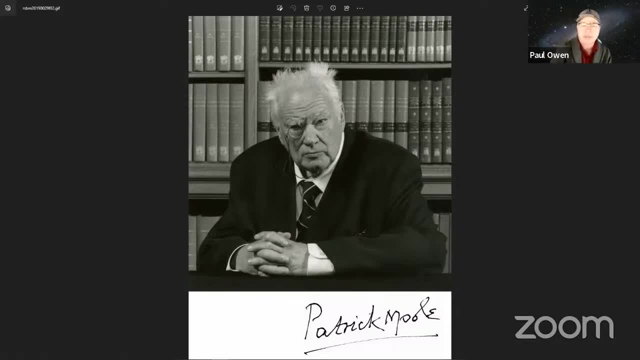 ill health in 2004.. He presented the subsequent episodes from his house. His last episode was broadcast on January 7, 2013,- a month after his death, making it the longest running program. What was it? It was a series of interviews. 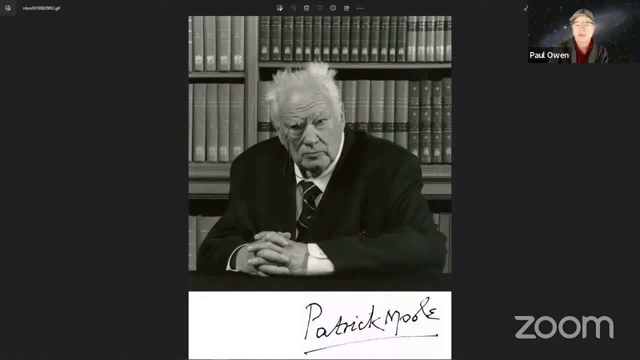 It was a series of interviews with the same presenter in television history. Moore was sometimes, but not always, joined by guests among the most of the world's leading astronomers and astronauts, but it was his ability, his ability, ability with television person sorry- and rapid fire delivery which held the program together and gave a verve. 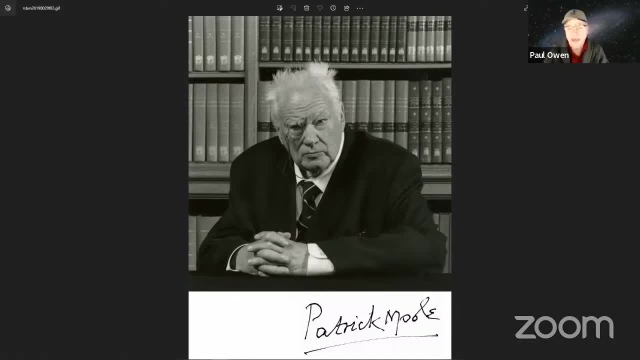 and pace. the series drew large audiences and amateurish astronomers and was credited by many younger professional and amateur astronomers, and indeed scientists more generally, with the first sparking of their interest in science. Now I'm going to show you one more picture. That's kind of cool. 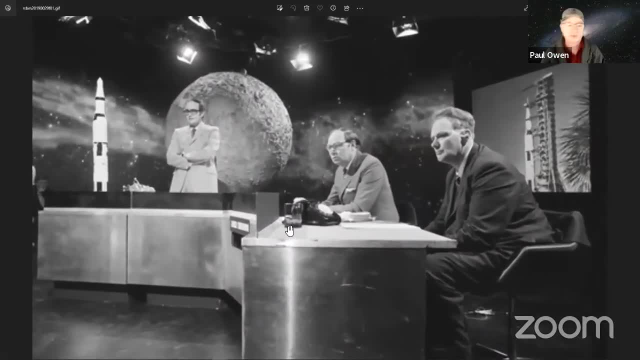 Chris, I think you can relate to this as well. This is for Patrick Moore, James Burke and Cliff Michael Moore reporting on the Apollo 11 mission to the moon. This was in 1969. And this was a BBC, So they actually covered that. 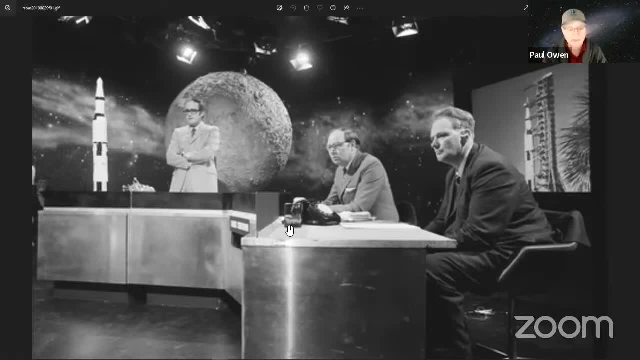 And this was the actual show, an image of the show that was broadcast when they were covering that, that particular mission. Nice, Yeah, unbelievable, So anyway. so it goes on and on, and I won't get into everything else because there's so. 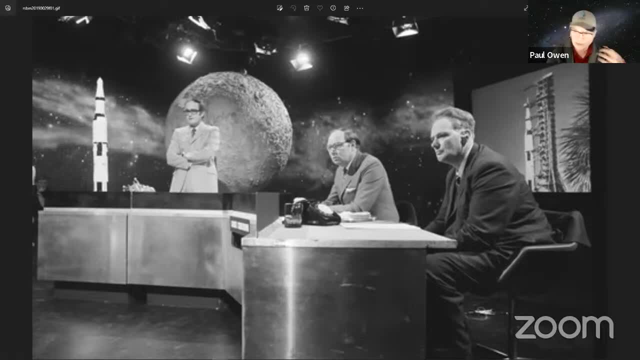 much more to talk about with this guy in terms of his telescopes and what he used and what his philosophies were and all that. But he is such, He is such a genius, He is such an important figure in astronomy from yesterday and still is today, even though 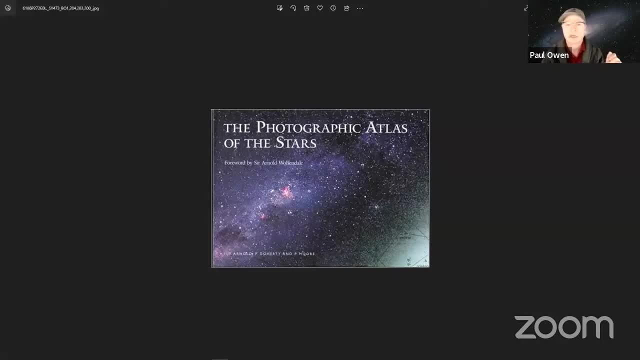 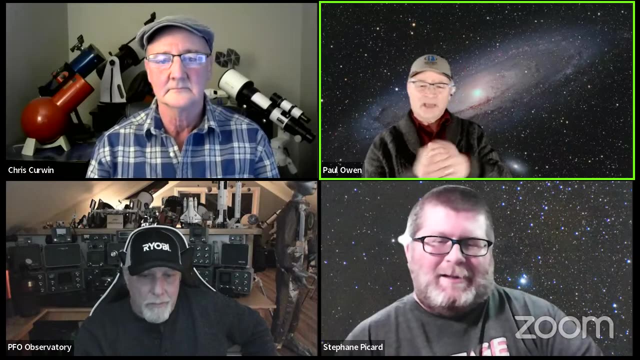 he hasn't been around in quite some time. So that's just what I want to cover. How do I get out of this thing here? Stop sharing. That's what I want to cover on Sir Patrick Moore, And that's just not even the tip of a tip of an iceberg of what he has done. 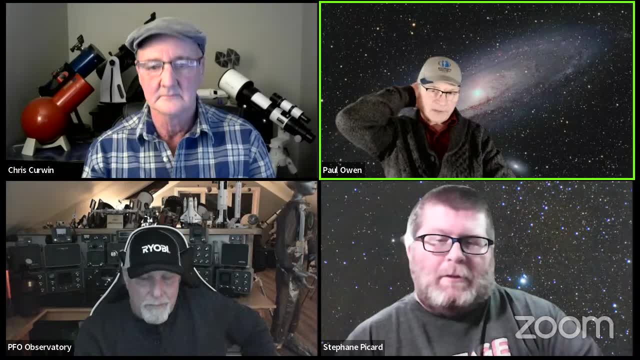 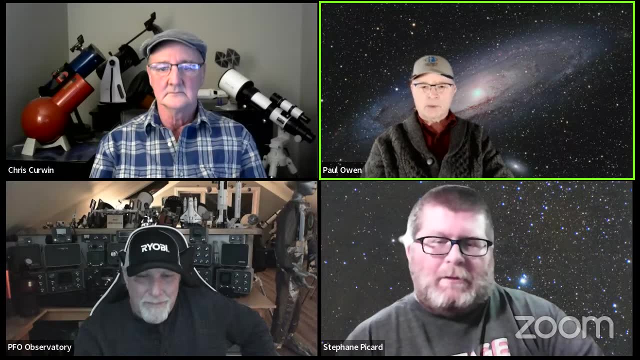 And so I think maybe later on I'll cover some more stuff that he did, because to me he is just such an Such an important figure that people should know about. if they don't know about him, he should study him, because he's, and all of his videos are still on YouTube. 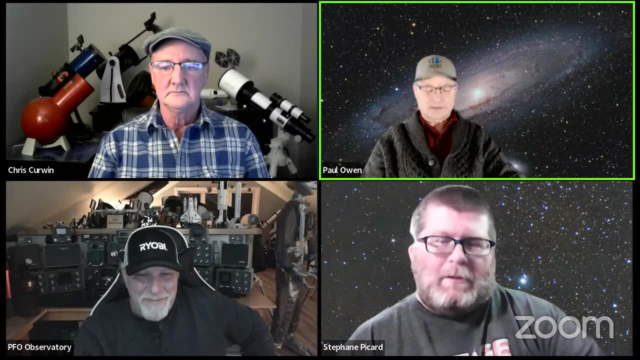 You can watch them. And if you want to watch the program, so it's. it's. anyway, he's an interesting guy. I got one question, One simple question. Yeah, What's with the British people in this hair, Boris Johnson's hair, his hair. 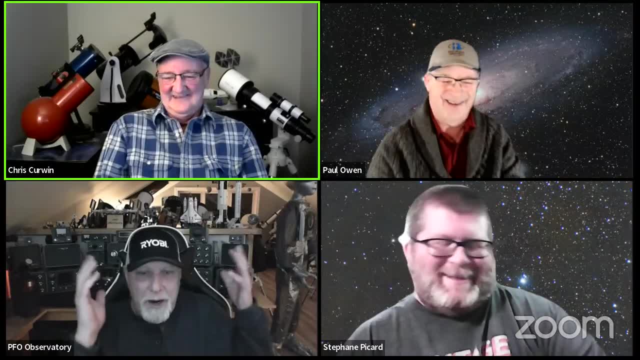 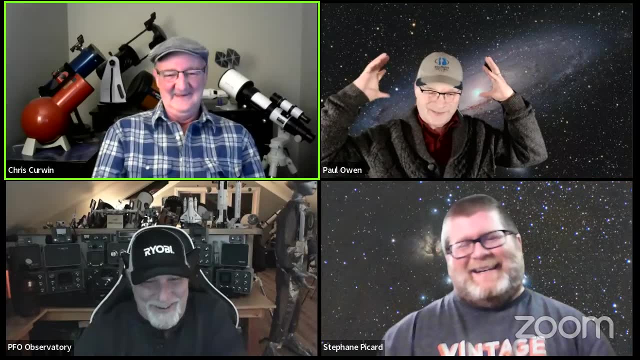 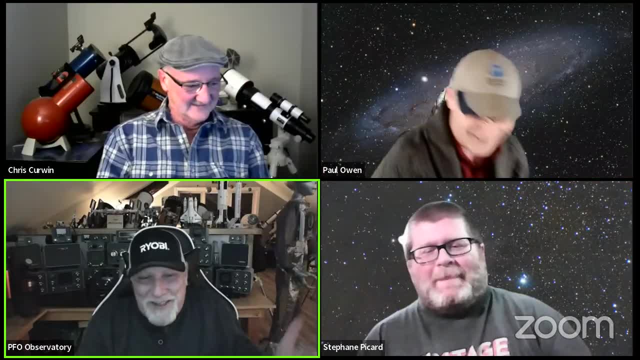 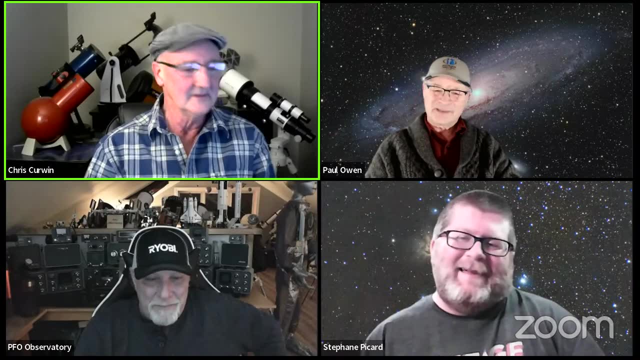 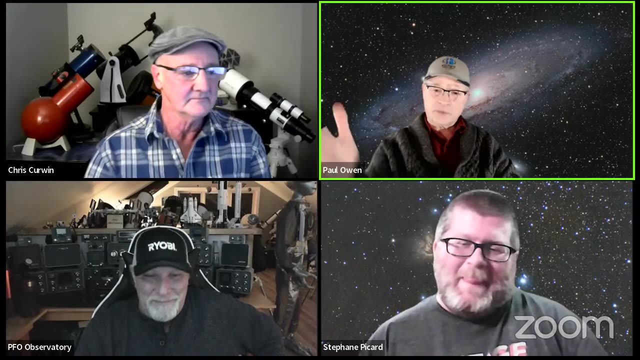 Buggy, That's a simple question. Fascinating Thanks, Paul. Fascinating man: Yeah, He would have quite the stories that prison, Oh yeah, Yeah. So when you're going through the catalogs, the Caldwell catalog, that's the other messier. 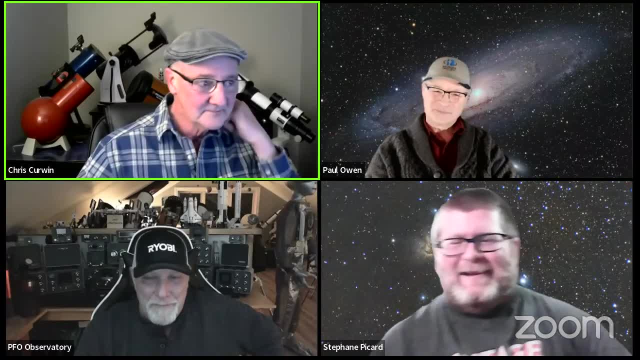 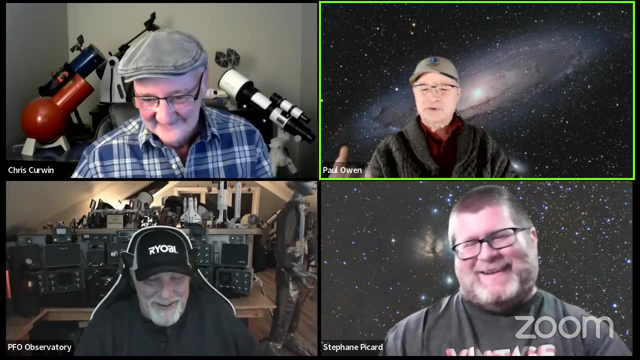 exactly The other messier, that's right. Messier part two. Messier part two. Well, there's a Caldwell 40. it's even interesting to know where that name came from. yeah, really, his grandfather's middle name. yeah, there you go. 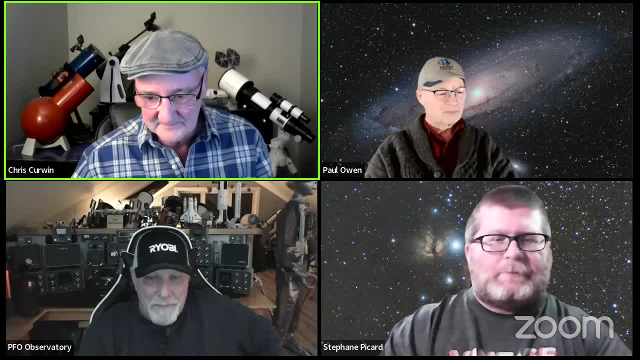 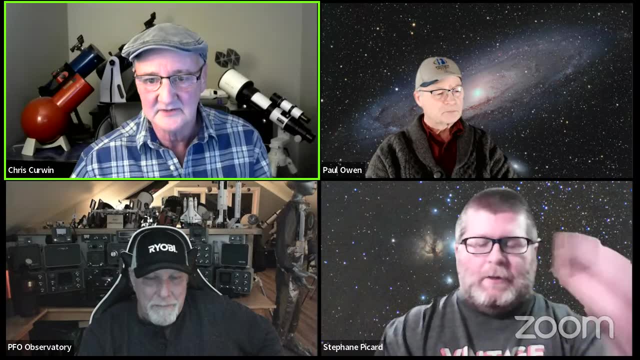 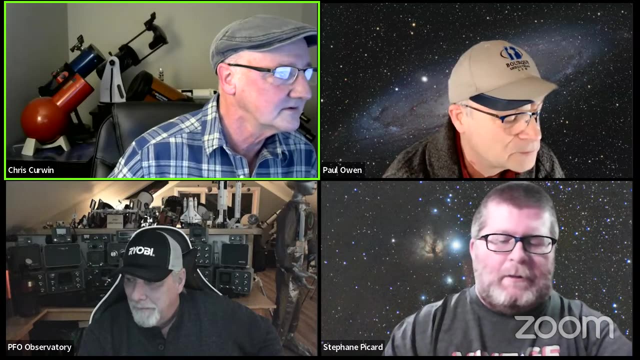 awesome, thank you, yeah, okay, um, i'm gonna try my talk, i guess, um, and get the right screen to share. first of all, let me get it up on the screen here first of all. i don't know whether i'm going to have sound. oh yeah, lisa. uh mentioned a magazine or a book. 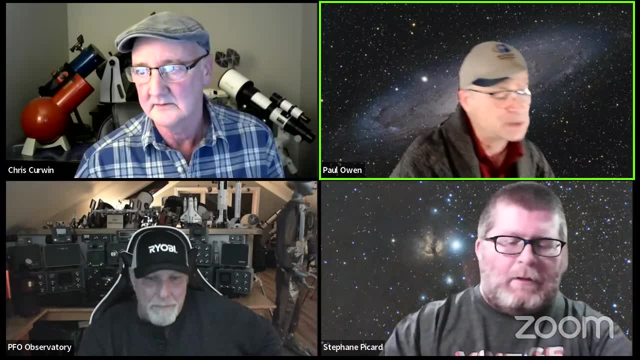 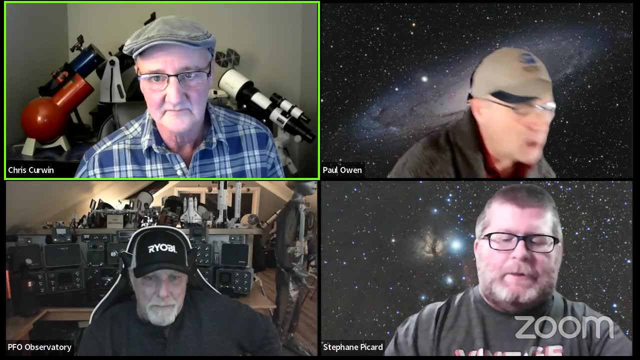 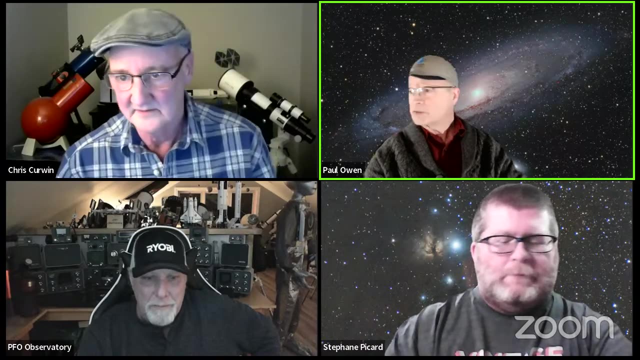 it was called uh bang and it was the complete history of the universe, and brian may was actually in on that one with uh right, yeah, who else opa? author: chris chris linton. chris linton lintot, i guess you have to pronounce it. i'll have to get check that one out, because i 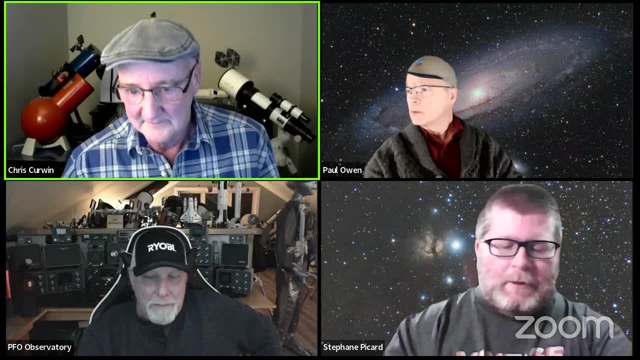 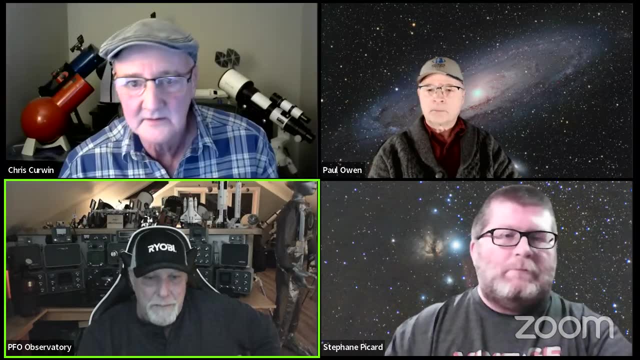 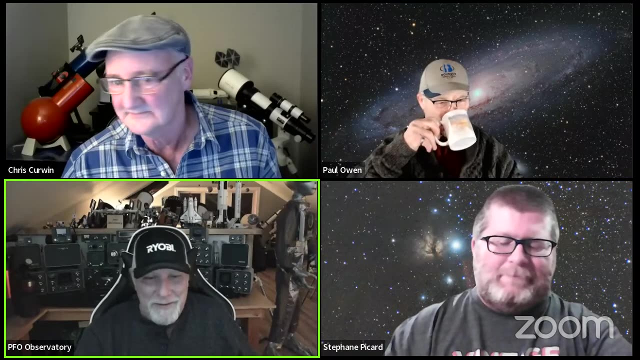 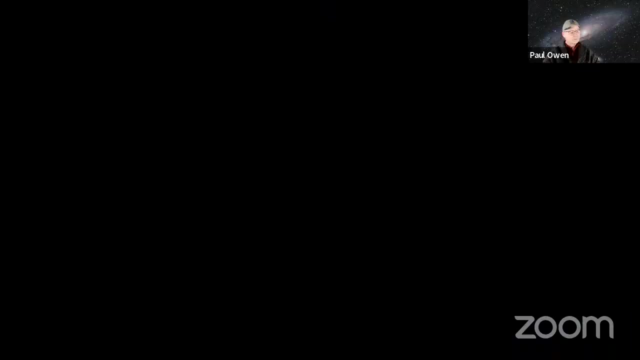 haven't seen it okay. um, i guess what am i out here on screen number one, next slide? yeah, i have to keep forgetting my guitar. i gotta bring it out. yeah, i guess i'm in between music going great screen here in a second. i think it might be part of it. there he is, do you want? uh? 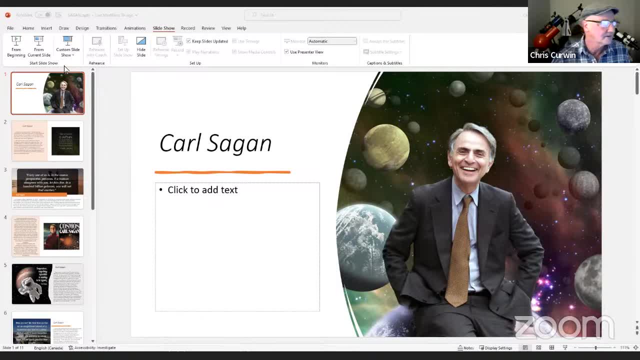 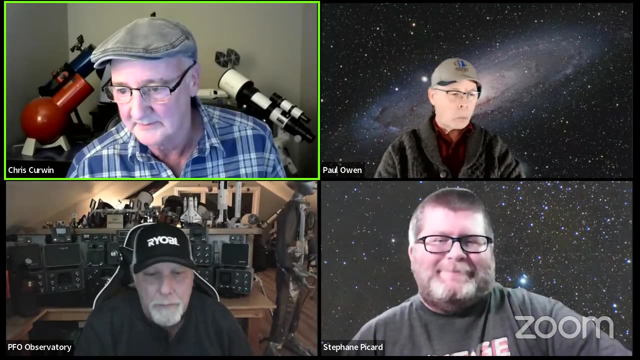 that one. i want it. though, hang on, i'm sure i'm beginning get them up on the other screen, so just a second. stop sharing the right screen. this would be okay. now i get them up there. okay, yeah, for me, for me, it's got to be this guy. 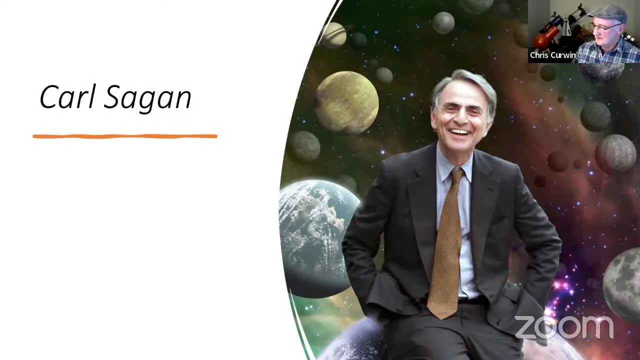 um, i guess because i became such a fan of astronomy when, uh, the cosmos series um that he that he produced um with andrewian his wife became his wife, i guess, later, um, and i was hooked on that series uh very early in in my astronomy. uh, love, i guess of astronomy. so i'm gonna just one more second here. 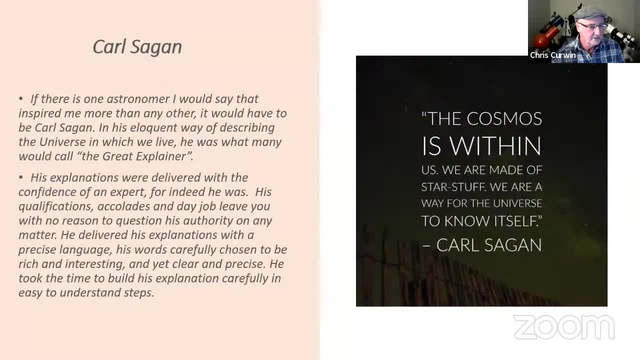 i'm gonna bring up my third screen. here we are. okay, we'll talk a little bit about carl sagan. uh, on the right hand side you're gonna see a little bit of the quotes that i've copied from uh, some of his best quotes that he gave, anyway. um, now, if there was one astronomer, i would say: 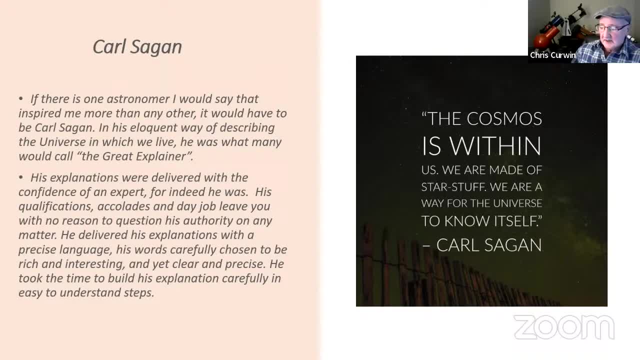 that inspired me more than any other astronomer. i would say that inspired me more than any other would have to be carl sagan. uh, in his eloquent way of describing the universe in which we live, he was what many would call the the quote great explainer. uh, his explanations were delivered. 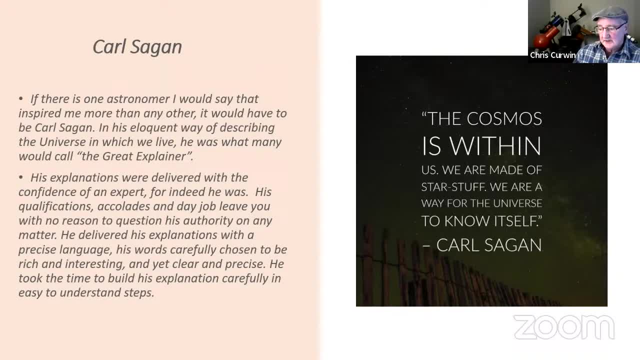 with confidence of an expert, for indeed he really was. uh, his qualifications, accolades and and day job leave you with no reason to question any of his authority on any matter. he delivered the explanations with precise language, his words carefully chosen to be rich and interesting, and yet clear and precise. 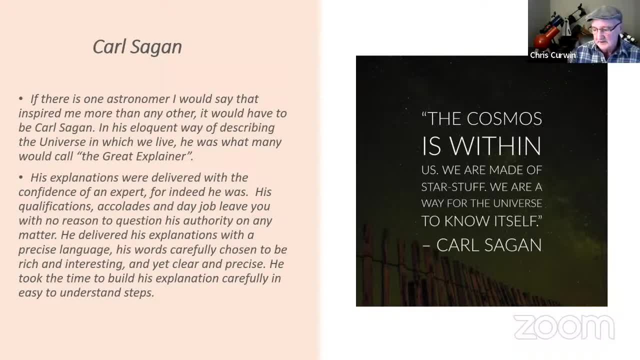 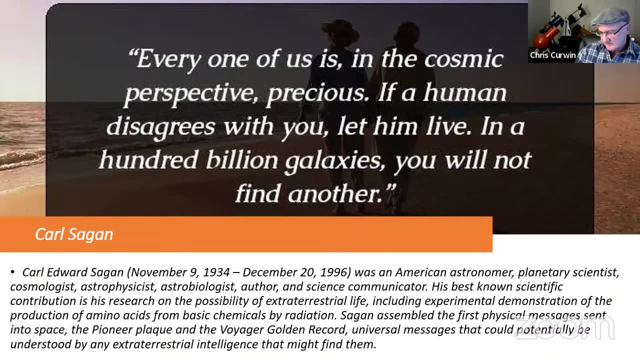 he took the time to build his explanation carefully and easy to understand. steps now, carl sagan uh, from 1934, november 9th 1934 to december the 20th 1996, was an american astronomer. american now listen all this american astronomer, planetary scientist, cosmologist, astrophysicist. 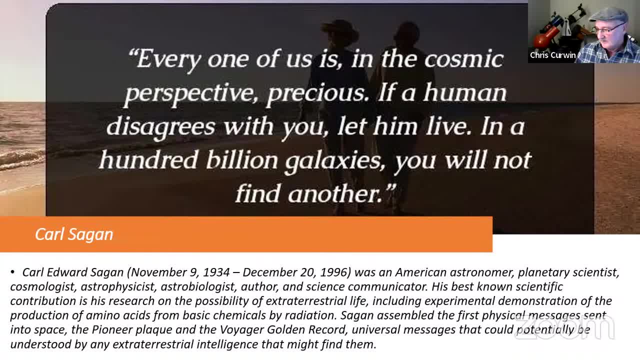 astrobiologist, author and a science communicator- what a resume. his best known scientific contribution is his research in on the possibility of extraterrestrial life, including experimental demonstration of the production of amino acids from basic chemicals by radiation. a sagan assembled the first physical messages sent into space: the pioneer plaque in the voyager. 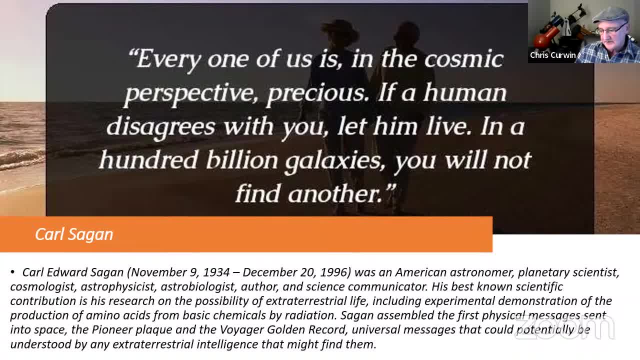 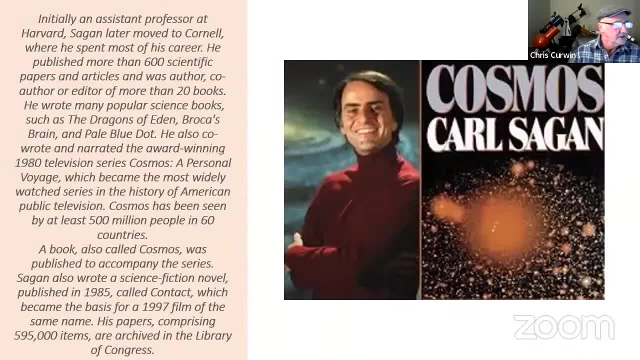 golden record: universal messages that could potentially be understood by any extraterrestrial intelligence that might find them. initially, an assistant professor at harvard, sagan, mentioned that he had been working on a research project on the possibility of extraterrestrial intelligence that could potentially be understood by any extraterrestrial intelligence. a sagan 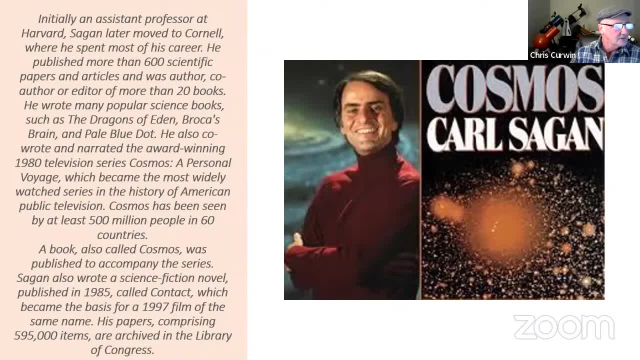 later moved to cornell, where he spent most of his career. he published more than 600 scientific papers and articles and was author, co-author and or editor of more than 20 books. he wrote many popular science books, such as the dragons of eden, rock his brain and the pale blue dot. he also co-wrote. 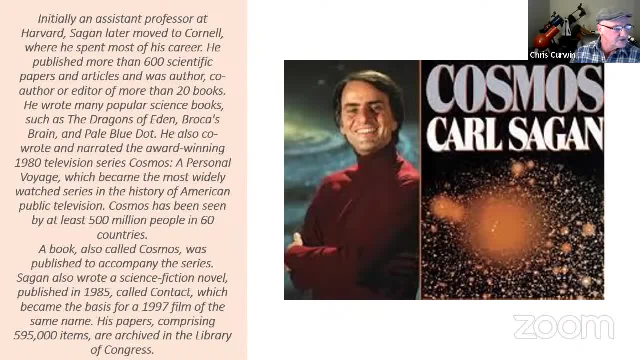 and narrated the award-winning 1980 television series cosmos, a personal voyage, which became the most widely watched series in the history of american public television. i've watched it probably a hundred times myself. uh, cosmos has been seen by at least 500 million people in 60 countries now. a book also called 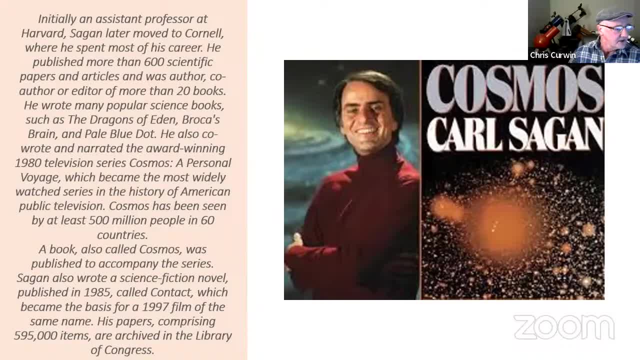 called cosmos was published. to accompany the series, sagan also wrote a science fiction novel published in 1985 called contact, which became the basis for a 1997 film of the same name. now his papers, comprising 595 000 items, are archived in the library of congress. 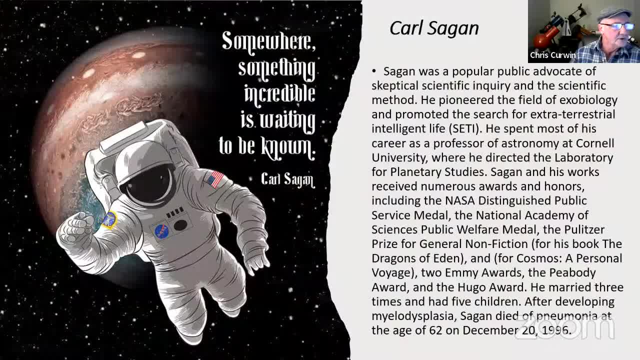 sagan was a popular advocate of the skeptical scientific and scientific research and the scientific research and the scientific research and the scientific theory and the scientific method. he pioneered the field of exobiology and promoted the search for extraterrestrial intelligence, life or a city. he spent most of his career as a professor. 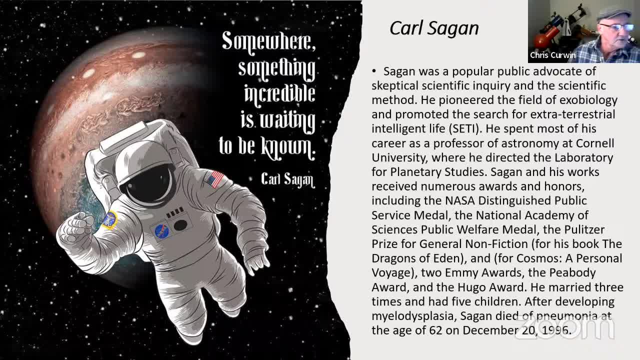 a professor of astronomy at cornell university, where he directed the laboratory for planetary science studies, sagan, and his works received numerous awards and honors, including the nasa distinguished public service medal, the national academy of sciences public welfare medal, the pulitzer prize for general non-scientific research and scientific research and the scientific research. 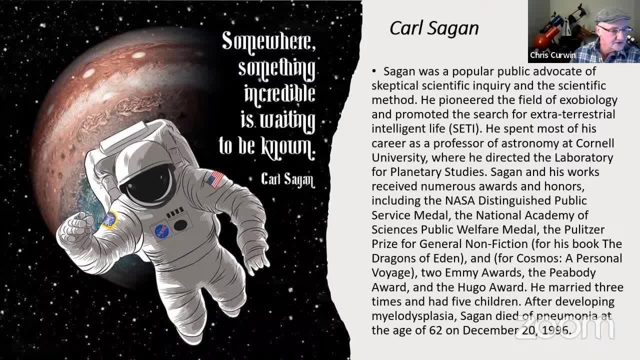 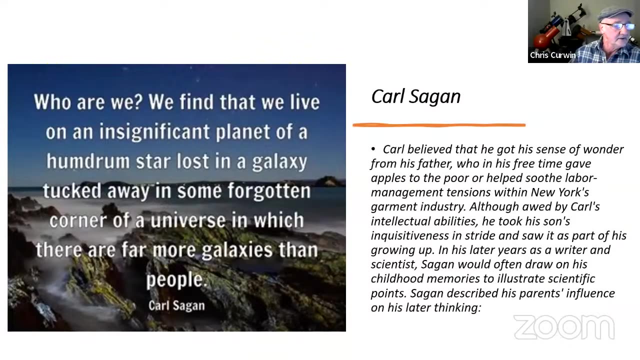 group without the sagan marketing. Space Science et al published millions of quadruple evolves in an epic to work among fellow scientists, both for the red circle and for the www. cm ты re you come c? t or helped soothe labor management tensions within New York's garment industry. 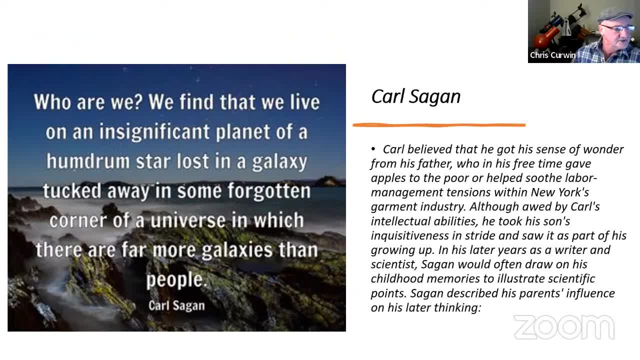 Although awed by Carl's intellectual abilities, he took his son's inquisitiveness in stride and saw it as a part of his growing up. In his later years as a writer and scientist, Sagan would often draw on his childhood memories to illustrate scientific points. 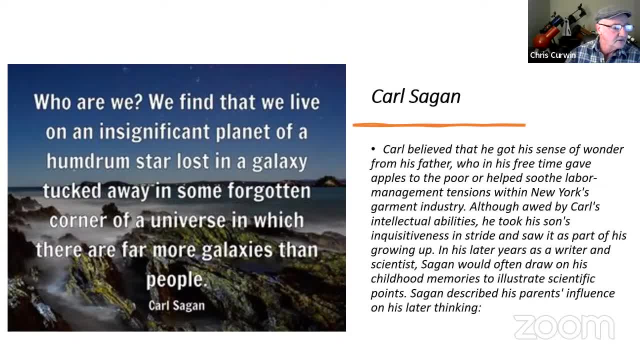 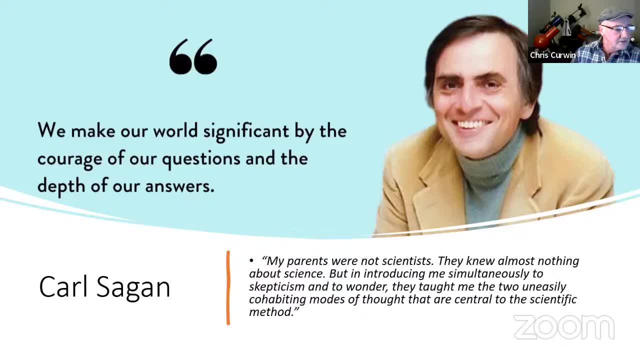 Now Sagan described his parents' influences on his later thinking Quote: my parents were not scientists, They knew almost nothing about science, But in introducing me simultaneously to skepticism and to wonder, they taught me the two uneasily cohabiting modes of thought that are central. 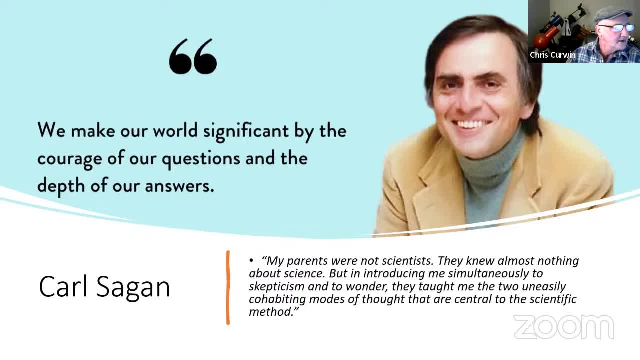 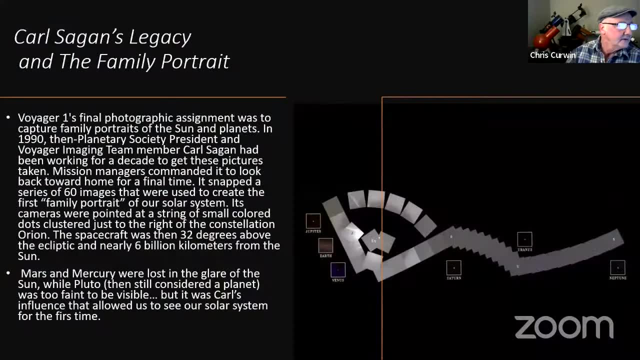 to the scientific method. I like his quotes. We make our world significant by the courage of our questions and the depth of our answers. Carl Sagan's legacy- part of his legacy- in the family portrait. We'll talk a little bit about this one. 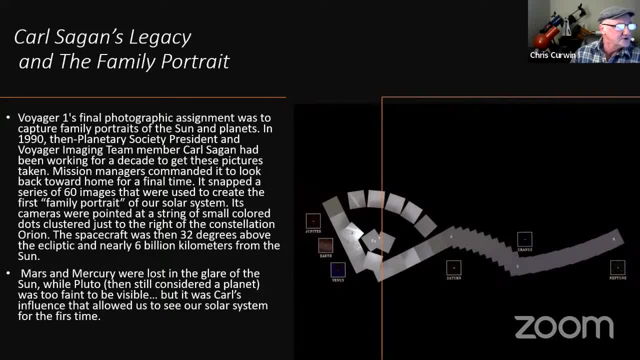 The Voyager 1's final photographic assignment was to capture family portraits of the sun and planets In 1990, then Planetary Society president and Voyager imaging team member, Carl Sagan, had been working for a decade to get these pictures taken. 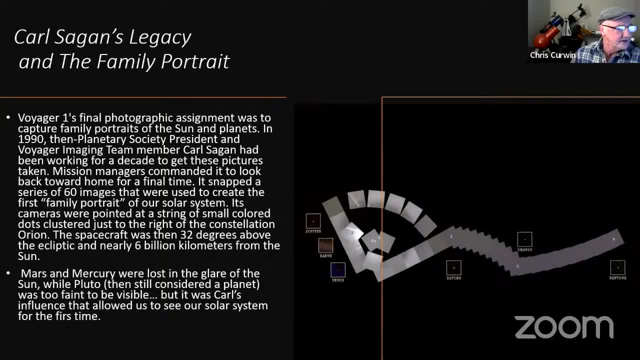 Mission managers commanded it to look back toward home for a final time. It snapped a series of 60 images that were used to create the first quote, family portrait of our solar system. Its cameras were pointed at a string of small colored dots clustered just to the right of the constellation of Orion. 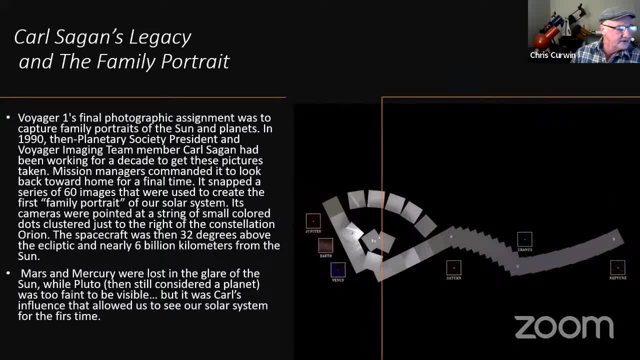 The spacecraft was then 32 degrees above the ecliptic and nearly 6 billion kilometers from home. Mars and Mercury were lost in the glare of the sun, while Pluto, then still considered a planet, was too faint to be visible. But it was Carl's influence that allowed us to see our solar system for the first time. 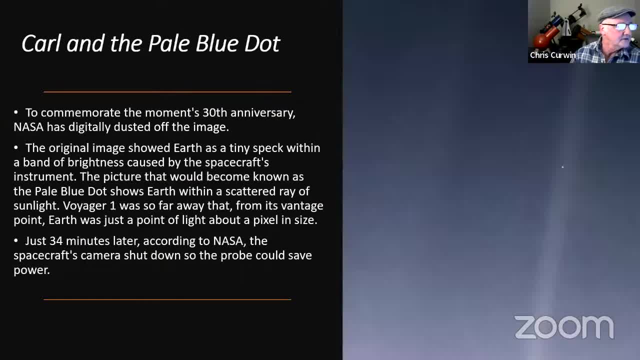 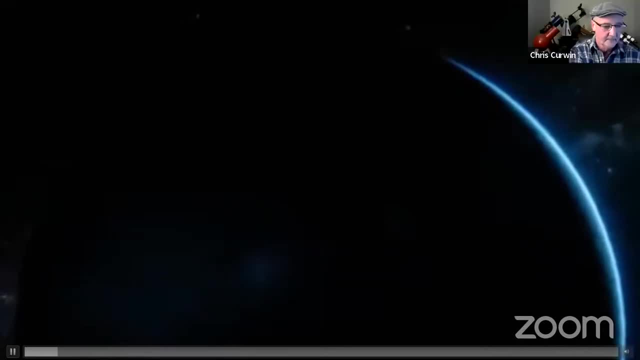 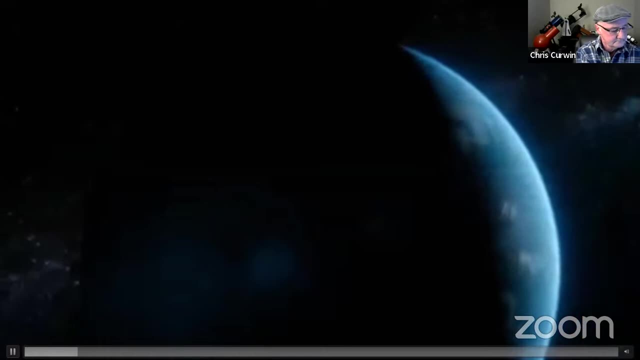 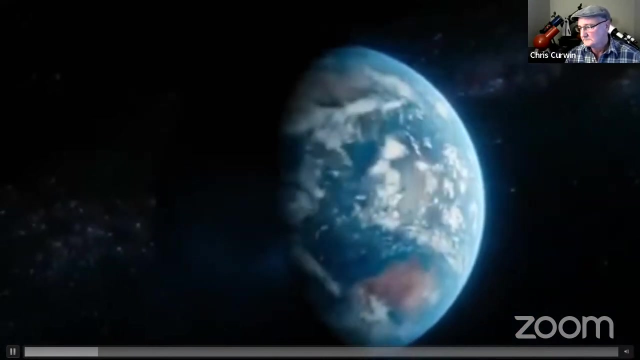 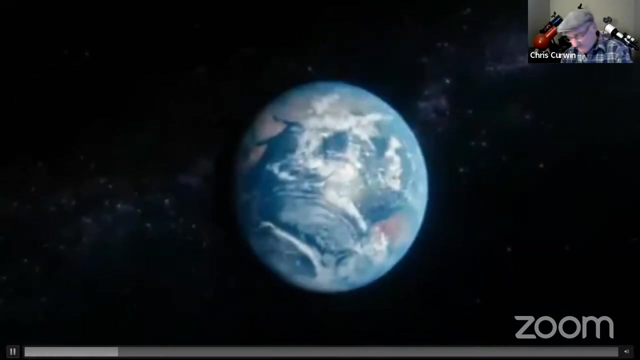 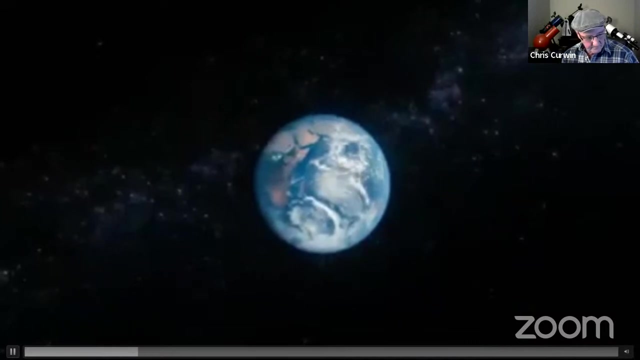 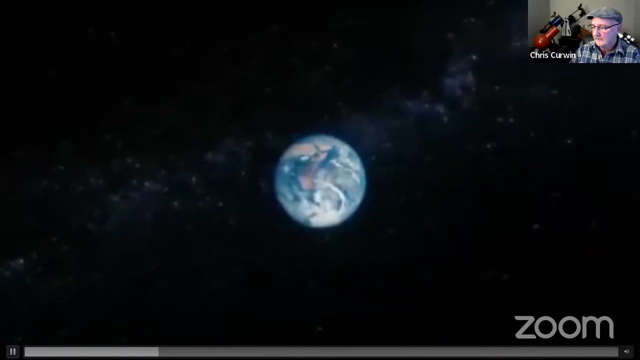 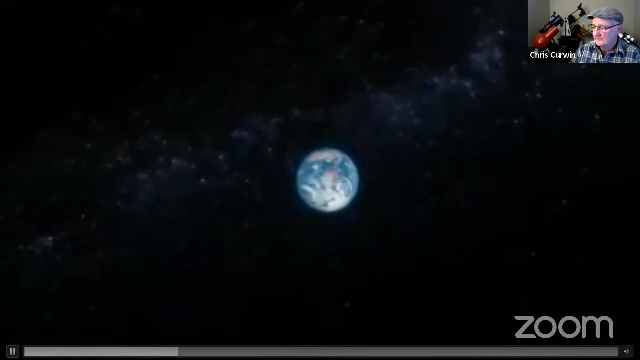 The original image showed Earth, the sun and the moon, Every king and peasant, every young couple in love, every mother and father, hopeful child, inventor and explorer, every teacher of morals, every corrupt politician, every superstar, every supreme leader. 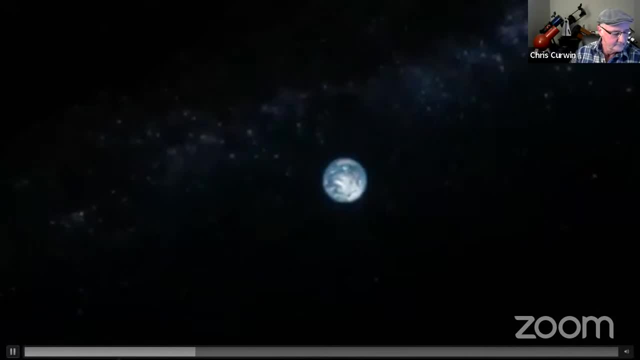 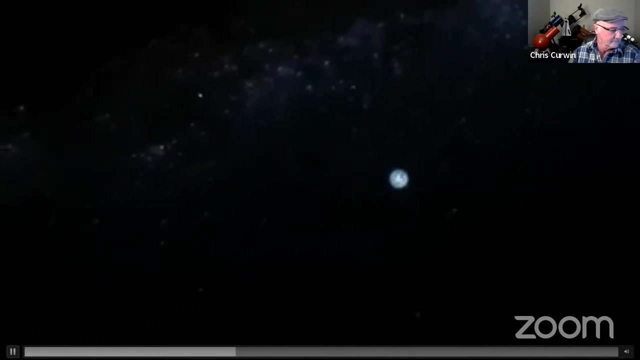 every saint and sinner in the history of our species lived there on a boat of dust suspended in a tsunami. The earth is a very small stage, yet fast For me, the rivers of blood spilled by all those generals and emperors. 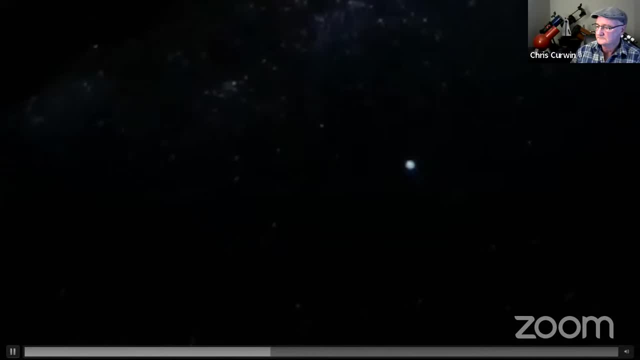 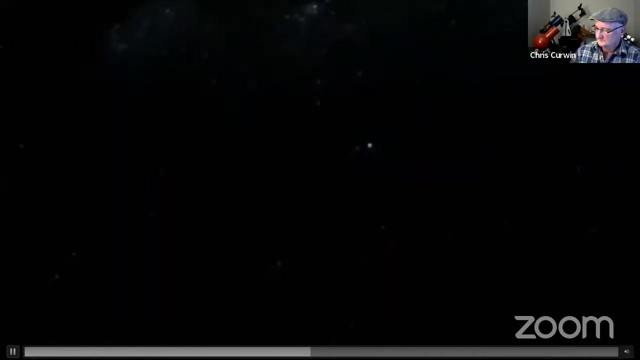 so that, in glory and triumph, they could become the momentary masters of a fraction of it. Think of the endless cruelties visited by the inhabitants of one corner of this pixel on the scarcely distinguishable inhabitants of some other corner. how frequent their misunderstandings, how eager they are to kill one another. 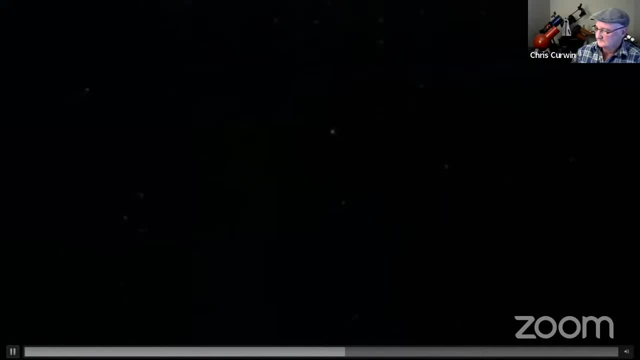 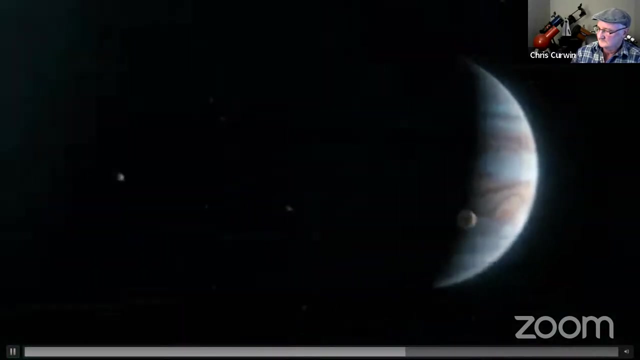 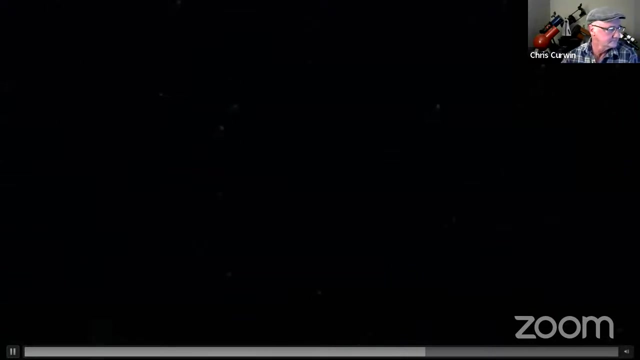 how fervent their hatreds. our posturings, our imagined self-importance, the delusion that we have some privileged position in the universe, are challenged by this. Thank you. In our obscurity, in all this vastness, there is no end. 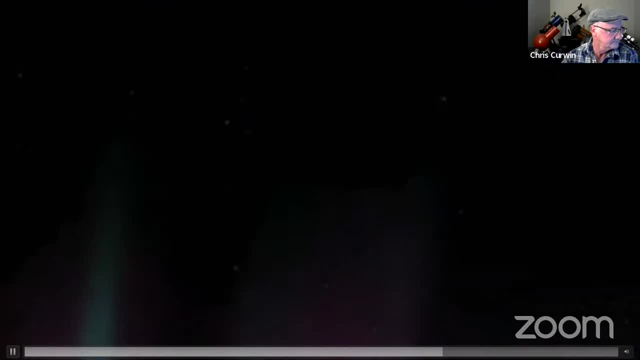 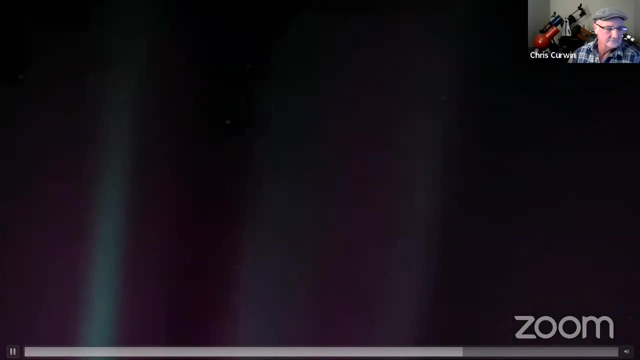 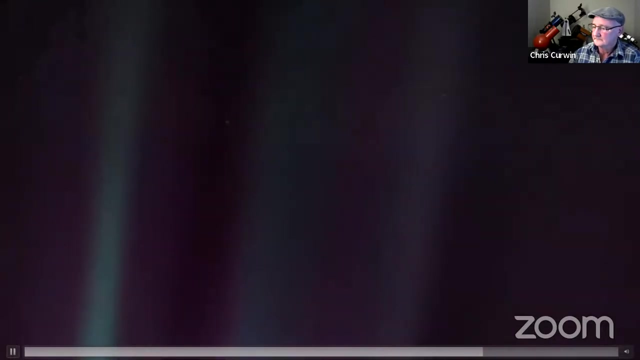 The help will come from elsewhere. The earth is the only world known so far apart from life. There is nowhere else, at least in the near future, to which our species could migrate. Did it, Yes? Settle Time? Like it or not, the moment is the officiary of the question. 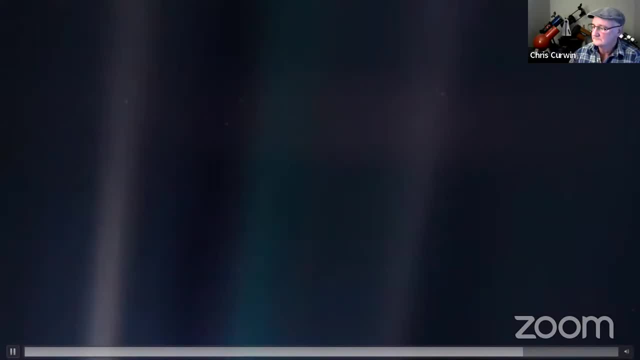 It is a humbling and character-building experience. There is perhaps no better demonstration of the folly of human conceits than this distant image. To me, it underscores our responsibility to deal more plainly with one another. The jury's choice, Thank you. 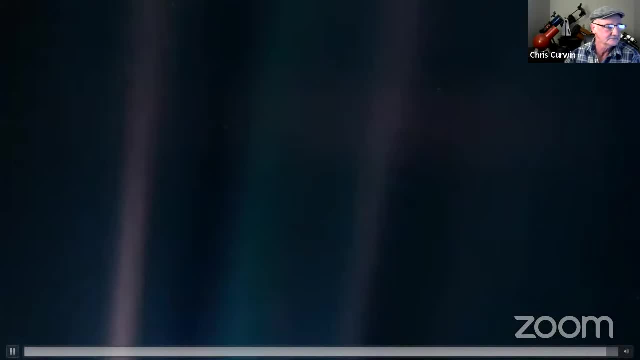 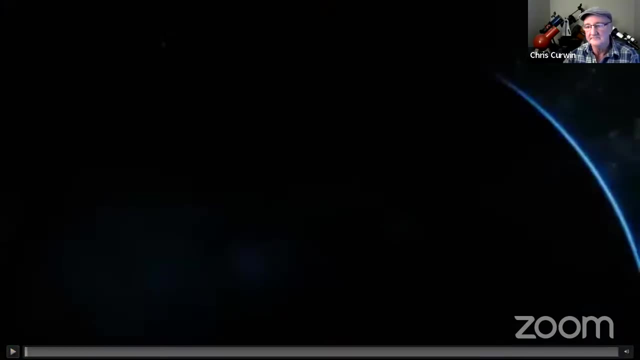 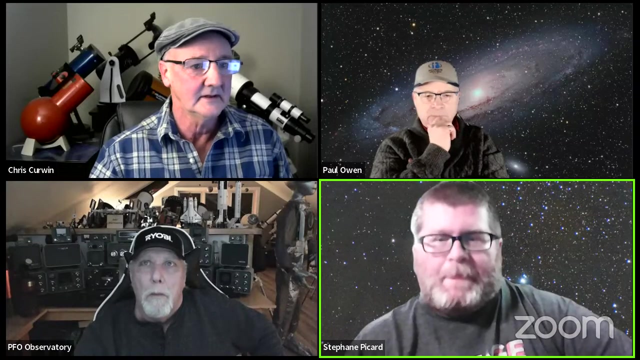 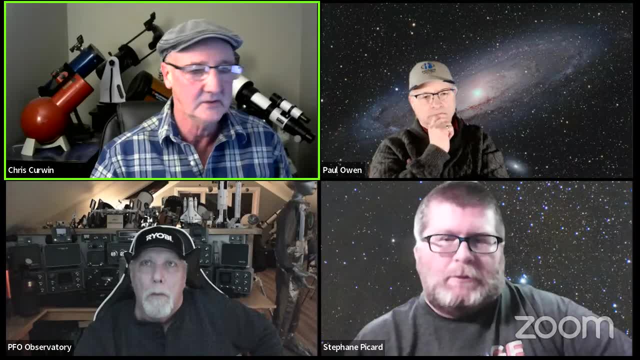 Pretty amazing, isn't it? Yeah, I think he told the story well there, And he always told the story well. He was always very eloquent in how he spoke To me. I don't think there was anybody that could match. 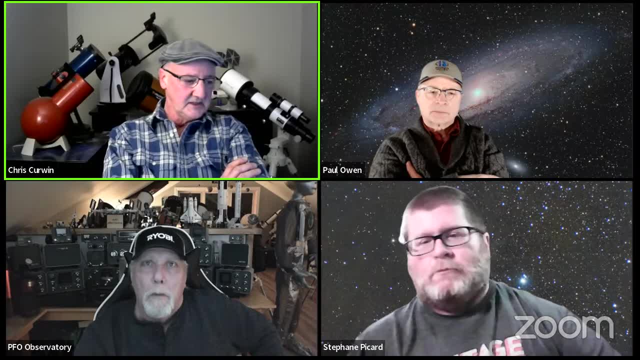 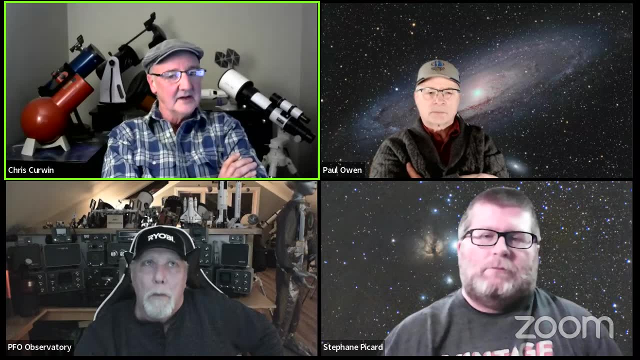 Patrick Moore was incredible, I think. when I look at Carl Sagan, he put it to poetry. He was very poetic in the way he spoke. He hooked me at Cosmos. i mean, cosmos is available. i know you can watch it on youtube right now and it's called cosmos. 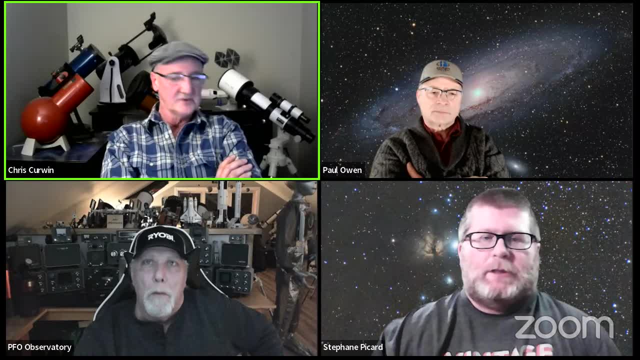 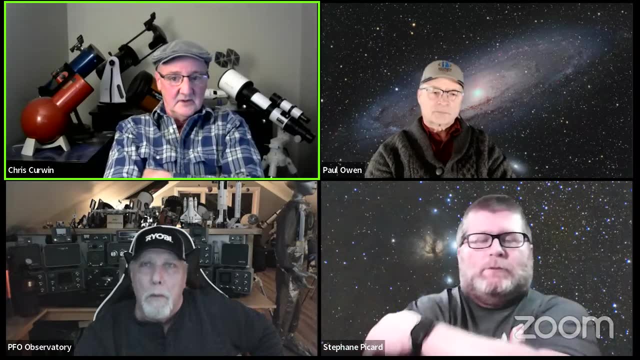 a personal voyage and uh was put out, you know, a number of years ago, but it's still a lot of the things that they they talk about are still applied. of course it was, you know, just after the voyager spacecraft, when the cosmos was, uh was released. so all the things that we've done since, 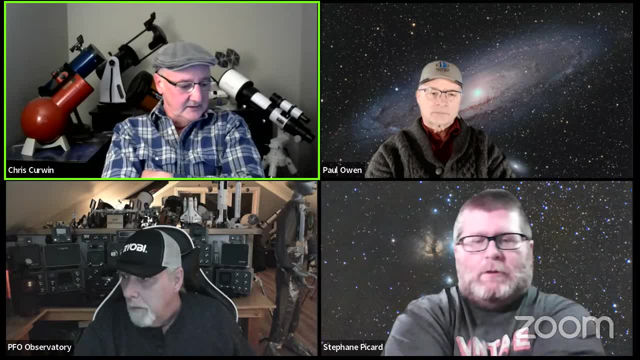 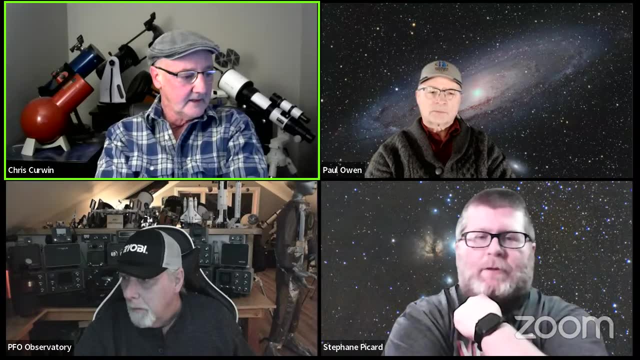 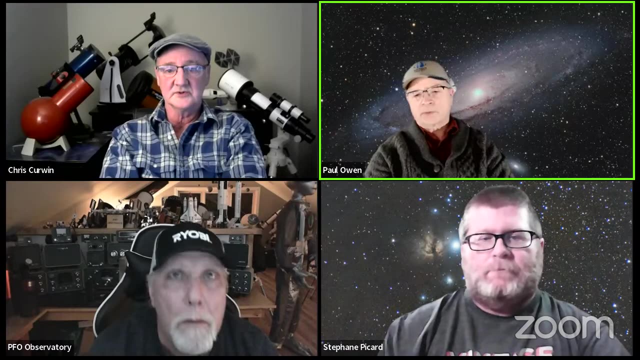 then web and everything has not been really involved, and, uh, neil degrasse tyson kind of carried on torch after that with his series of cosmos personal perspective. so, uh, i think, i think that he probably influenced me more than any other uh astronomer to me, well, there were two. the two 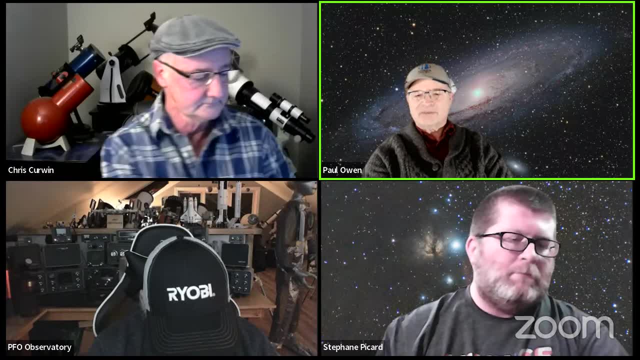 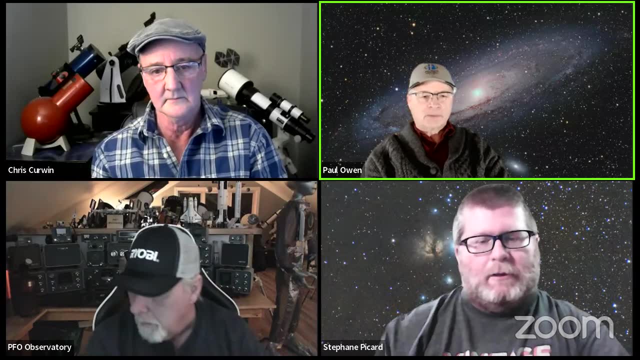 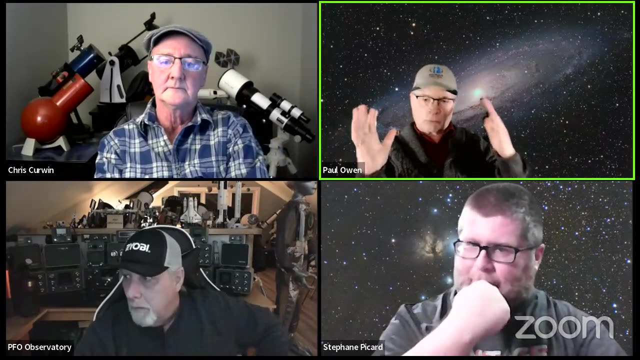 that we're talking about tonight were very, very different, even in their background, um, you know, whereas carl sagan was a professional in every way, yeah, yeah. and where patrick, sir patrick moore, was a teacher and a professional in his own right, but not a professional astronomer, certainly not a natural. 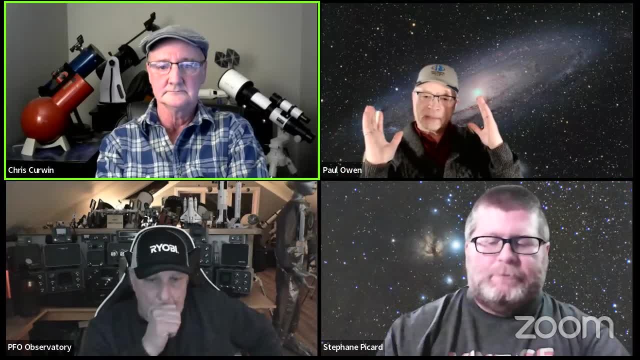 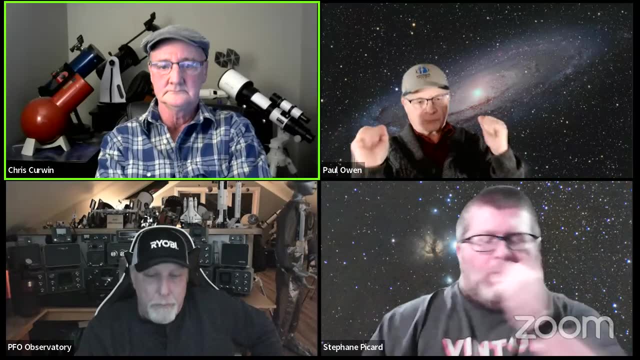 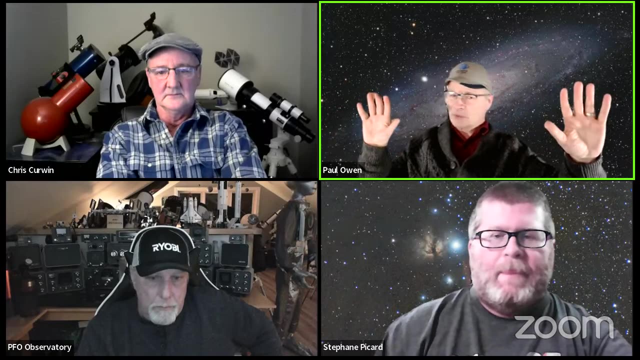 physicist or anything like that, but he was able to keep going for 55 years based on his um appreciation for what was out there and a totally different speaker. if you listen to carl sagan and then you listen to sir patrick moore, you almost have to be european or english. 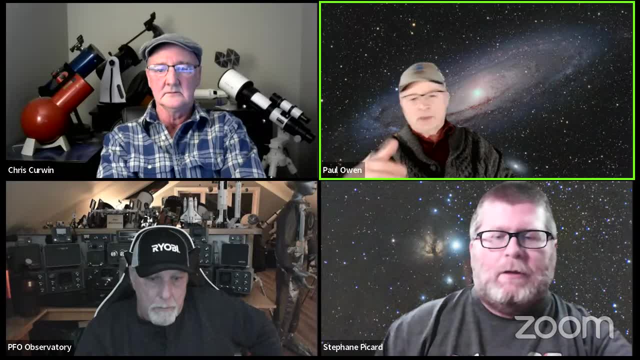 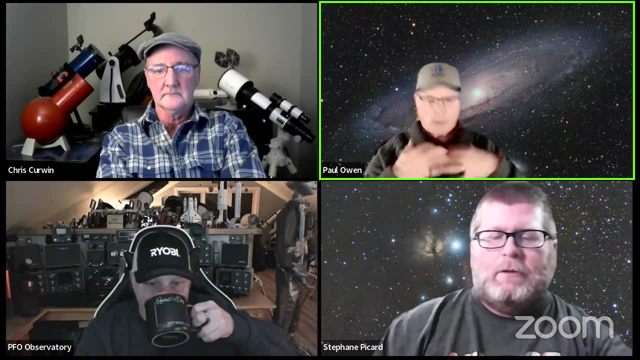 to really to really get what he's saying, because a lot of things that he's saying will have nothing to do with the, the type of language that's from over there. so that would be another separation from segan to him and from our perspective. right, exactly, yeah, i mean so. 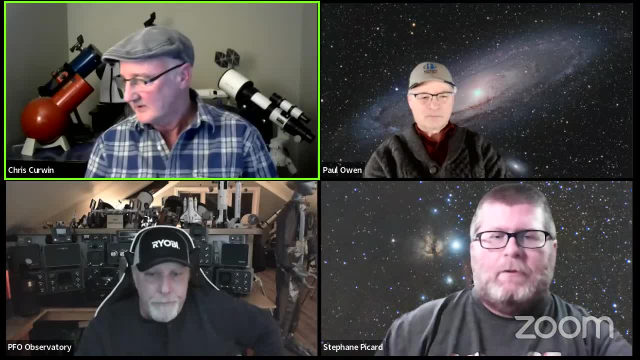 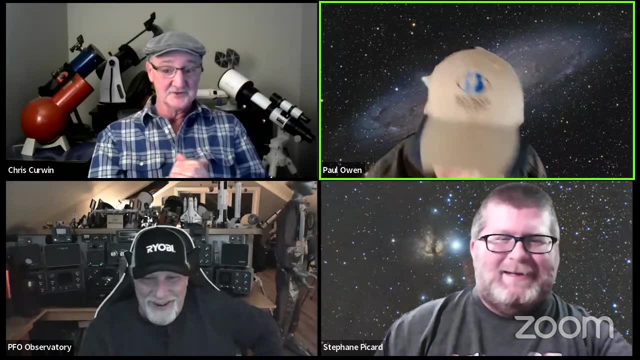 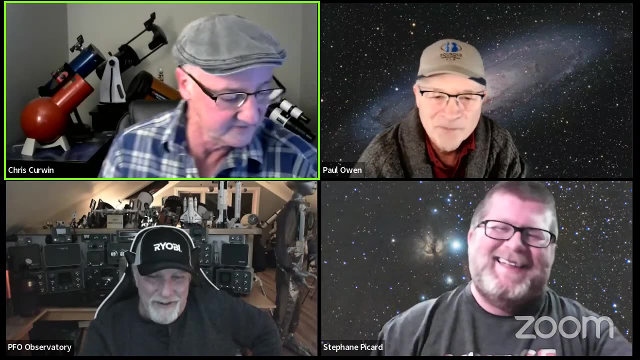 but anyway, but very, very important people, yeah, very much. so both of them, yeah, okay, i think we covered that. uh, we have another important person coming up here. oh, we do, yes, we do, that's right. modern astronomer. your next topic right after, uh, right after, right after stefan does his little bit of a talk. 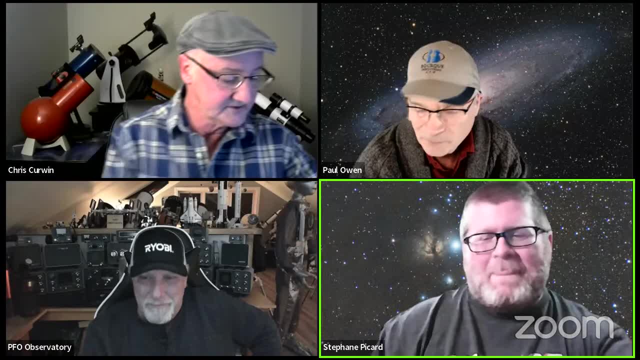 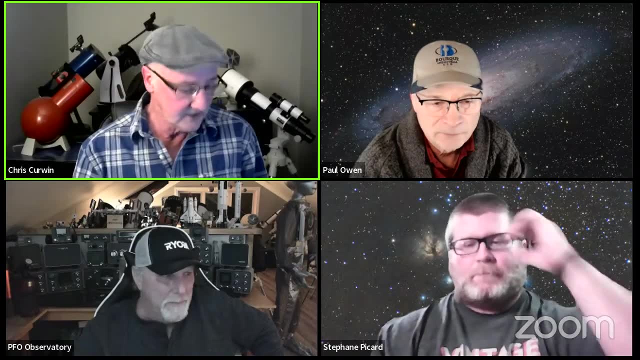 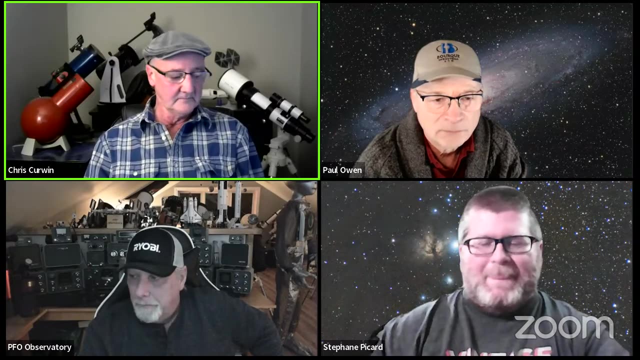 stefan, i'm going to introduce you next. i guess, sure, stefan is, of course, the uh the uh developer and producer and owner of uh cliff valley astronomy. uh, it's a uh a company that is uh reaching out into the astro tourism uh venture right now very heavily um stefan offers uh. 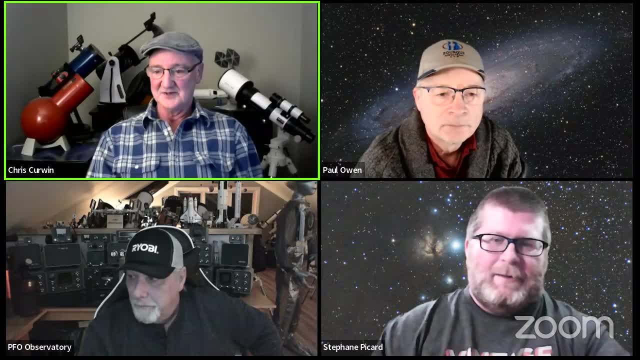 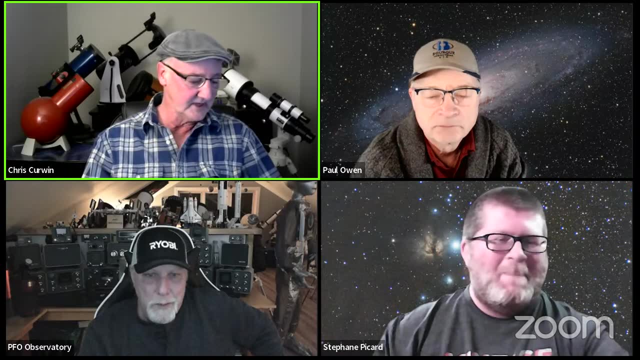 private star parties. that's how we started out, but it's gotten much bigger than just private start parties, uh, as of as of late anyway. um, and stefan is offering actually another thing called the sky experience 2024, which he's going to talk about a bit too. so, stefan, i'm going 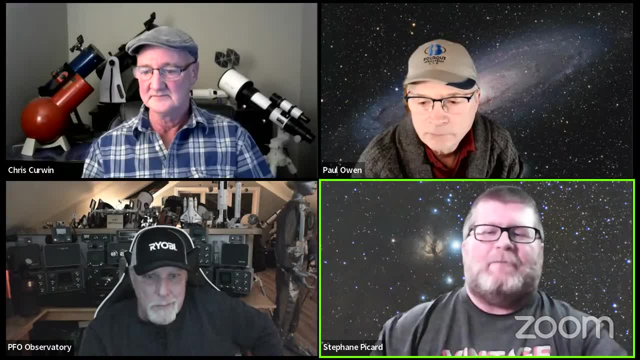 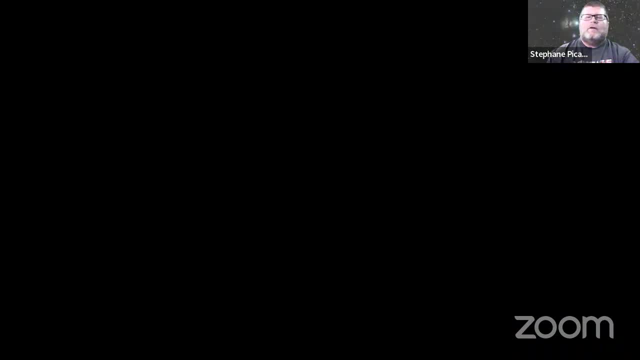 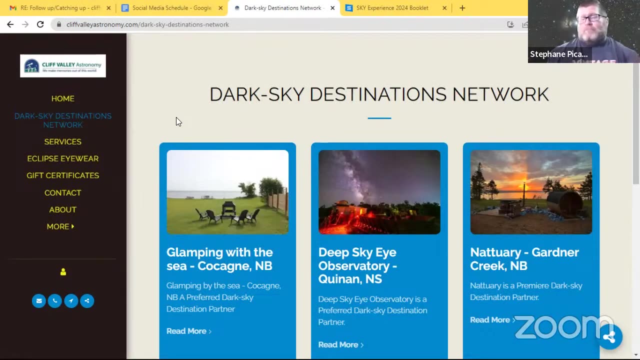 to hand it over to you now for sure. i'm just going to quickly present my screen because everything's on my website, right? so, uh, it will just be two quick seconds and, if you can, let me know if you see my screen, you're up and running. yeah. so, uh, if you go to my, we're really march this. 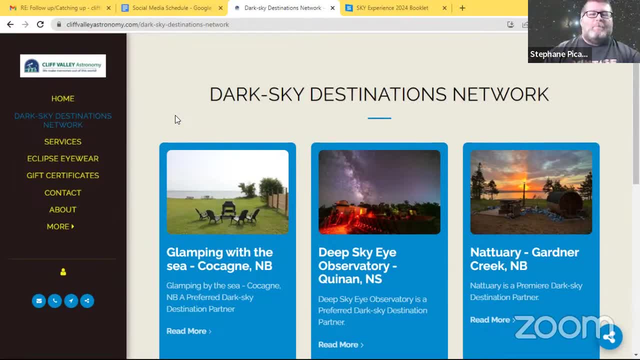 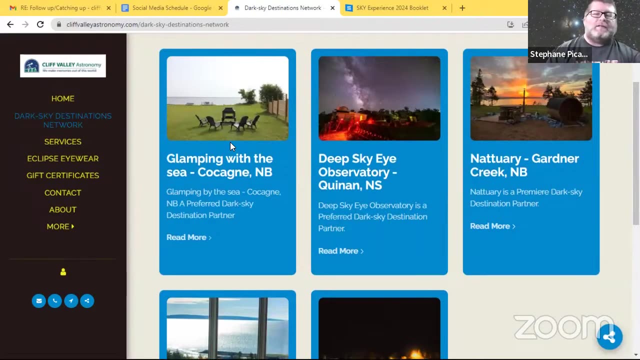 this march was really important. uh, earlier this month we uh launched um the dark sky destination network and i've started with five partners where uh we got four in new brunswick and one in nova scotia and these are identified as great places and um rural coastal areas where 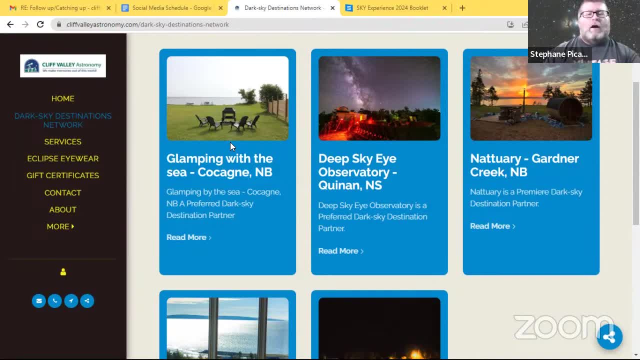 you're away from the glare of urban lights. so, uh, not only are they great accommodations that offer uh great activities or near uh sightseeing during today the day, you can also appreciate some great conditions, if the weather cooperates, of course, uh in the evenings. i've got five partners- we've been in touch with uh a few more- who are considering joining, but 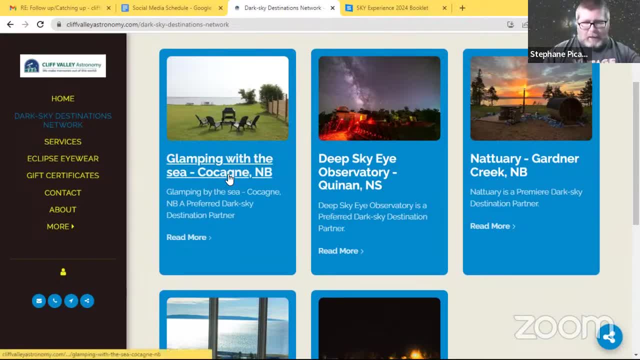 the first one we have is in cocai, which is uh near bhaktush, somewhere between or shiriak and miramichi, and it's a waterfront property. it's a uh- they call themselves glamping, but uh, they have a very good weather system. it's very well done and you'd be amazed at the uh experience you can. 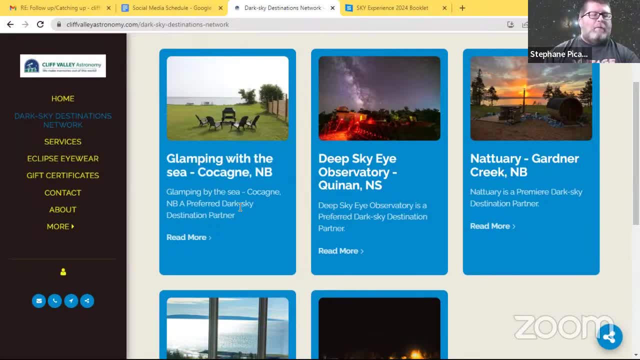 have there and, uh, they're seasonal. their season runs from uh june to the end of september. uh, after that we got deep sky eye observatory. our friend from uh quinn in nova scotia, tim duset- uh, he's got some pretty amazing uh accommodations there. the sky bubbles are put up uh for the summer months and 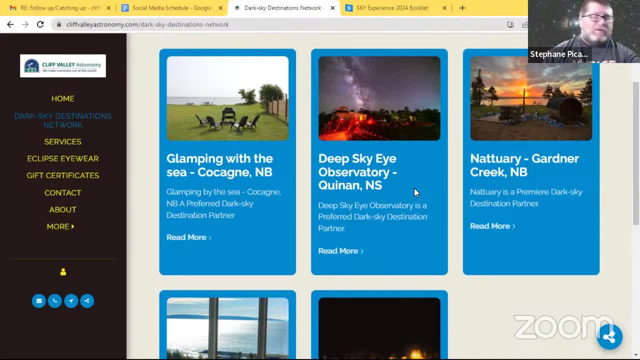 those are pretty amazing. he's got two- uh couples sky bubble which are perfect for a couple's getaway. all the sky bubbles have a ceiling window so when you lay down you got portal two almost conditions and you can see the night sky like amazing. amazingly, they do have also a family sky bubble and tim has a quite an impressive. 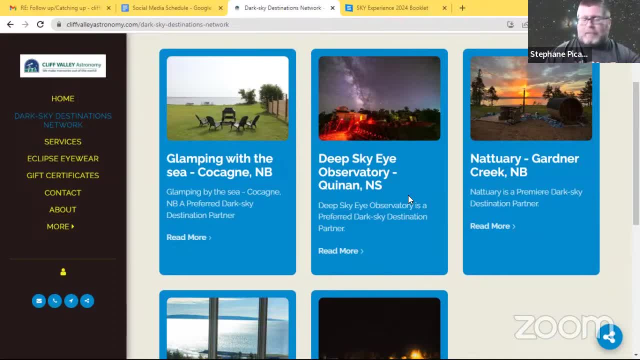 observatory and he does a nocturnal theater on many evenings, so totally worth doing the activity, sure, uh, we have another partner here near saint john, uh, in gardner creek. it's uh when you make your way heading towards, uh, saint martin's along the coast, uh, it's a beautiful spot, it's like uh. 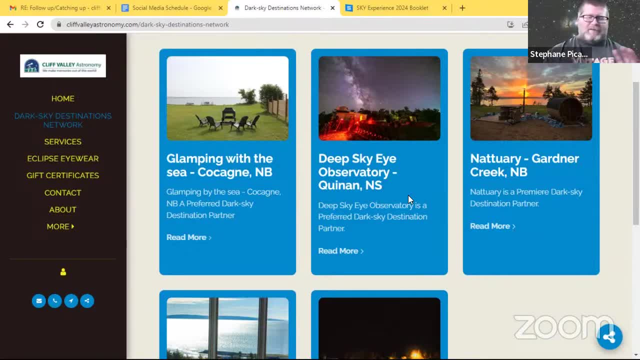 this modern slash nordic spa of a blend of a place where you have in one building your, your, uh, your bedroom and sort of a sitting area and you got really great, comfortable setting. and right next door, the building next door is where you got a full kitchen and a four. 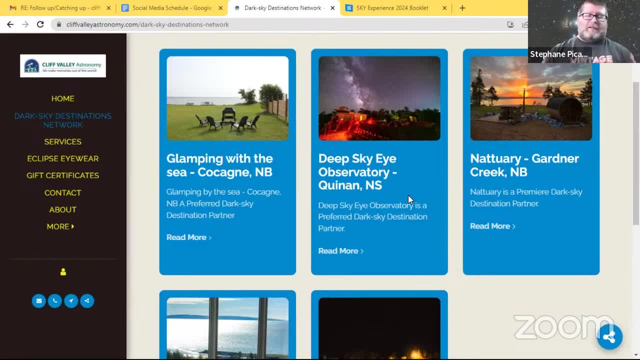 piece, bathroom and all that. but when you step out of the buildings you're facing towards the bay of fundy and you're facing southeast. you're looking at the distance at a rocky point called the split rock and i think we've seen some pictures on the show here of people taking pictures of the sunrise. 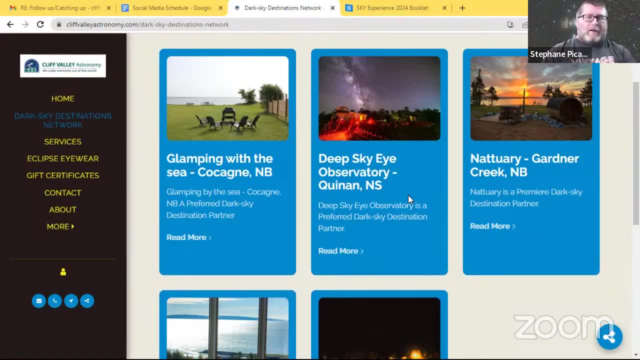 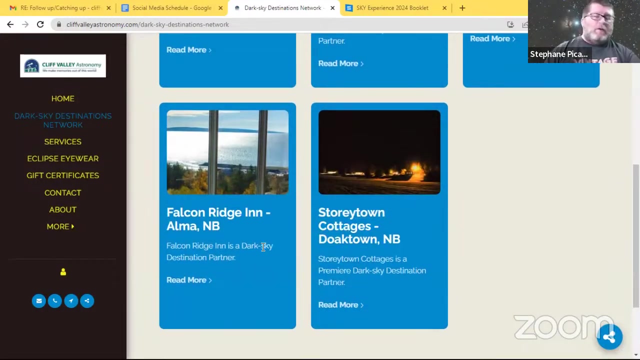 at split rock and all that. there's a wood fired hot tub outside and little sauna, so it's a perfect getaway and a lot of room, and you're high above on the cliff, above the water, so the conditions are really amazing there. uh, it's probably one of the darkest sights i've seen in the region, uh, at night, uh, and then we go to alma. 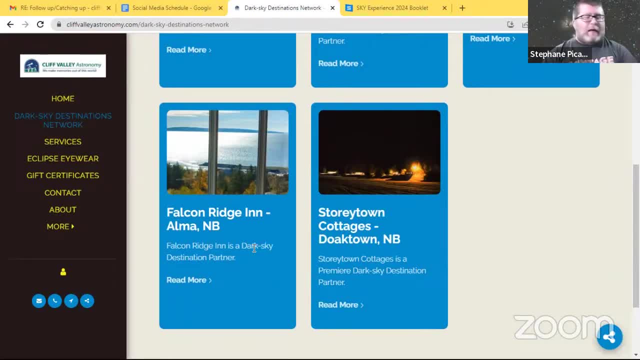 and which we all know, that fundy national park is a dark sky preserve and uh, one of the popular uh tourism operators in the area has even more and more and more of that is the uh uh tourism area. and in alma is a falcon ridge end. they're right on top of the mountain, overlooking the town, facing. 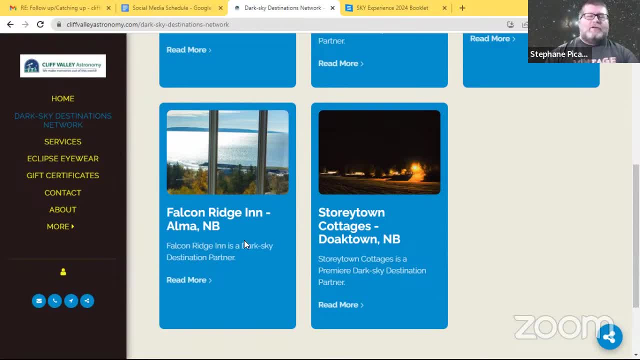 as you can see in the picture towards nova scotia, you're just minutes away from the uh funding national park for great conditions for stargazing and all that, and really bill and susan are amazing hosts too, so i would recommend, if you're planning on doing. 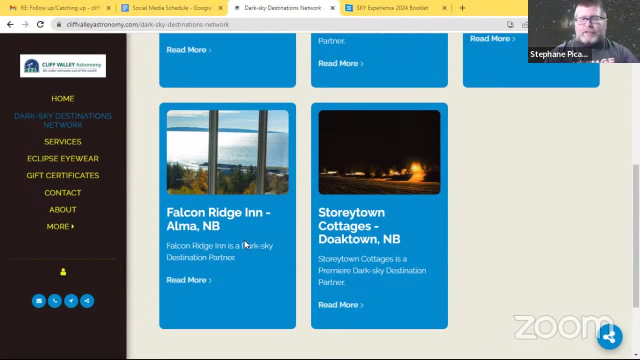 uh, funding national park or go to the region? uh, definitely, that's one of my top picks for sure, especially being a partner, and then one i'm very familiar with is in dope town. uh, story town cottages. it's a campus of cottages and the main building that offers sort of like hotel suites or 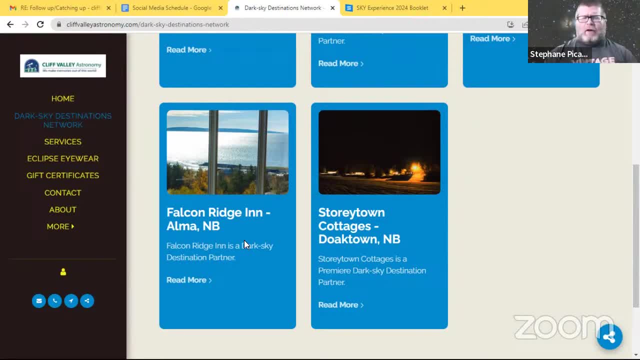 a kitchenette suites and it's a huge private lot. it's on the north side of the river. all the cottages and the uh uh the buildings are sort of facing south, so at night you see everything rising. you're outside the town of dope town a little bit, so it's quite dark and they have a huge field in front, uh, of the. 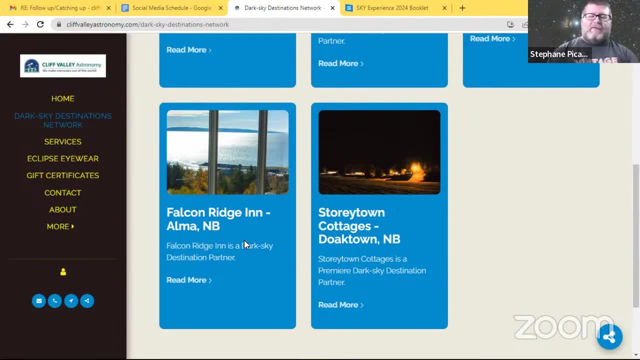 property that goes down to the river. if you go halfway down that field, you have amazing 360 views all around. i know, when i've gone there personally myself, i've always brought my camera and my telescope and it's just amazing. and these guys are open year-round. so these are my partners. more will be added. 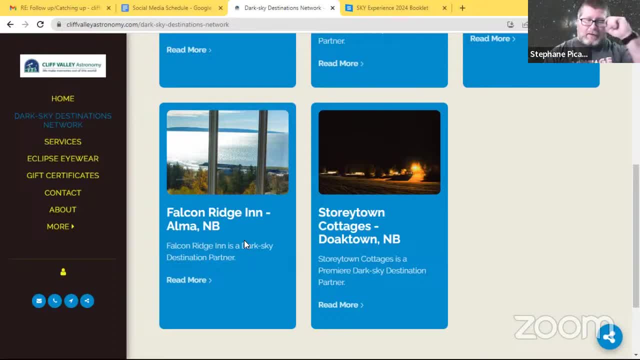 in the uh coming weeks and we'll be excited to make those announcements. some are seasonal, some are full, uh, year-round. uh, they're booking up fast. there's already uh somebody i was talking to that was looking to book at enalma for the rasped star party and unfortunately they are all booked up for. 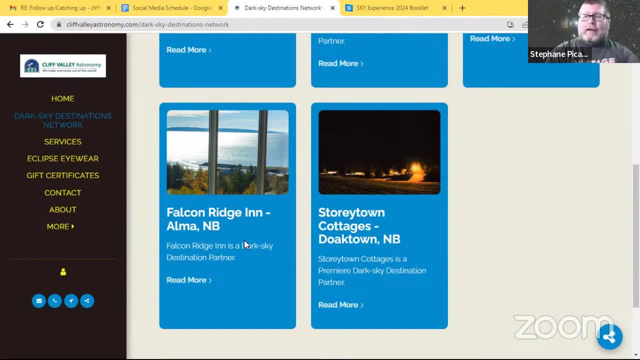 that weekend. so, uh, don't wait the off-season, the whole- you'll see how discount에는 Deals are on right now for the ones that are open in the spring and in the fall, and they're fantastic deals. You can book through us on the website here, or you can book directly. For example, if you book a naturalry, if you book with Airbnb, if you decide to book through Cliff Valley Astronomy, you would save over $100 because you don't have to pay the Airbnb service fee and also they charge a cleaning fee. 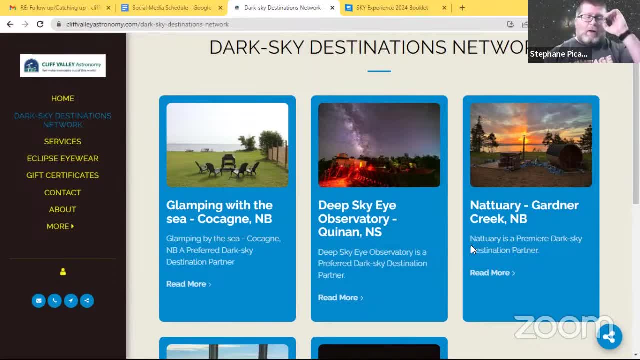 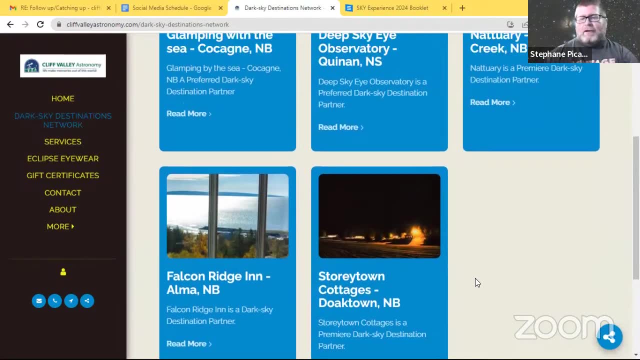 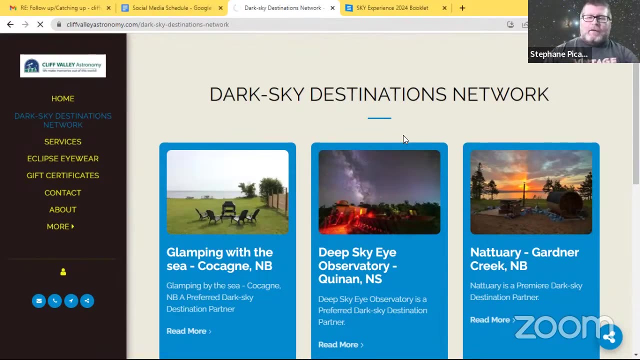 But through us we don't have that cost. so there's opportunities and some of these partners you can book directly, obviously with them too. So that's really our first dive into astrotourism, And then the really big dive is the event that we're going to do for the Eclipse next year. 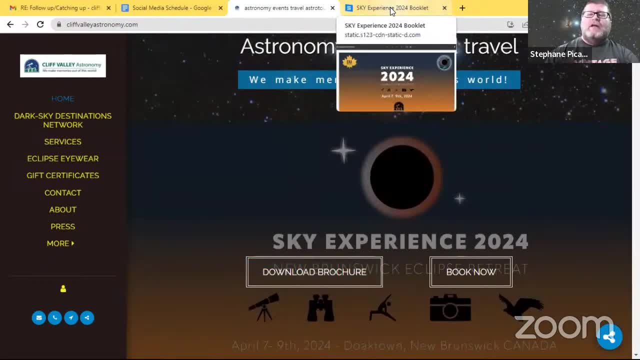 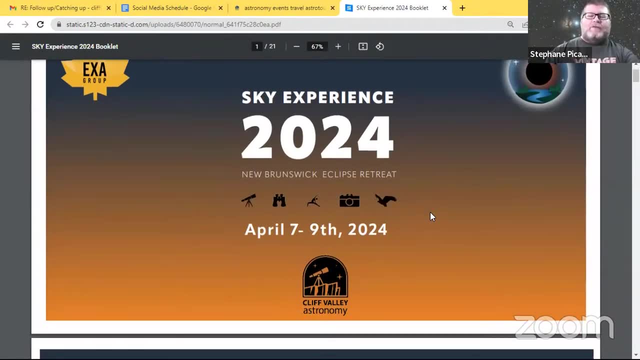 We're coming back to Dope Town for discussion and we've launched earlier this month, This past week, the announcement of our retreat that we will be doing around the total solar eclipse that's going to visit us next April of 2024.. 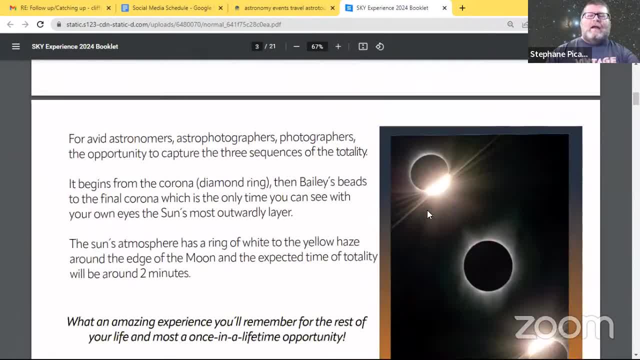 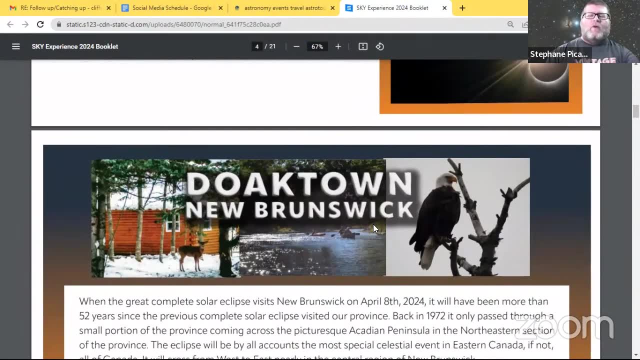 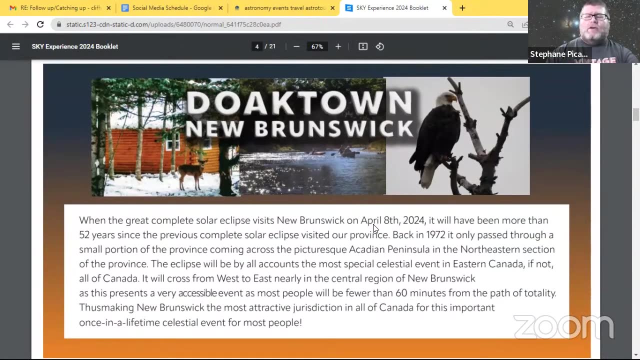 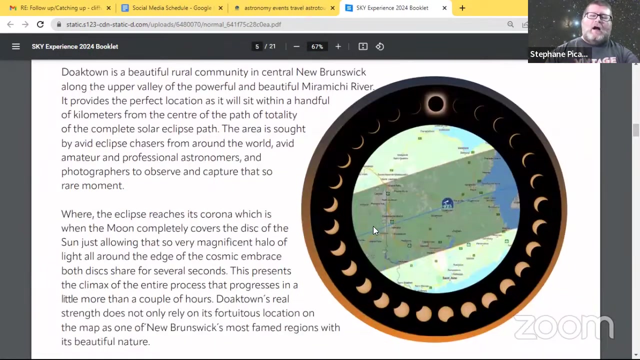 So I've been working hard on building a unique experience that would provide a lot of value for people who would want to come to New Brunswick, because I think New Brunswick will be the best jurisdiction in all of Canada to experience the total And because I was so familiar with Dope Town. you can see the path of the eclipse here, where you see my logo. 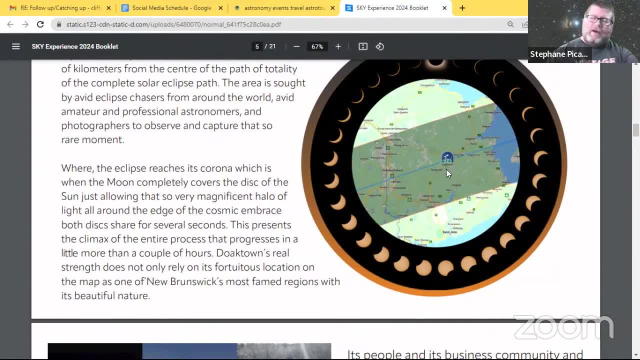 That's where Dope Town is and that's where Story Town. So if you're an avid eclipse chaser, astronomer, astrophotographer, and you want to have the best view of the total eclipse for either just viewing, taking the picture, taking the video, whatever, we are dead center there. 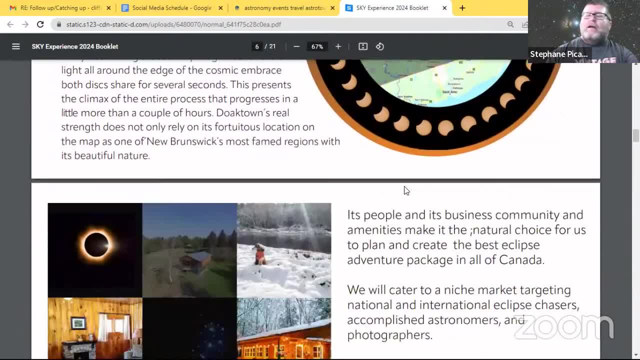 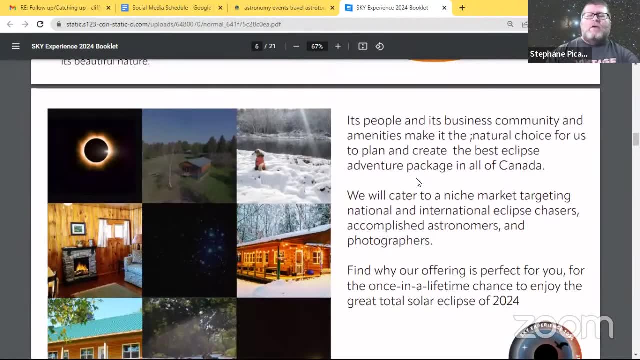 And we will be. We will be in a natural setting in Dope Town where there's lots of wildlife- the eagles, the deer and all that- So you'll have also the opportunity to experience how the wildlife is going to react to it. 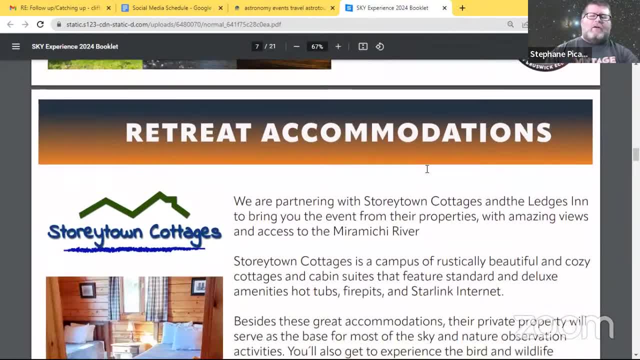 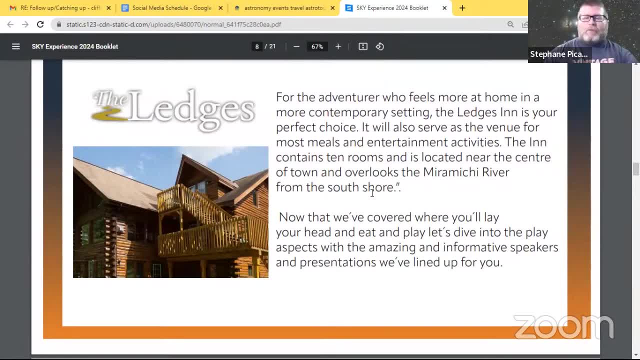 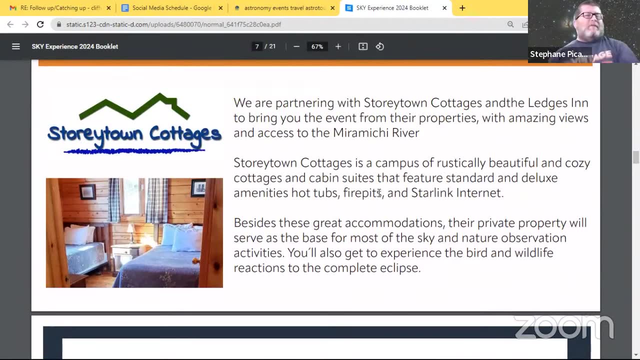 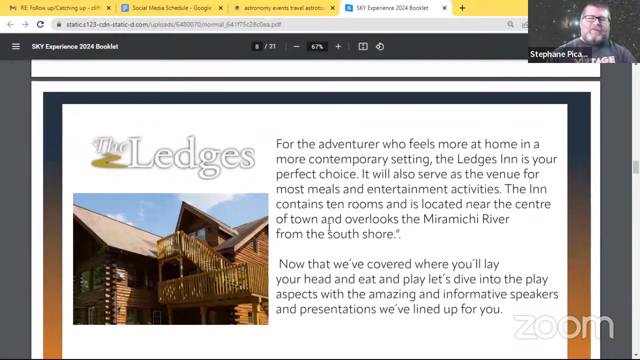 We've also added a second partner for the accommodation, which is the Ledges Inn, which is also a very popular and renowned tourism operator in Dope Town. So that gives great Choices for if you like the style of being in the cottage or if you prefer being in more in the one building, sort of like in slash hotel. feel fields, sorry feel. 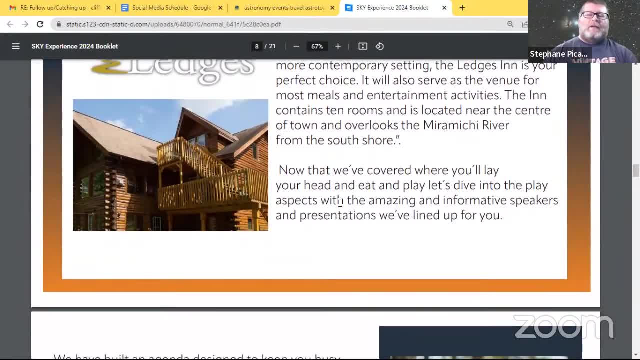 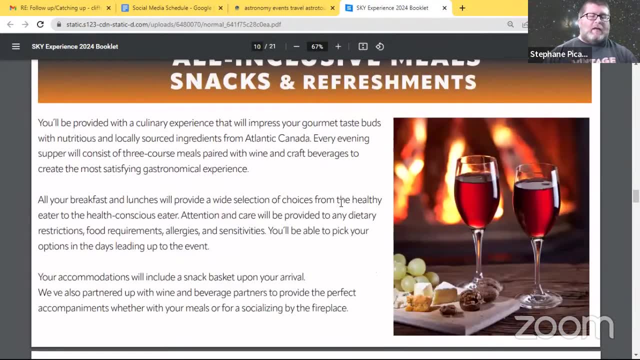 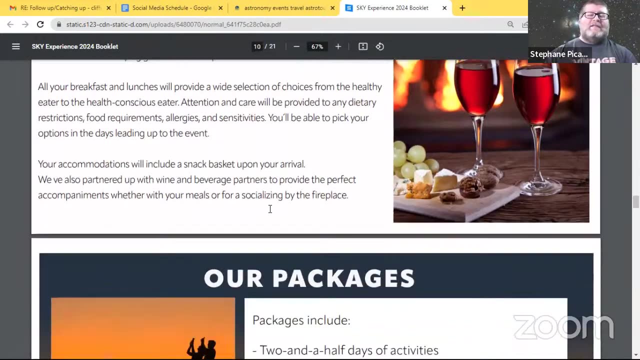 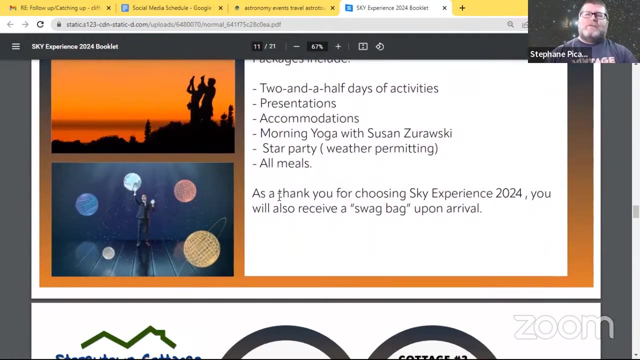 Then the Ledges Inn is also a great, a great place to be And we will have some various activities. We're providing all the meals, So it's turnkey. Your cost for your package includes your accommodations, Fantastic food, All the activities. and really what really started really feeling like it was falling into place was once we started approaching speakers and presenters and all that. 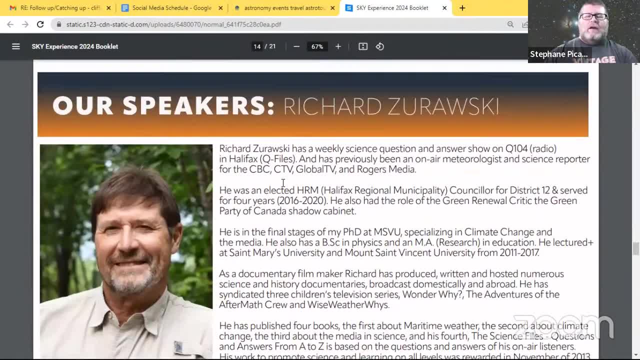 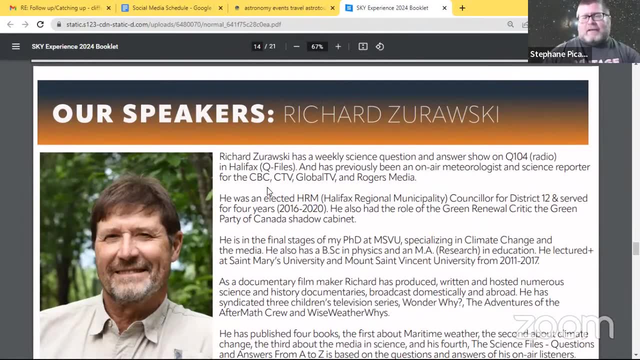 And I'll come back to these. I was really excited to approach Richard Zyrowski, a well-known meteorologist out of Halifax. a personal radio personality. He's currently on the Stingray radio fan Family stations across the Maritimes right now. 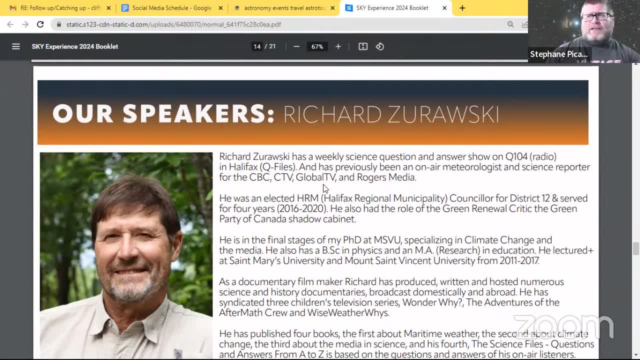 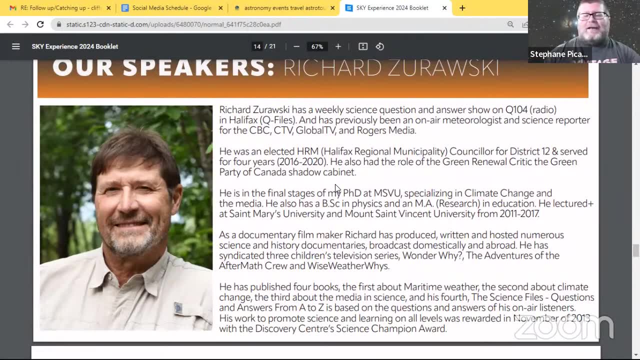 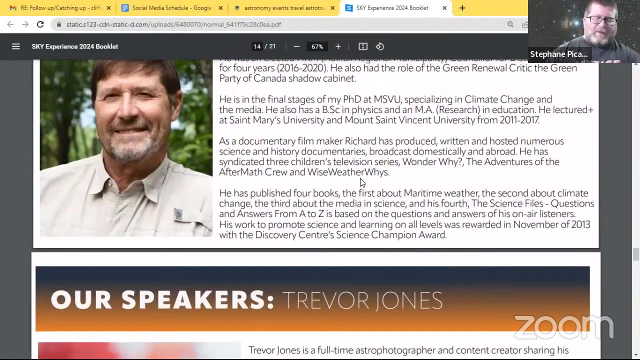 He was on Rogers. He's a. he's a meteorologist, but he's really a scientist. You know he's got an amazing. He's definitely an overachiever. He's right now still doing a doctorate and really engaging and fascinating science figure in our region. 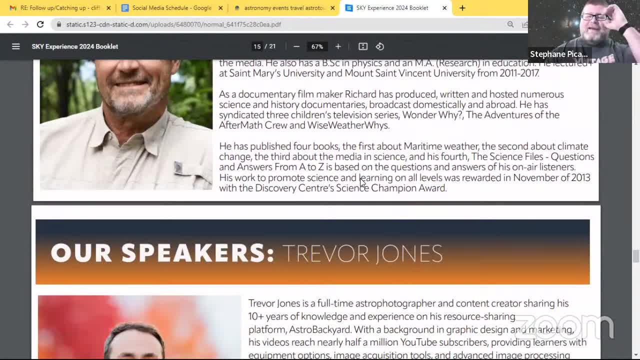 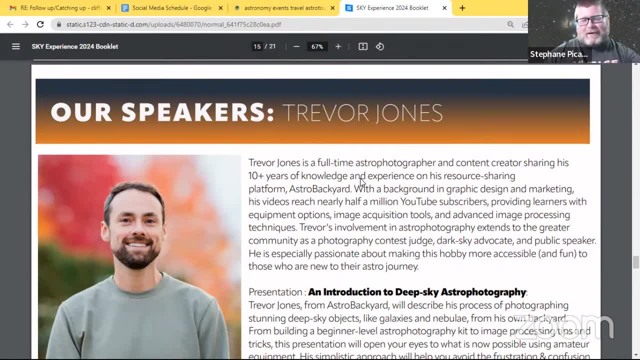 So he's well known. So he said, yes, he's all behind it. And then, to my second surprise, was I approach a well-known Trevor Jones out of Ontario. He started Astro Backyard dot com. He's got a website. that he's all. he's probably the one of the best known astrophotographers in Canada. 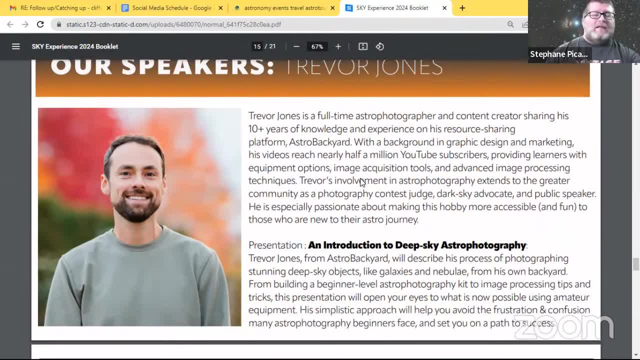 He's been on YouTube for a few years. He's built quite the following. He's at over four hundred and twenty one thousand subscribers to his YouTube channel And, like me, he's a astropreneur at him And his wife started making the business of it. 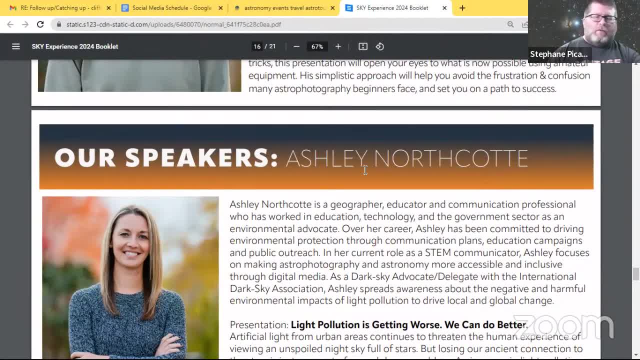 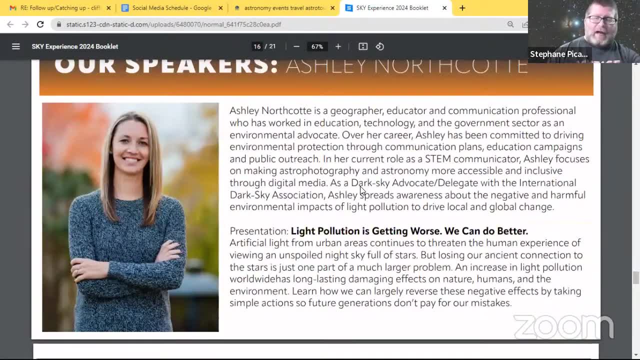 And they develop content. They review equipment with manufacturers and they're having a lot of success. And this is his wife, Ashley. She will be doing a presentation also. She's a big dark sky advocate like me. She belongs to the IDA and she's really passionate. 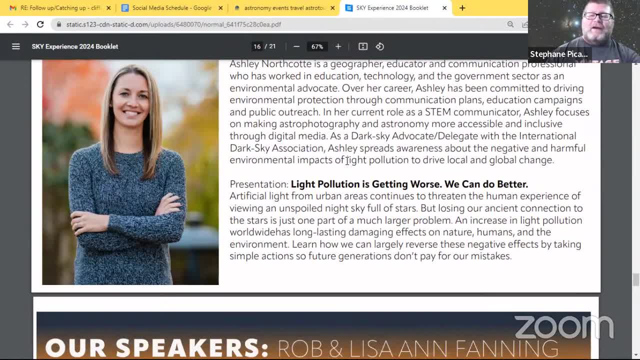 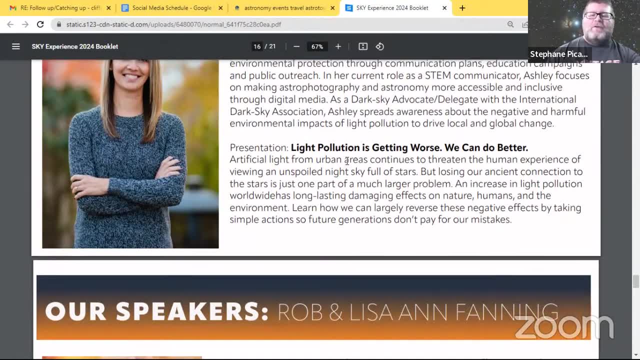 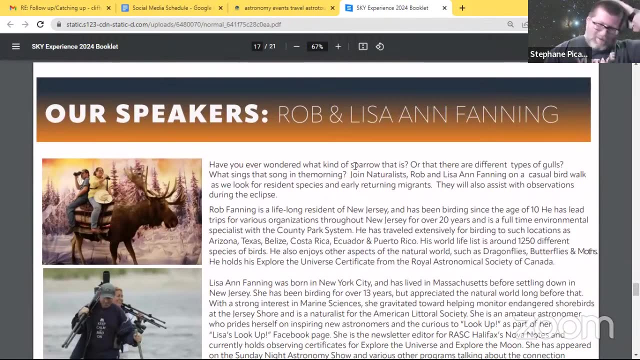 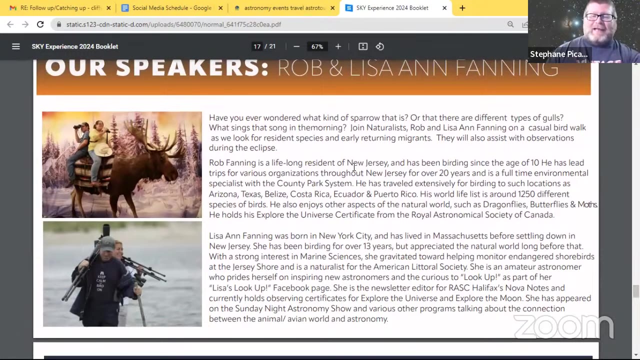 So that's going to be really interesting to hear what she has to say on the subject of preserving our nocturnal space guys as much as possible. and then we have uh well known to us here, uh, on your show, chris and mike and paul, uh lisa and rob fanning out of new jersey. they're, uh, as you know, uh amateur astronomers, and 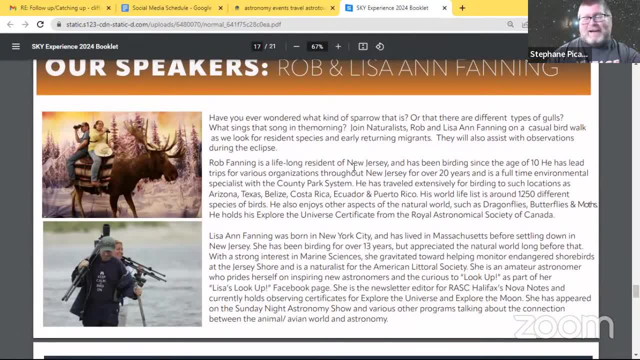 expert birders, so they're going to do a presentation on birding and take us on an excursion to see the uh- the flying uh- wildlife, if you will. in doketown there's bald eagles. there's countless types of birds. it's a beautiful part of our province so that'll be a fun. 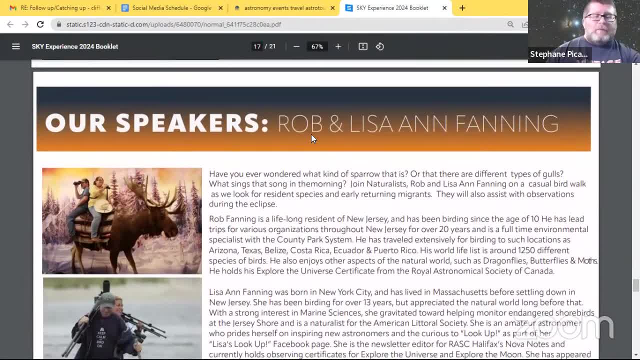 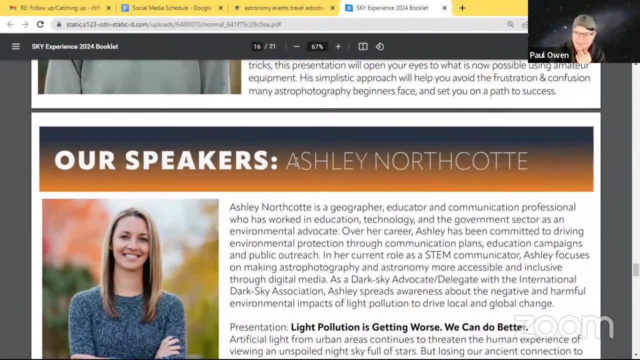 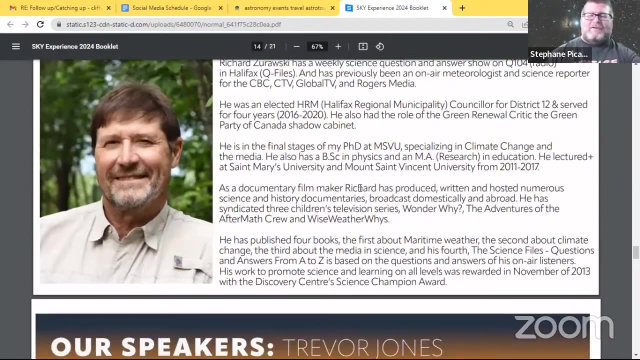 activity. uh, we've also added morning yoga classes, just for paul. i think paul would like that now and uh, anyway. so we're still building the agenda. we're gonna have an amazing two days. it starts on april 7th. we'll conclude that on the 9th. the eclipse is on the 8th, so that's. 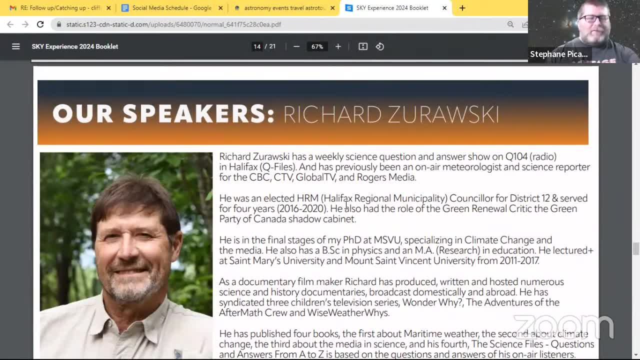 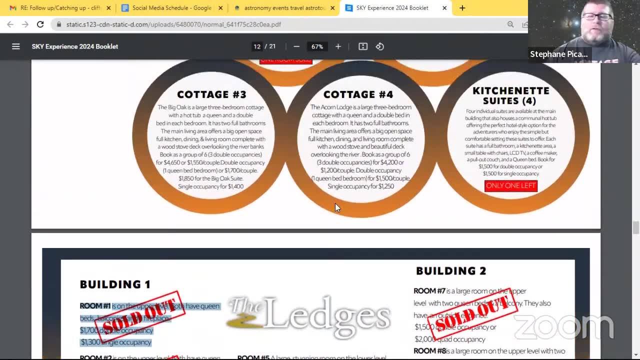 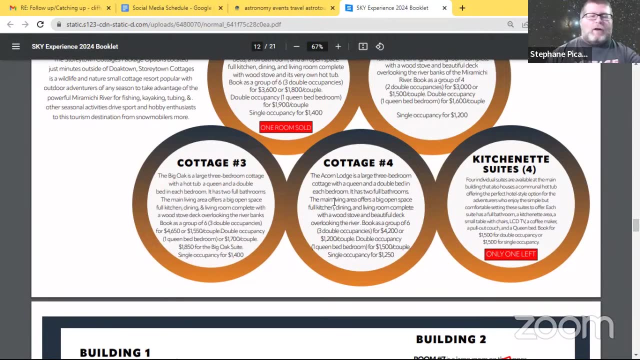 going to take a chunk of the agenda on the 8th afternoon. uh, i heard some people say: well you know, is the weather going to cooperate? the thing with a total eclipse- even if you're clouded over, everything's going to get dark. every wildlife will react to it. uh, we're going to have a contingency in case the weather doesn't. 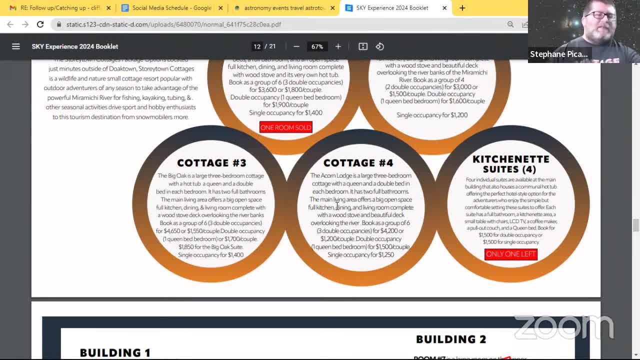 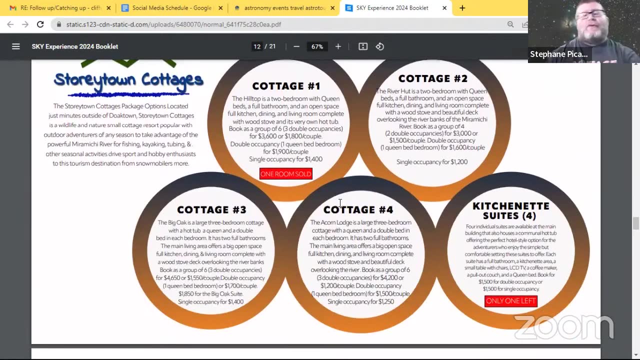 cooperate that we could sort of have a live stream coming in but still experience the darkness and being in nature and all that. so, uh, and you'll be surrounded with like-minded people. uh, we started selling, like i said, this week. we're already past the third way of uh packages sold. 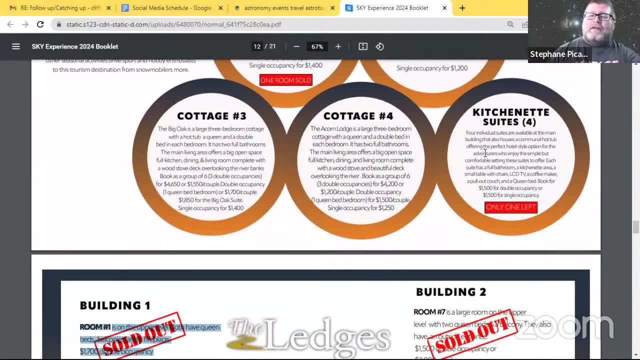 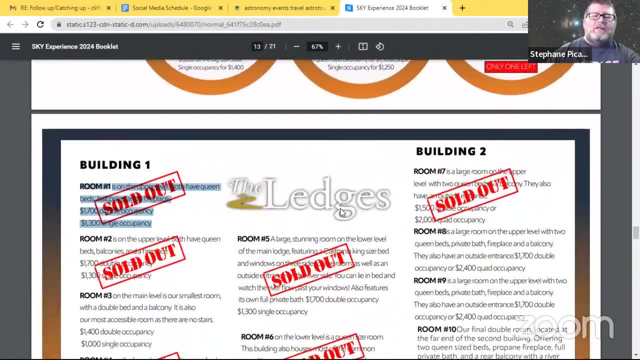 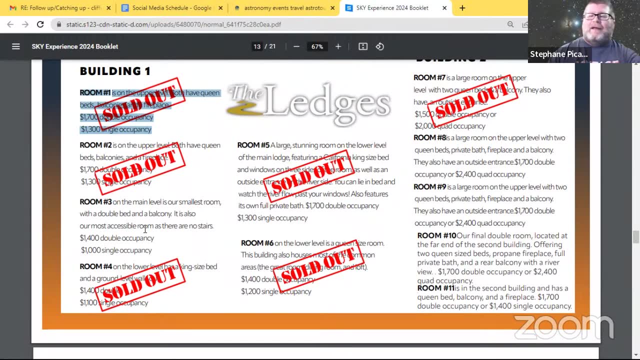 uh, we got um one kitchenette suite left at dope town amongst the four. uh, we've got a commitment on half of one of the cottages and at the ledges in we now have, uh, seven rooms, because i sold room three this morning. so it's moving fast and you know, i uh, we're, we're. 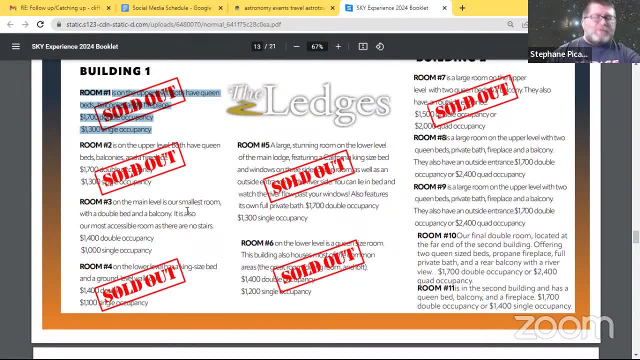 really trying hard to uh create a exceptional, unique event that you'll remember for sure, on top of being, you know, one of a once in a lifetime event with the eclipse, and uh, we're hoping that if at the rate everything is going, we might have to add a third location to accommodate. 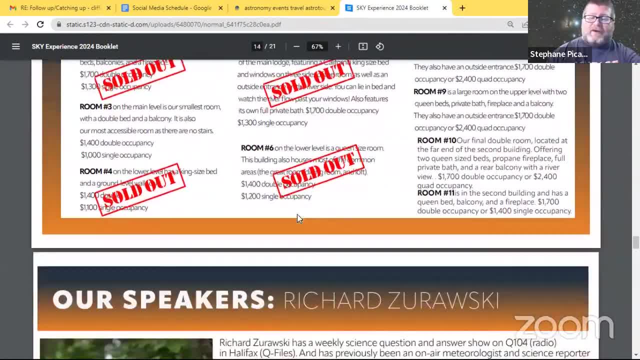 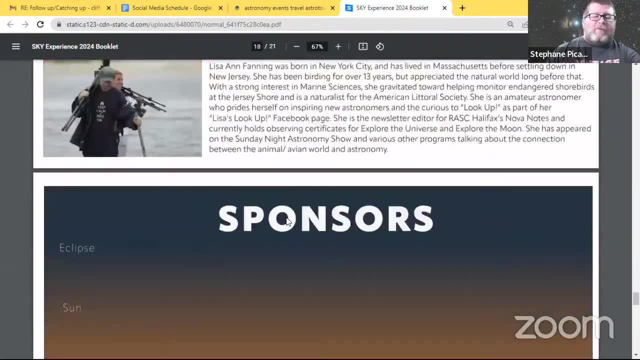 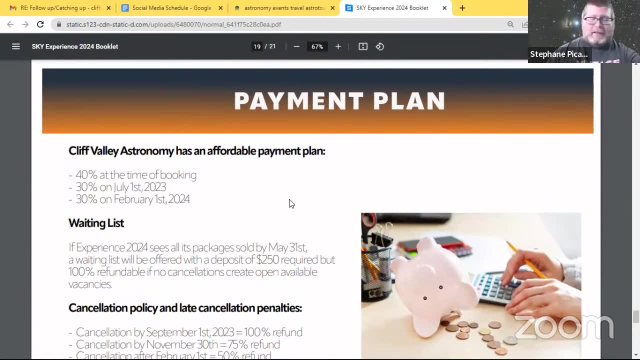 more people, but, uh, we're very enthused and very happy to with the way things are progressing out and, uh, we offer payment plans and there's going to be some sponsors being announced, so we're making this as feasible as possible. it is a little bit of an investment but, at the end of the day, for 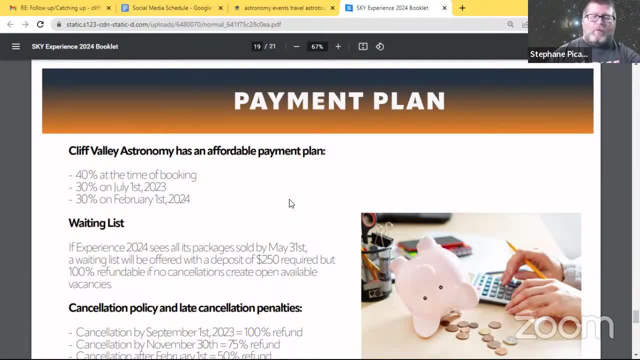 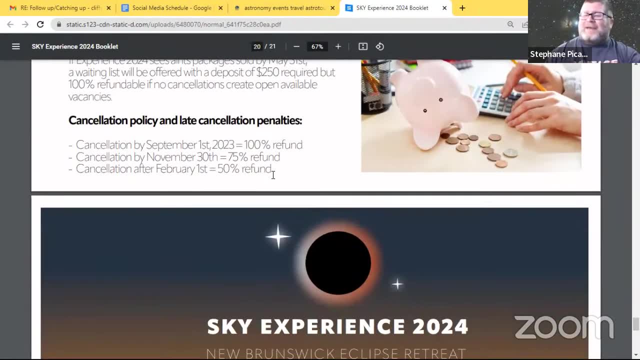 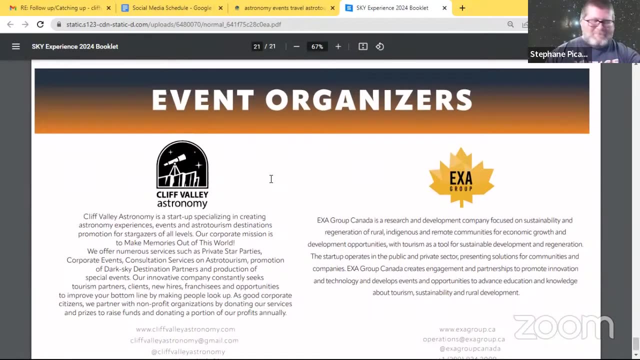 the value that we're going to provide and the experience. it'll be well worth for a once in a lifetime opportunity, right? so? so that's my spiel. i tried to keep it short, chris, so it was perfect. uh sounds awesome. yeah, you've. uh, you made some real good headway on that, for sure as well. yeah, this has been in. 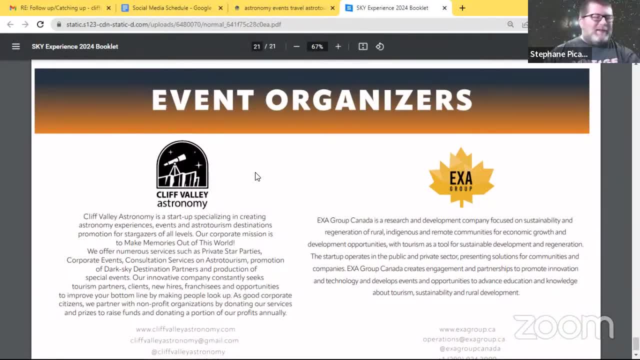 the plans for a while. so, uh, yeah, a lot of father's been given to it. yeah, it's a fascinating event. it's going to be fascinating event, uh, you know, if you stand on the earth. apparently one uh once in your lifetime. no, sorry, uh, it won't even happen once in, like maybe every 375 years when an eclipse. 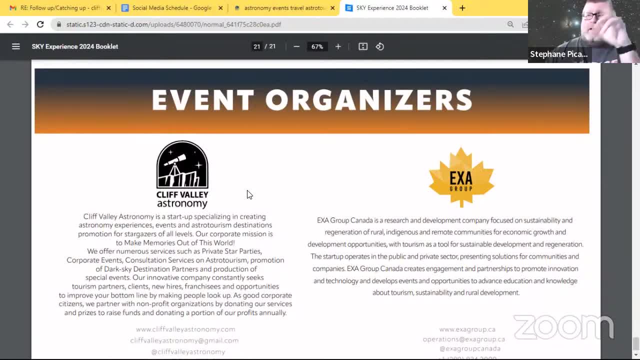 passes over your head. yeah, and just to point out the last little bit: yeah, the last total solar eclipse that passed through new brunswick was in 1970, i believe, and they only passed a short portion of the acadian peninsula, so quite a bit of the province missed it then. so this is definitely 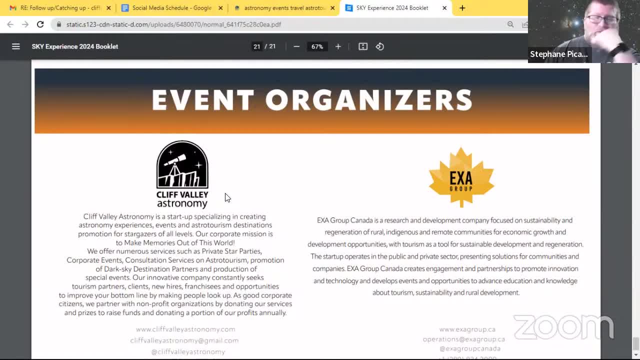 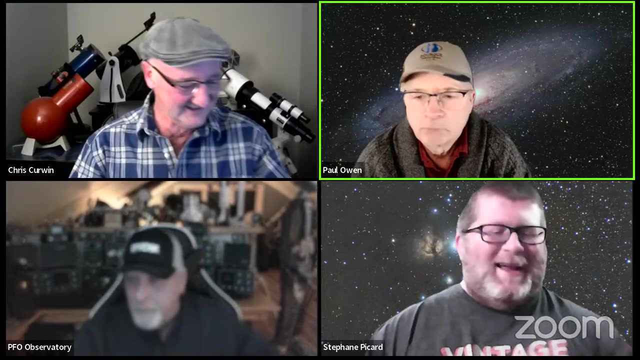 more than one in a century or plus more years of an opportunity, right, yeah, yeah, fantastic good stuff you're doing. uh, you're moving it right along. yeah, well, thank you good. oh, and one last thing i'm also. uh was the interview subject for, uh, the night sky tourists. 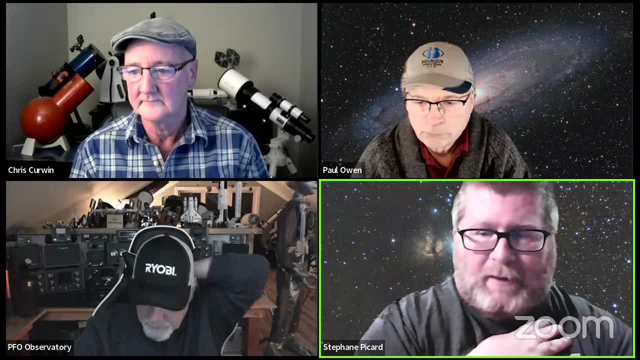 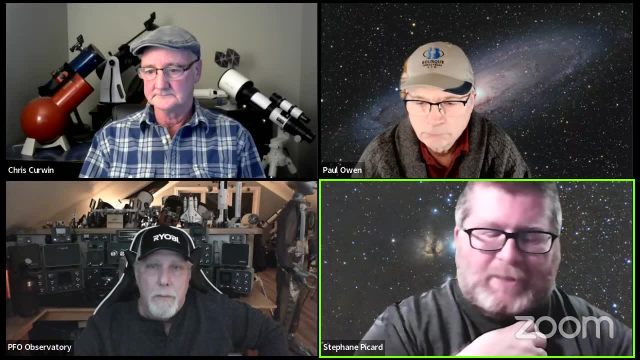 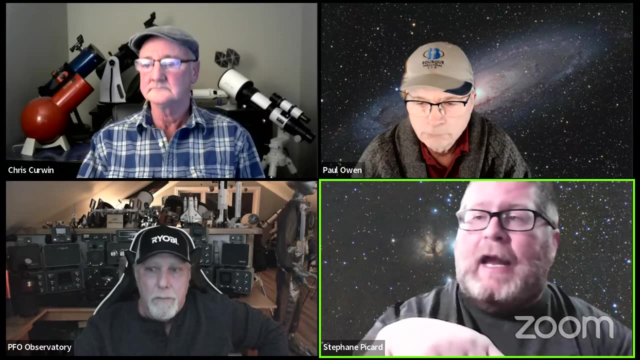 uh podcast. uh, which is a lovely lady, uh, vicky derson, out of uh arizona, and uh she stumbled across me. she thought was pretty fascinating so she interviewed me a couple weeks ago. that podcast will be going live tuesday and uh again, i'm just excited to bring new brunswick to. 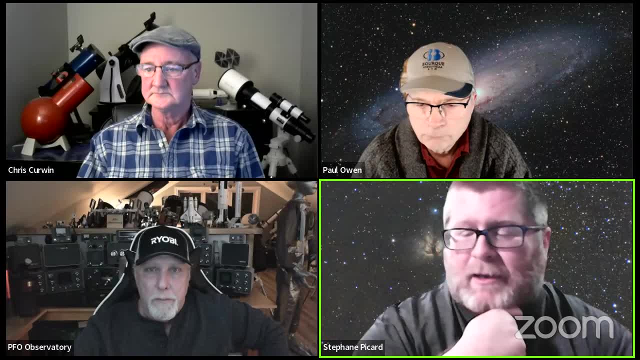 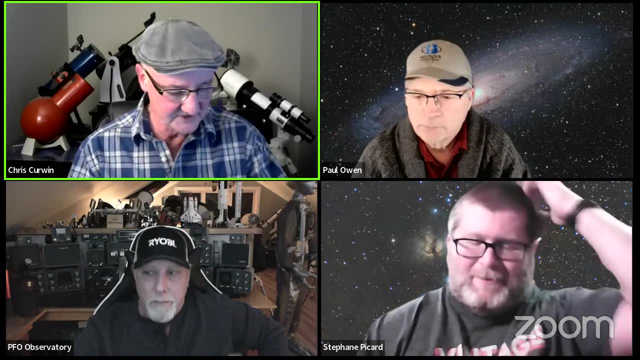 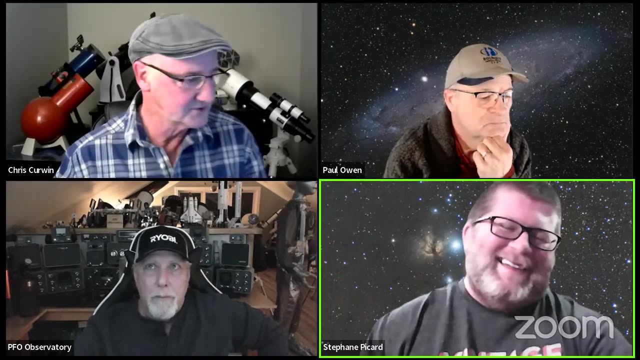 the rest of the world, because we have some really neat uh assets here from an astro tourism stand. well, no doubt you're doing your part, sir. yeah, awesome, thanks, my pleasure. thank you, hey, john. luck, sir, for the rest of it, i'm sure you'll do. it's going to be an amazing event for sure. we're all looking forward to it. 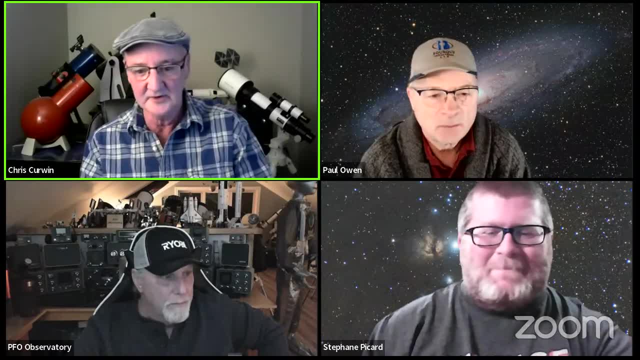 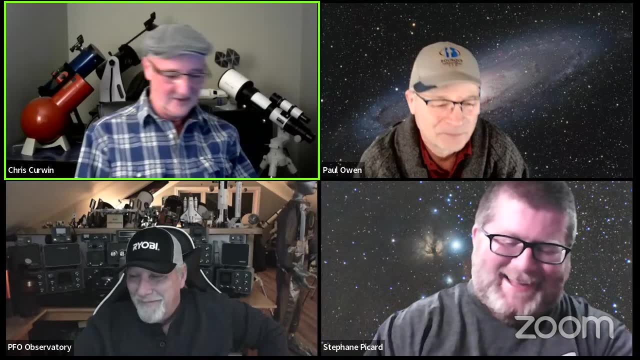 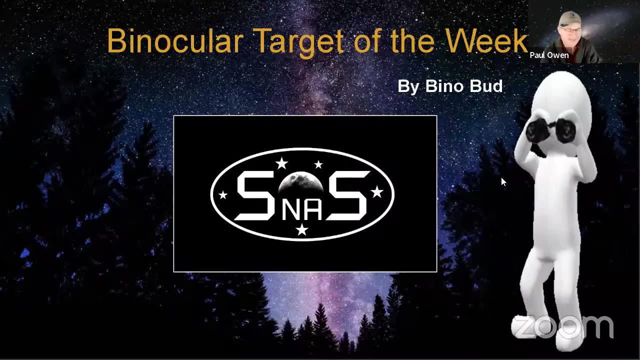 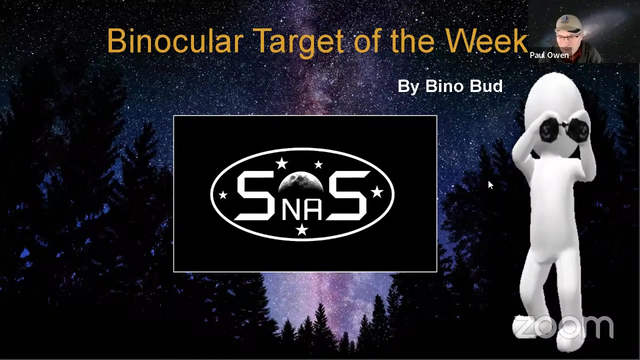 okay, um, our third monitor astronomer, mr mike, is going to introduce our next astronomer on the tablet: vinyl bud, hopefully coming up here. sir patrick moore, carl sagan and vinyl bud. i know what. what can i say? i'm right up there in the big leagues with 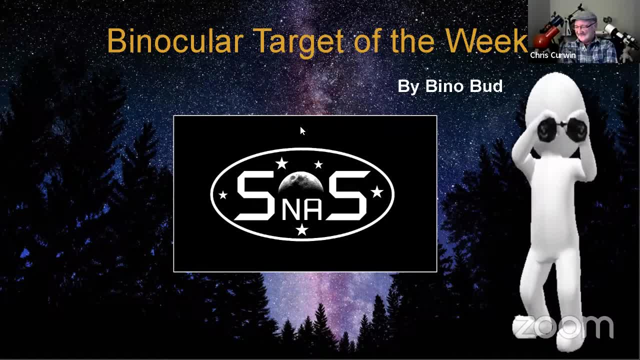 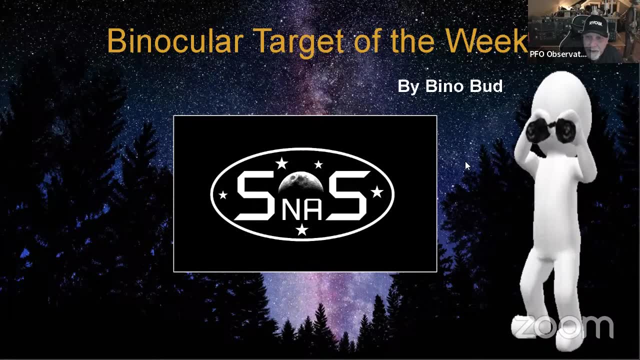 this guy all righty well, you'll all recognize this one, but it's you know. it's been a full 365 days that we've gone in a circle and now he's back. so binocular target of the week this week by bonobon is the smiley face. 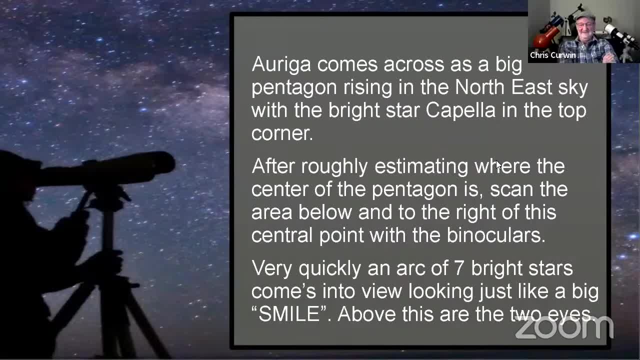 and it looks like that it really does. auriga comes across as a big pentagon rising in the northeast sky with the bright star capella in the top corner. after roughly estimating where the center of the pentagon is, scan the writing area below and to the right of this central point with binoculars very quickly. an. 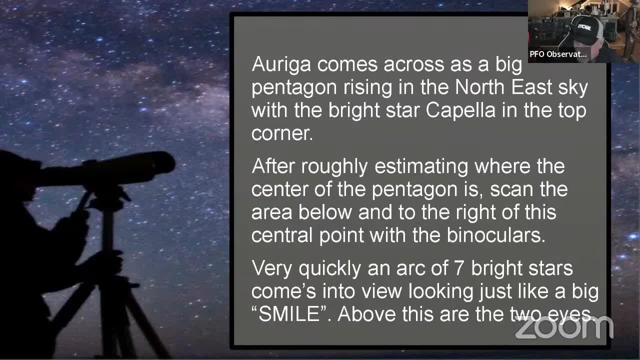 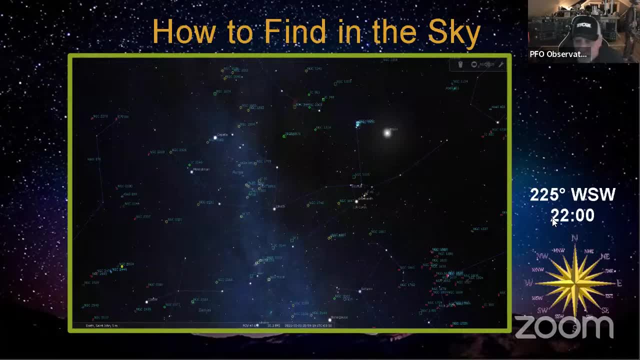 arc of seven bright stars came into view, looking just like a big smile, and above it are actually two eyes. now how do i find it in the sky? well, if you're outside tonight- and it was starting to clear, but i don't know if it's clear yet- but at ten o'clock, oriented yourself at 220 degrees west. 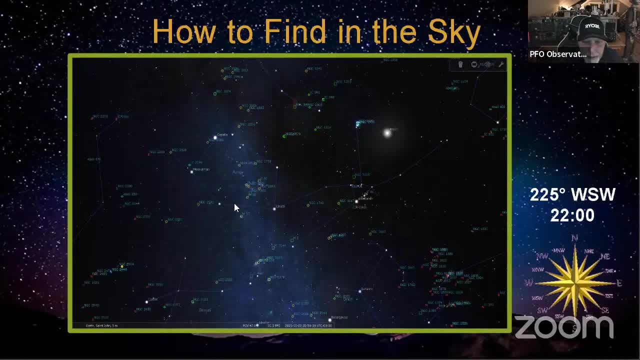 southwest pretty much looks straight up, you're gonna find a arrival. there's that pentagon kind of looks like baseball plate archipelago. you come down about two-thirds through and the smiley face is right in this area, right in here, very close to the- uh, the fish that we talked about the other day, because there's the, the jumping. 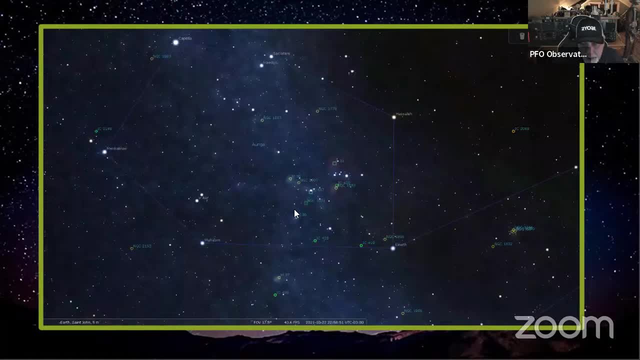 fish. well, guess what? m36 and m38 are right together and here's a smiley face right in here. one, two, three, four, five stars of makeup, the big smile and then two eyes right in there. what will you see? well, look at this roughly. this is almost what you're going to see in a pair of 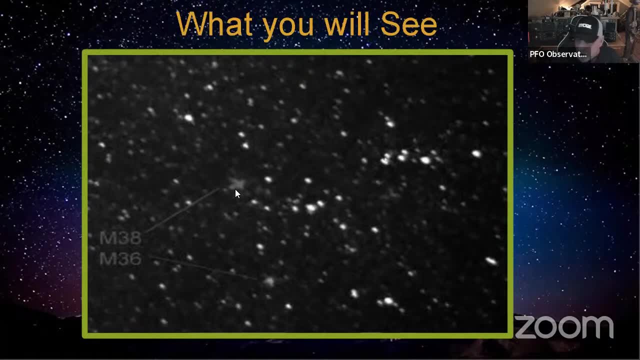 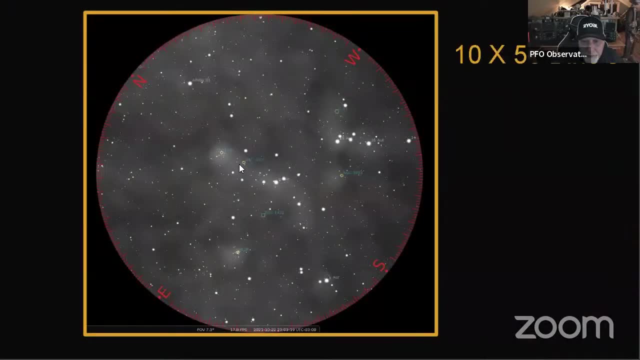 binoculars and if you look, get it in right spot. m38 almost looks like a mole on the side of a cheek. so there you go, in a pair of 10 by 50 binoculars. this is exactly your view. so there's the two eyes. 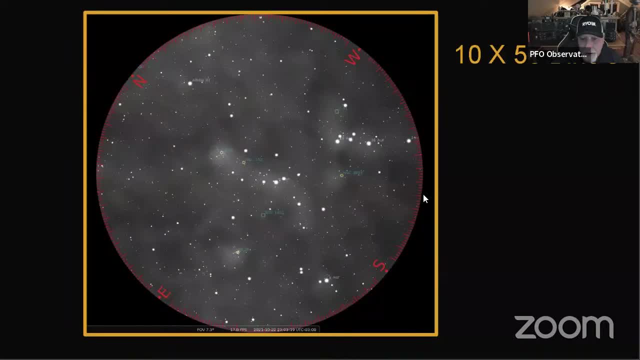 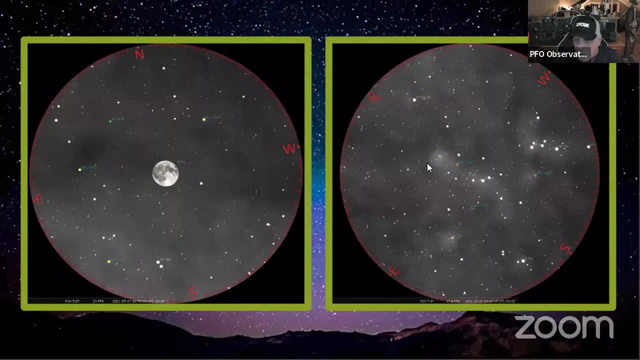 the big smiley mouth and, like i said, m38 makes a nice little mole on the cheek compared to the full moon. easily, easily two full moons, if not two and a half, maybe three full moons. so it's a very easy object to spot and when you get up in that area you'll know what the leaping 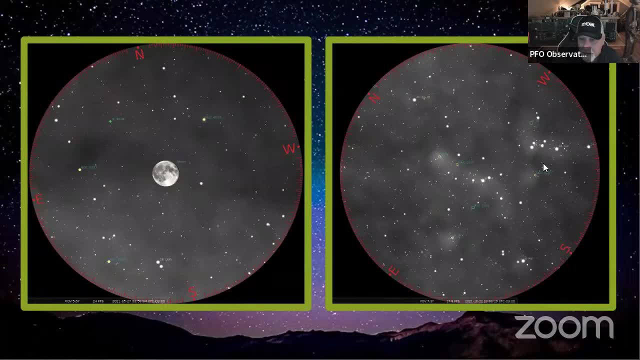 minnow. that's what i was talking about. it's right here off to the side, and the smiley face is actually part of the splash that the leaping minnow goes into. so not only going to get a smiley face, but you can eat the leaping minnow as well. 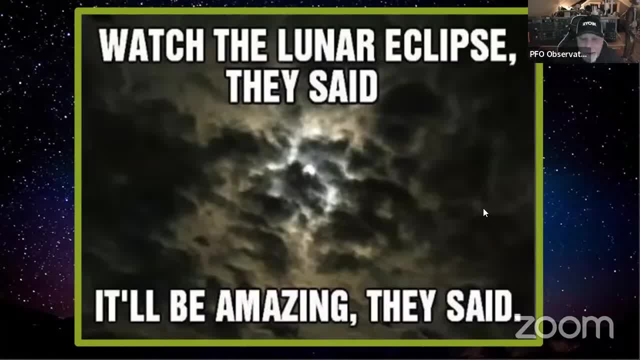 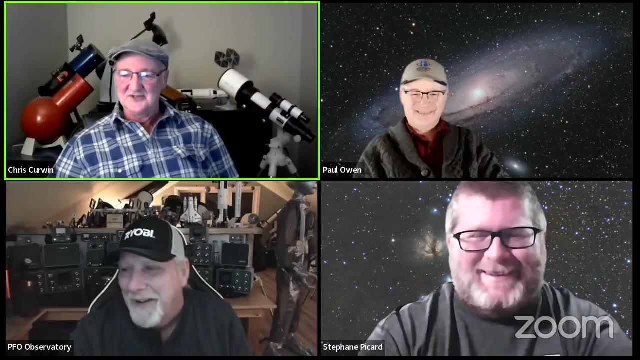 watch the lunar eclipse. i said it'll be amazing. i'm still hearing one there. this line was already done before your speech, so it wasn't. that's our final bun. that's no reflection on april the 8th. let's get no, no, no, no, you're indeed clear sky. 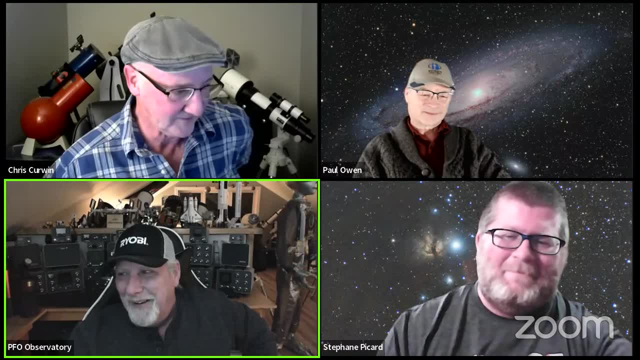 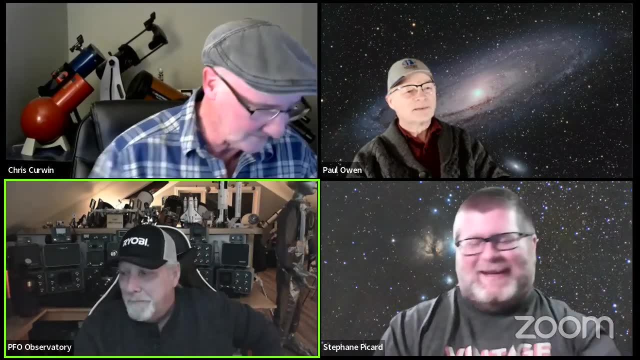 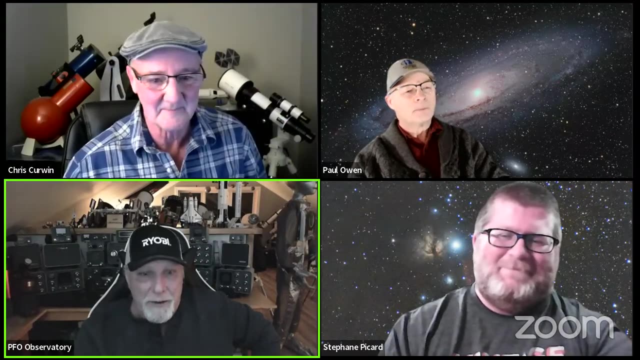 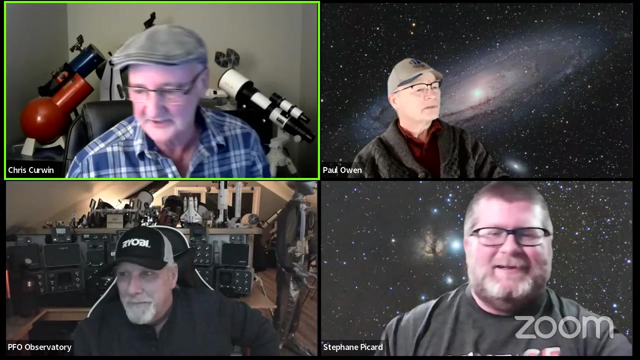 somewhere, somewhere, hopefully here. 99.9 chance here. yes, thanks, mike. keep our fingers crossed, there you go. that's the other professional astronomer. by no, bud, i don't want to remember. okay, and he combs his hair, true, okay, uh, we're running uh 903, but i guess we're gonna. well, we're about 10 minutes late starting, so 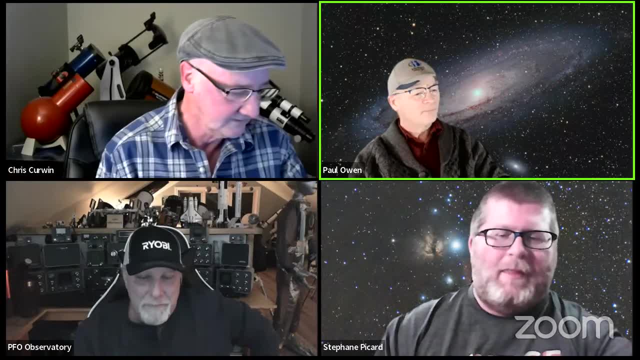 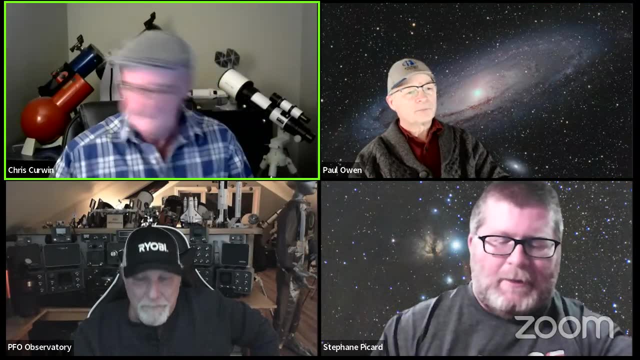 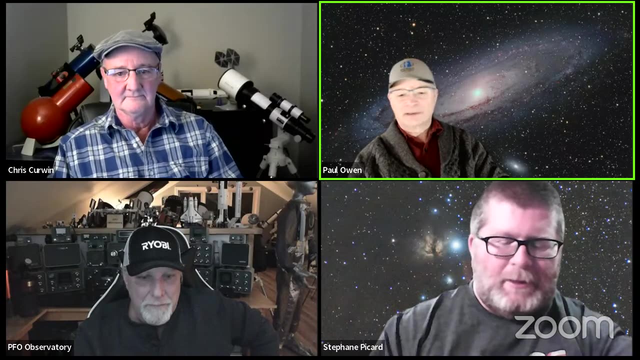 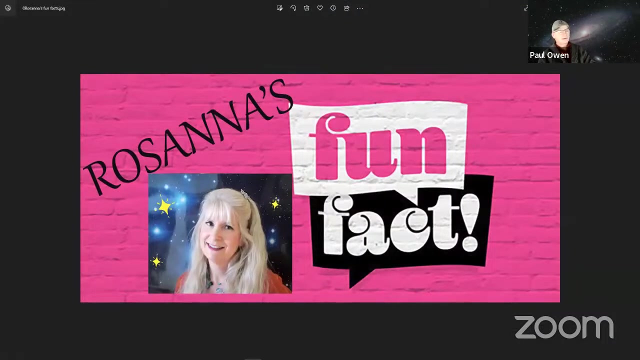 we'll continue. uh, paul, yeah, rosanna, yeah, okay, let's go. if everybody's okay, we'll continue on with the show a little bit longer, okay? so let me share my screen, share my screen, and this is going to be this week's rosanna's fun fact. 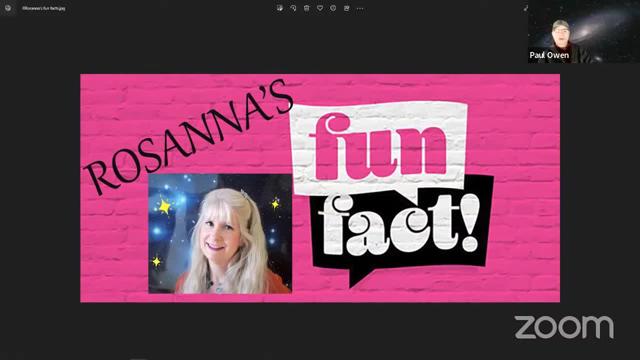 well, welcome back rosanna for another amazing fun fact, and i read this one today and this is: this is a really, really, as they all are very cool fun facts. let's get right into it. so rosanna writes: hi, paul, back in 2021. the signatures of the ghost particles: neutrinos. 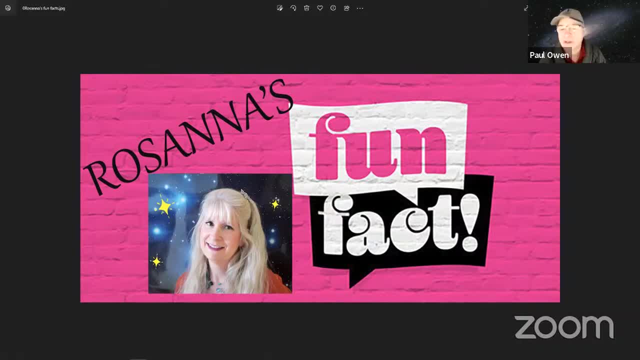 were tentatively spotted in a large hadron collider. just this past week, on march the 19th, physicists presented new results that neutrinos had actually been seen at the 57th uh, recontour's, demorand electro week interactions and unified thorium's conference in italy. now let me show you. 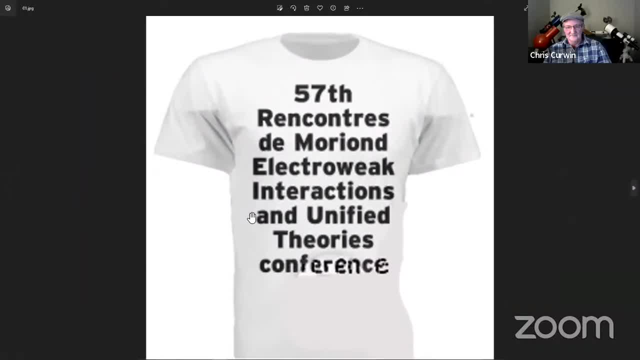 that t-shirt. you think you, you, you think i'm struggling, you read it, so back, so anyway. so yeah, that's what that is. wow, the conference souvenir t-shirt would be something to see, and no easy acronym either. that is unbelievable. the word, the word, scene is. 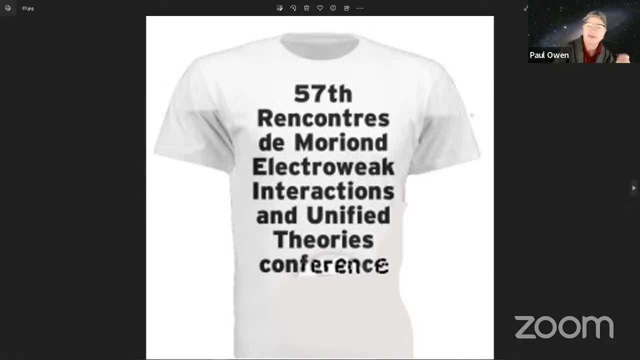 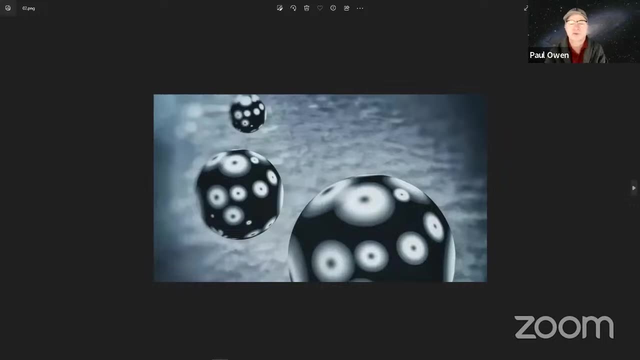 inaccurate, so as no one has actually seen the neutrino, just the evidence of it. but it, uh, but i guess it could look like this, and this is an artist's interpretation: the tiny particles were spotted by the phasor neutrino detector at the large hadron collider. 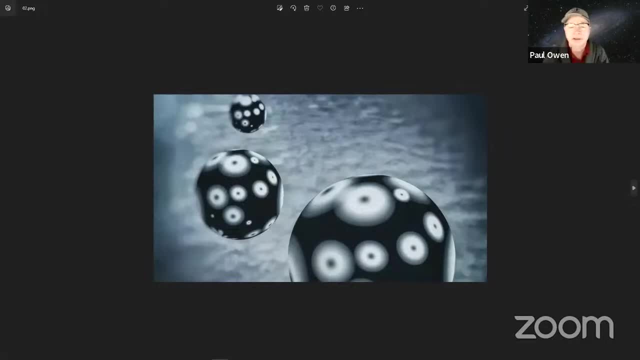 near geneva, switzerland, to catch the subatomic specters, the physicists built a particle detecting s'mores, dense metal plates of lead and tungsten, sandwiching multiple layers of light detecting gunk called emulsion. now, when high powered beams of protons smash together inside this l8c, they produce a shower of byproduct particles. a small fraction of 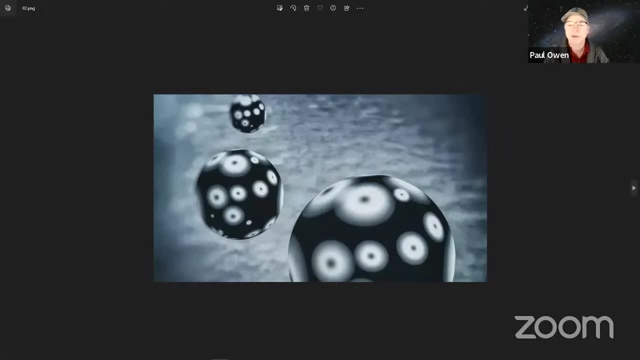 neutrinos that entered the small, the s'more, and the neutrinos from the from those from. these collisions then slam into an atomic nuclei nuclei and the dense metal plates and decay into other particles. the emulsion layers work in a similar way to old-fashioned photographic film. 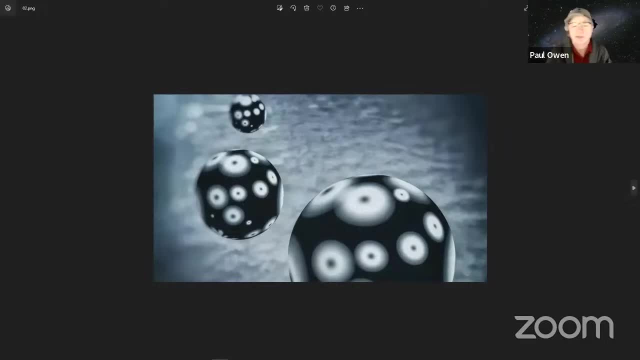 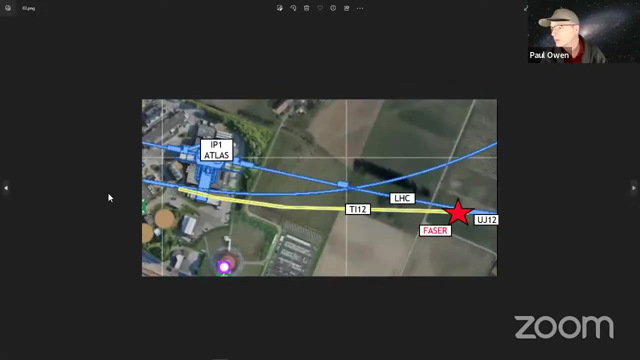 now in the industrial world. there are several other ways of interacting with neutrino byproducts: to imprint the traced outlines of the particles as they zip through them. amazingly, the whole 43 pages of the presentation are online available to all. i confess i did not understand the math or the 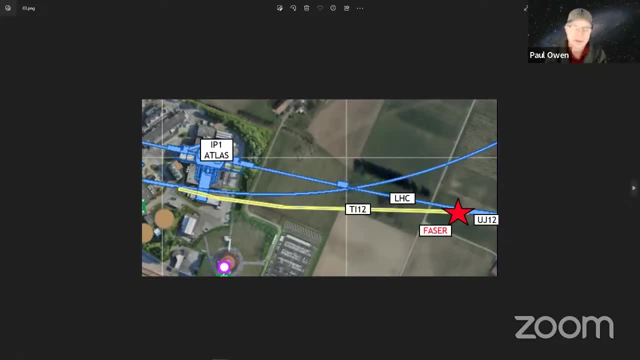 equations, so um. so one might ask: why is this significant? we've known about neutrinos for some phaser are not solar neutrinos, they are neutrinos that they created from smash ups. the study of these neutrinos- uh, the creation and the tracing of the scientists believe will eventually lead 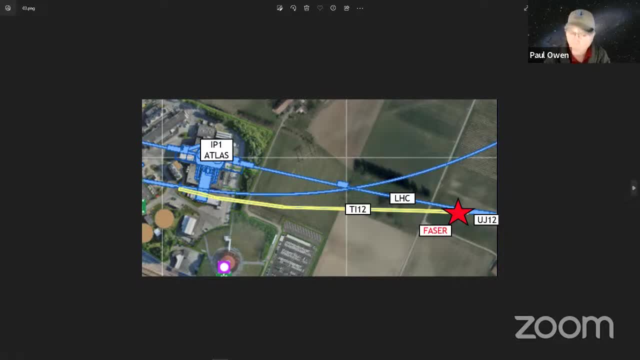 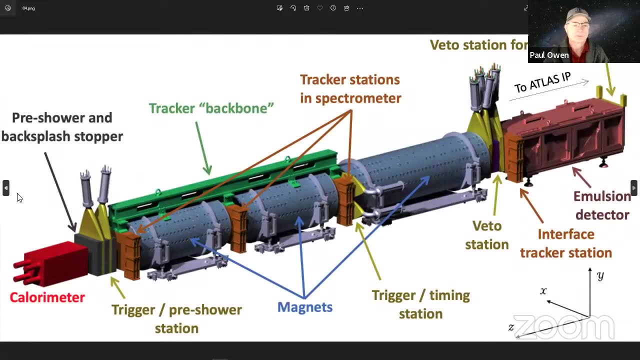 to understanding um the how and the why of stars exploding. so that's why they want to really look at these. look at these things: the heart of a nearby spiral galaxy, ngc 1068, researchers have found a thriving factory of neutrinos. researchers do not know why this massive amount of neutrinos. 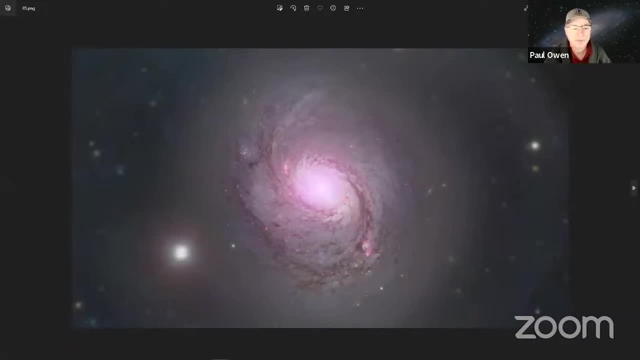 are being released. yet another mystery to solve. so every second, about 100 billion neutrinos pass through each square centimeter of your body. read that again: every second, about 100 billion neutrinos pass through each square centimeter of their body. the tiny particles are everywhere, produced in the nuclear fire of stars in enormous 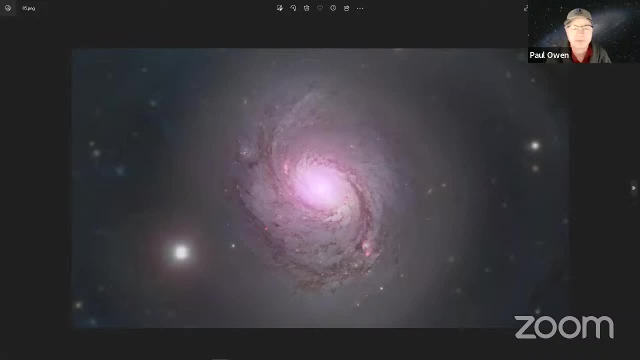 supernova, explosions by cosmic rays and radioactive decay, and in particle accelerators and nuclear reactors on earth. in fact, neutrinos, which were first discovered zipping out of a galaxy in 1956, are second only to photons as the most abundant subatomic particles in the universe. 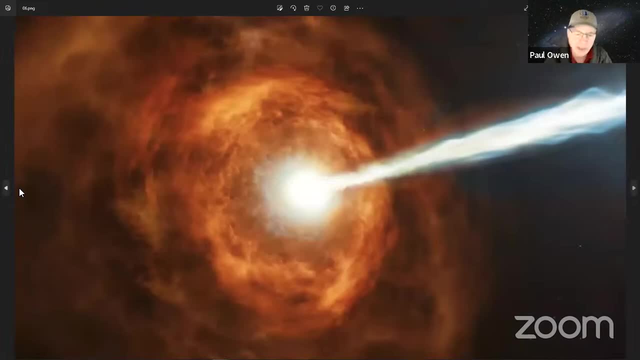 now here is another uh question researchers are asking: could gamma rays and high energy neutrinos come from the same intergalactic sources? not surprisingly, but in an effort to answer this and so many other questions concerning neutrinos, china is in the process of building a detective. 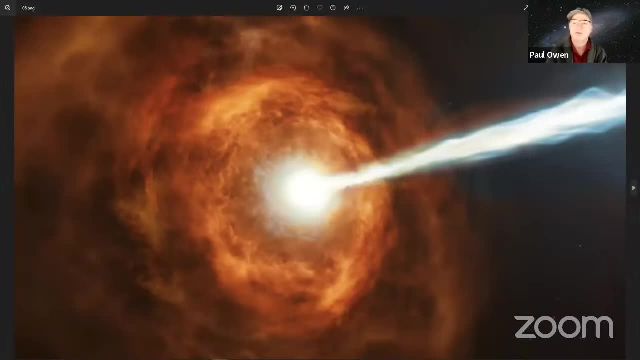 deep beneath the ocean surface to hunt for the elusive sub-atomic particle. although every second, tens of trillions of neutrinos stream through earth without interacting with anything, occasionally one of these neutrally neutrally charged particles will collide with a stray atom's nucleus, emitting a nearly undetectable spark of light. this spark of light helps scientists determine not only: 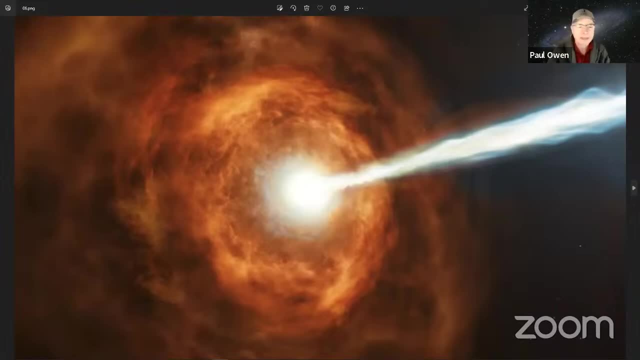 neutrino was there, but also identify where it might be or where it might have originated. This is absolutely amazing, as even the decaying potassium with a banana can create neutrinos. So did the latest neutrino come from a banana or a black hole? 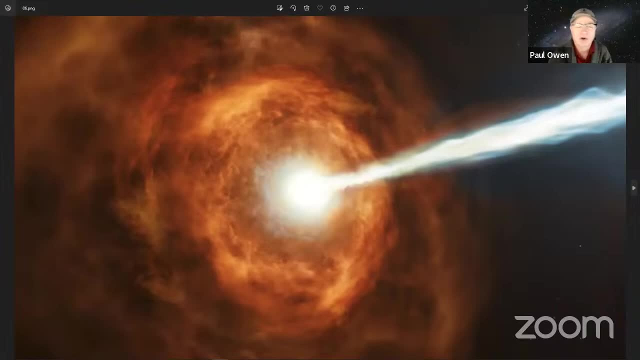 That's a bit mind blowing when you think about it. It rather makes all of China's alleged TikTok tracking of keystrokes fade into the background. Scientists have had to build neutrino detectors in areas with large amount of transparent materials in order to be a better spot. unpredictable flashes of light that reveal a neutrino. 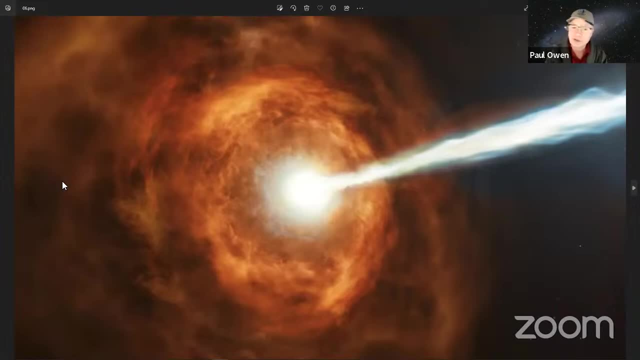 Existing detectors include the National Science Foundation Ice Cube Neutrino Observatory in Antarctica, which covers around 0.2 cubic miles, or one cubic kilometer, with 5,160 sensors, nearly a mile under the ice. Down there, the ice is clear enough that the sensors can pick up any tiny flashes of 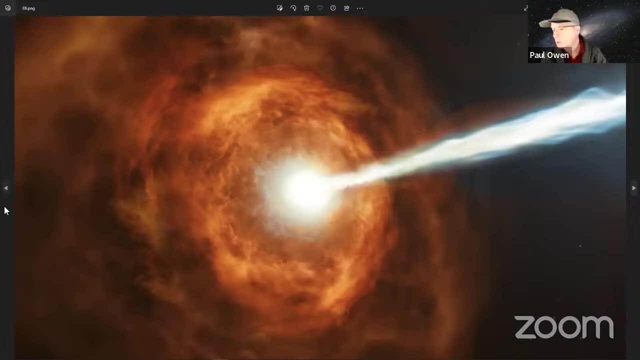 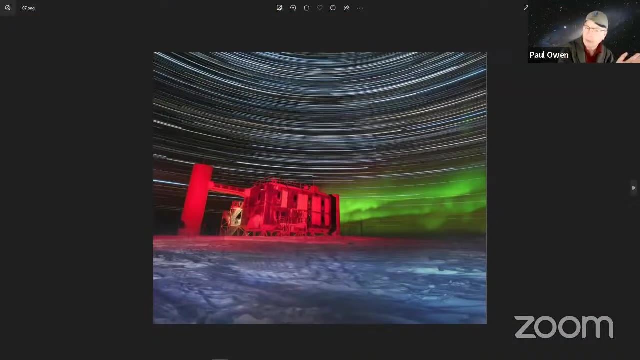 light. I love this picture of the Ice Cube Observatory. Now I don't know if you can see that or not. Yes, you can. There it is The Ice Cube Lake at the South Pole, lit up by star trails. is the photo taken in July? 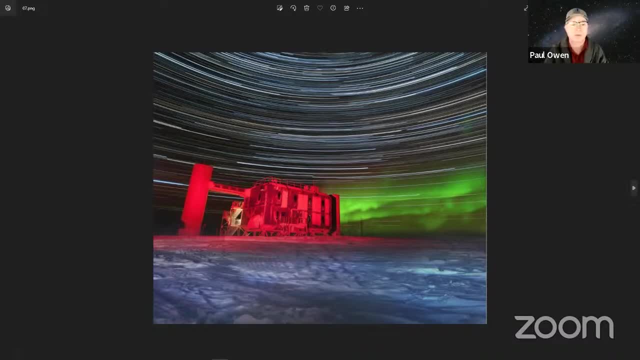 2015,. and the image credit goes to Ice Cube Collaboration. China's new detector will be built with 55,000 sensors. It will be suspended 0.6 miles or one kilometer beneath the ocean's surface, and the sun rays can't travel that deep, which will help the sensors detect neutrinos and distinguish. 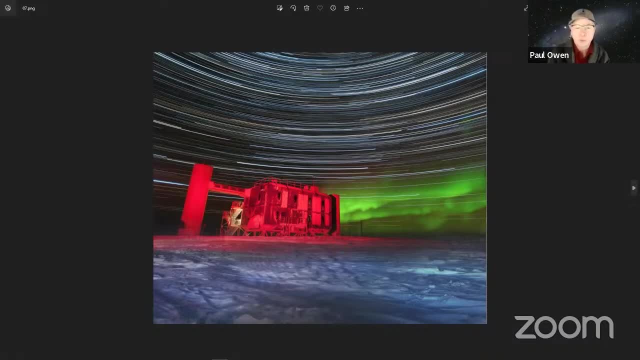 them from solar neutrinos. This will not be the only underwater detector. Russia is building the Baikal Gigaton Volume Detector in Siberia's Lake Baikal, the world's deepest lake. So then there's the upcoming European Cubic Kilometer Neutrino Telescope, a multi-institution. 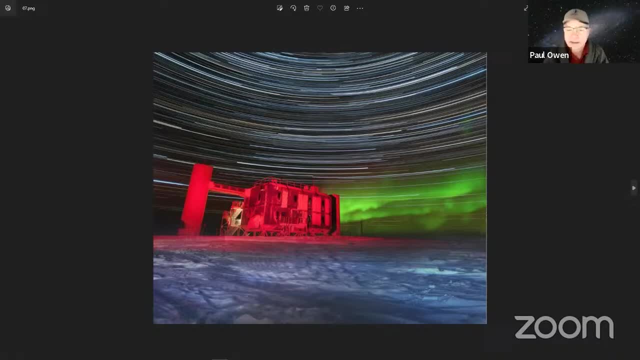 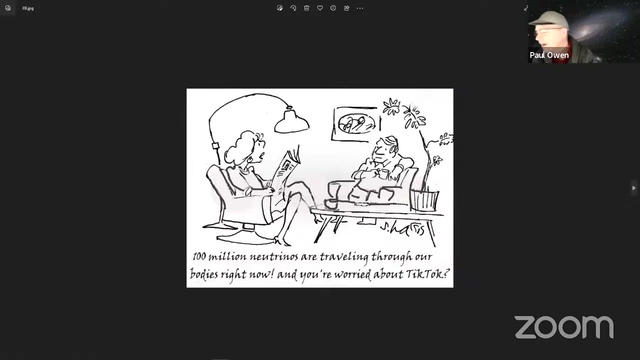 collaboration that will hunt for neutrinos in the Mediterranean. There's also a Pacific Ocean Neutrino Experiment, another multi-institutional collaboration working on a detector in the Pacific Ocean off the coast of British Columbia, Canada, Thank you. So a bit of international race is on and to find the untracked neutrinos. 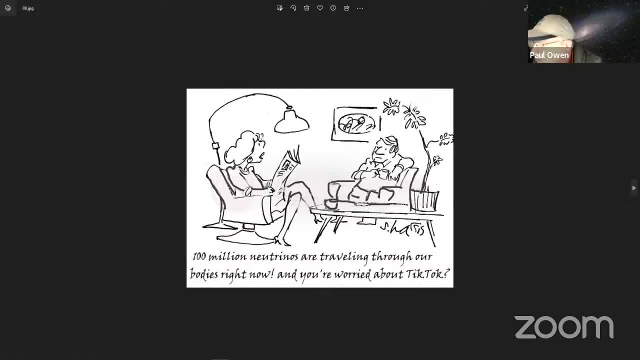 So these two are sitting there and she's reading the paper and she says: well, a hundred million neutrinos are traveling through our bodies right now and you're worried about TikTok? Oh my gosh, that is just too funny. 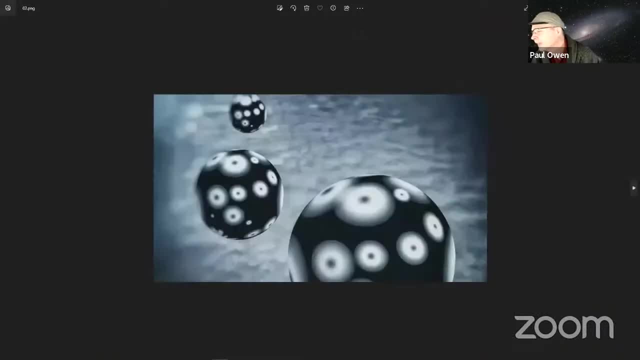 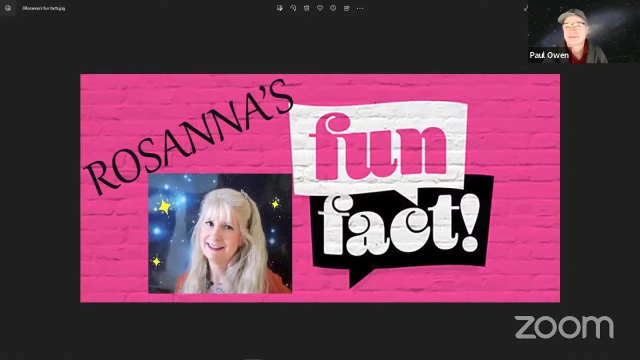 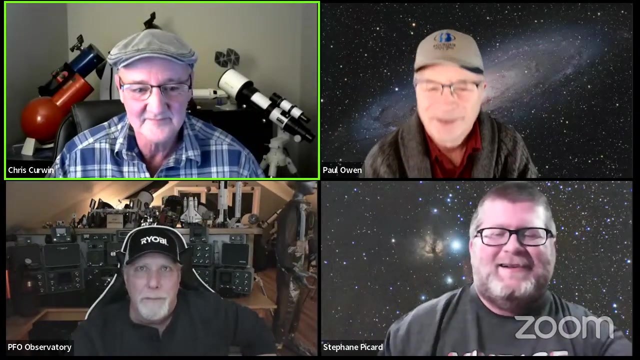 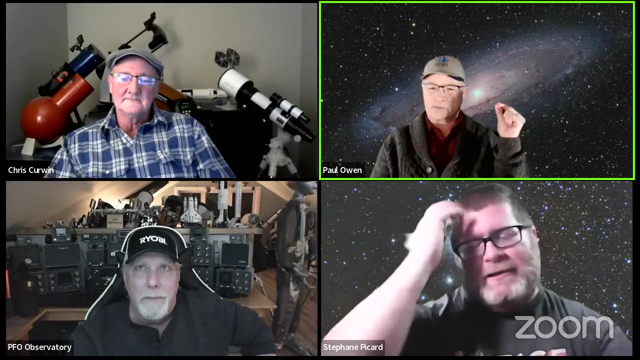 And let me see if I can get back to that. And that was this week's Rosanna's Fun Fact: Neutrinos, neutrinos, neutrinos. What they're thinking is they're connecting that with star explosions. So look at the vastness and the size of those two things. 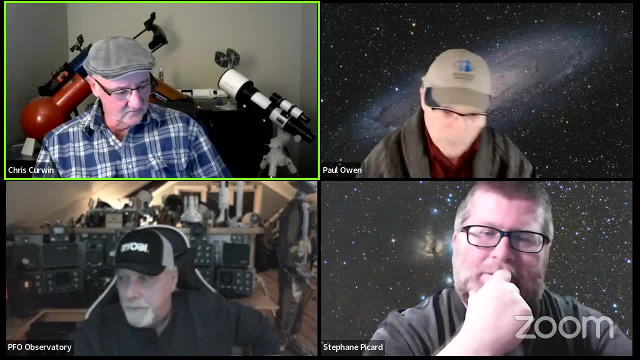 I was reading recently that with Betelgeuse, the fact that it's going to be, you know, a new device, Yeah, It's going supernova at some time. You say, well, when is it going to go supernova? 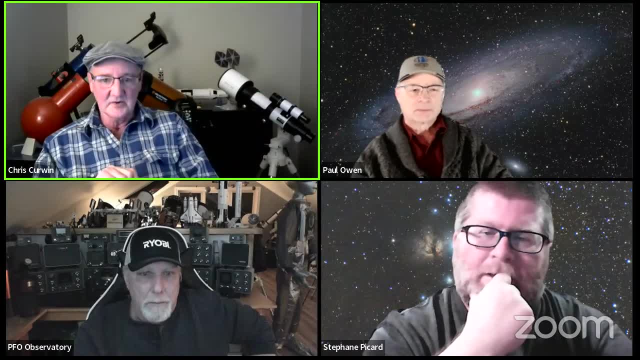 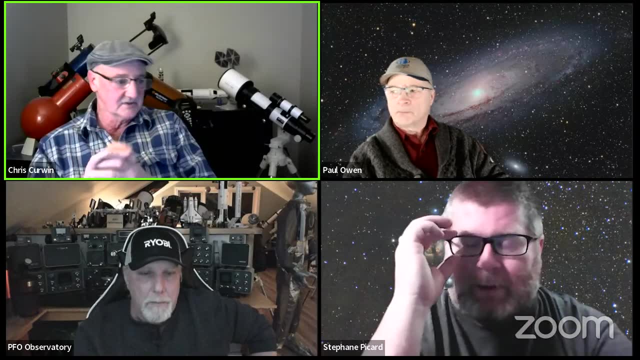 We don't know. Well, one of the things that they're going to be looking at is neutrinos. The increase in neutrinos will give them a sign that it's actually happening. I know we, just a year or so ago, they talked about. they thought that it was happening. 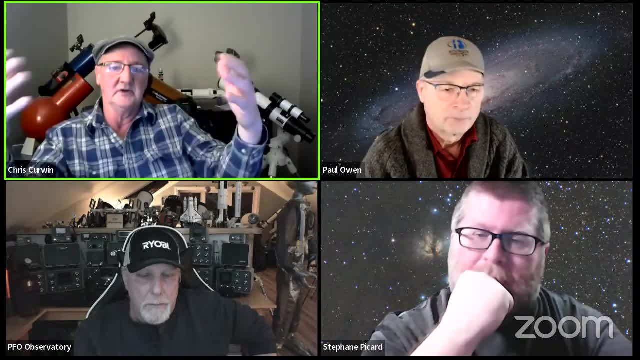 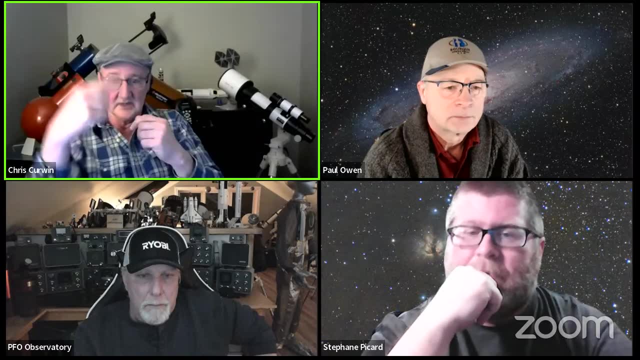 because they saw Betelgeuse dimming and brightening, and dimming and brightening, and it was more. what they believe now was that it was off-gassing, it was giving away material in space And, from our point of view looking at Betelgeuse, we were losing. 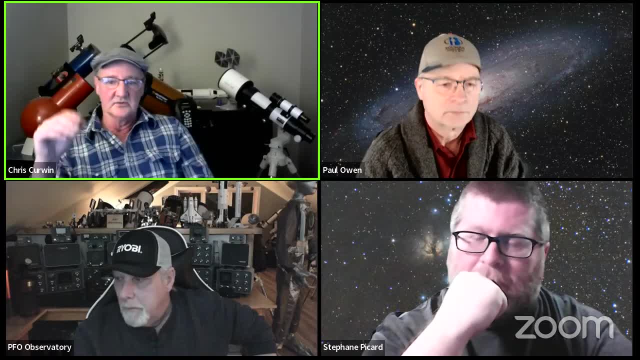 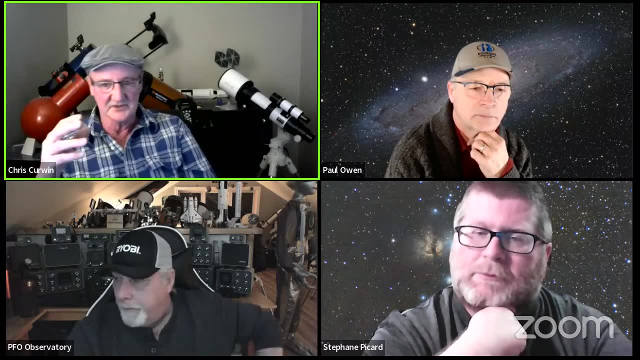 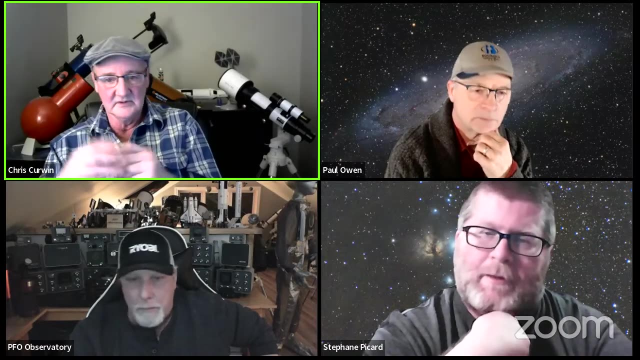 We were losing our view and then gaining it again, And so it was pulsating, basically releasing large amounts of material, but it wasn't increasing the amount of neutrinos, apparently. So that's what we're going to be watching for when we see the ultimate demise of Orion. 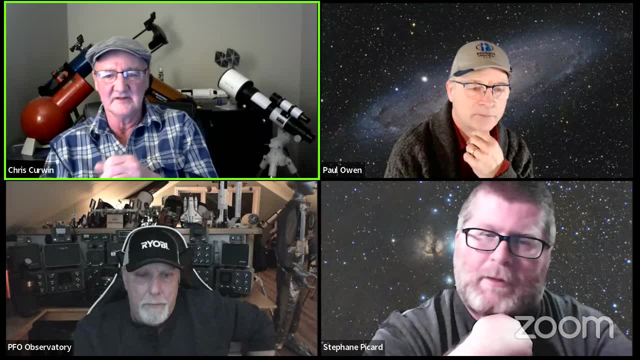 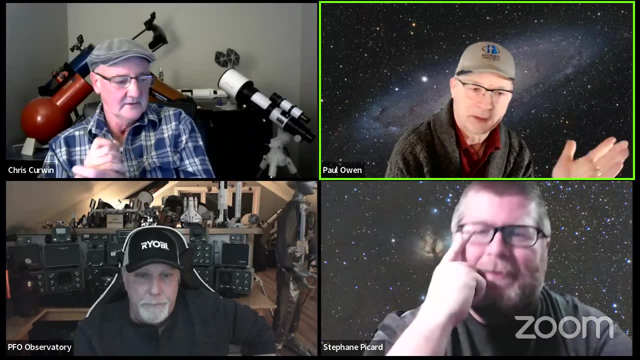 of Betelgeuse. Yeah, So they're fascinating things. a hundred billion of them in every centimeter, wasn't it? Every square centimeter, A hundred billion pass through your body, Unbelievable. They have to, They have to. 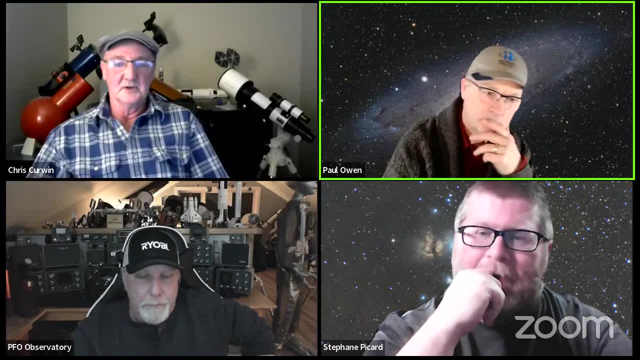 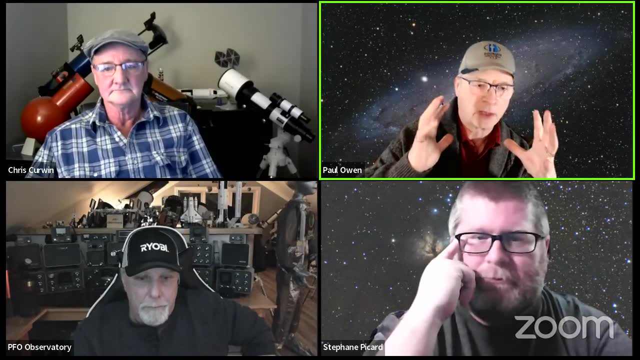 They have to collide with something in order to spark, So they have to have detectors below ground or below It's going to be, and because it's such a small bit of light, it has to be virtually dark, Yeah, Yeah, And then with photons, 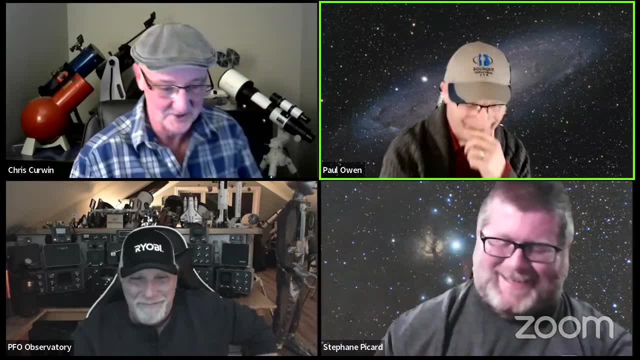 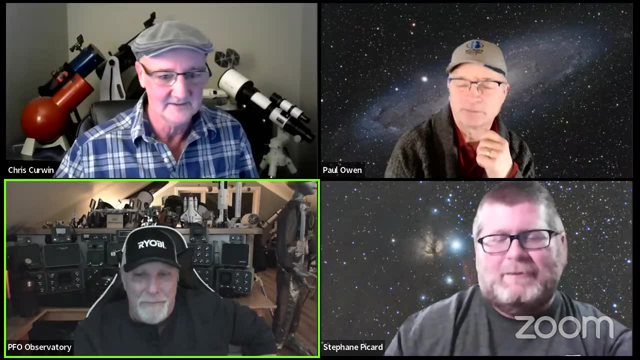 Hey, Mike photons, We were talking about them earlier. Hey, pretty cool, Thanks. Thank you, Rosanna, for another interesting talk. Absolutely, Yeah, Bobak, Awesome, Okay, Let's go from there. Yeah, Yeah. 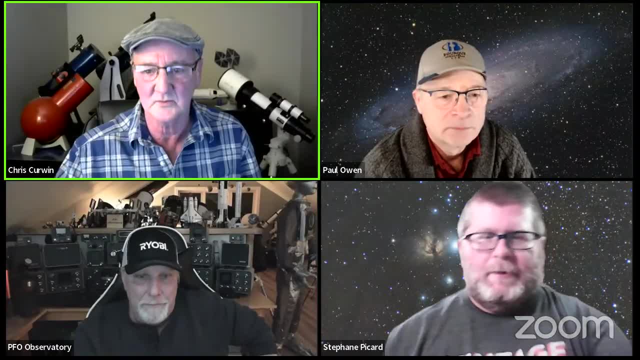 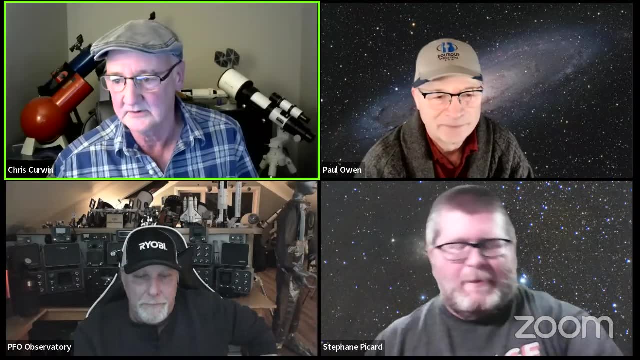 Yeah, So I'll go from there then to a quick what's up talk, What's up, talk, What up? Okay, We should be up here soon Now we're going to go through this pretty quickly because we have some photos to go. 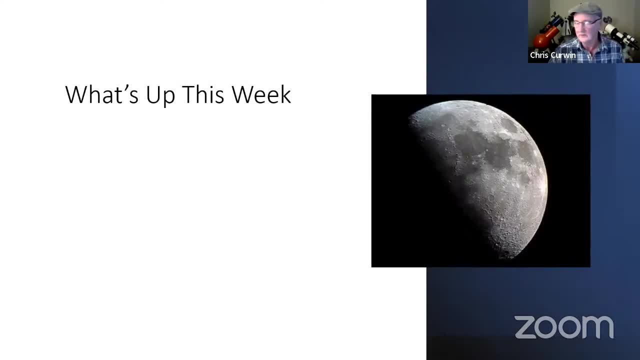 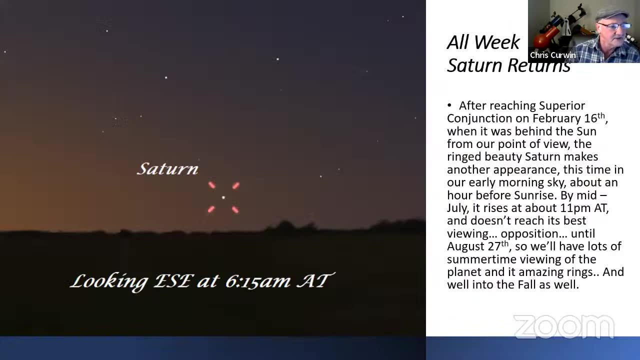 and then quickly through our closing. Okay, What's up this week? Let's take a look. Well, all week long, Saturn returns- actually, after reaching superior conjunction on February 16th. behind the sun, from our point of view, the ring beauty saturn makes it another appearance. now. 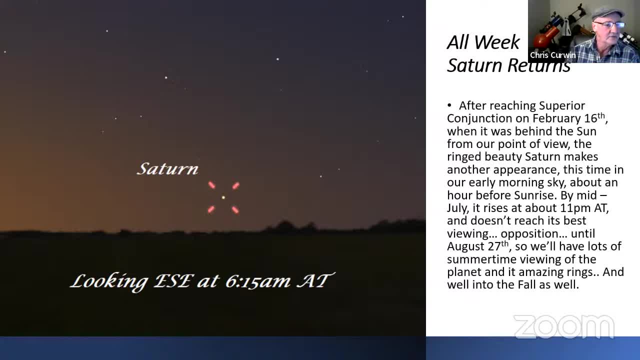 this time in our early morning sky, about an hour before sunrise. now by mid-july it rises at about 11 pm atlantic time. it doesn't reach its best viewing or opposition until august, the 27th, so we'll have lots of summertime viewing of the planet and its amazing rings, and well into the. 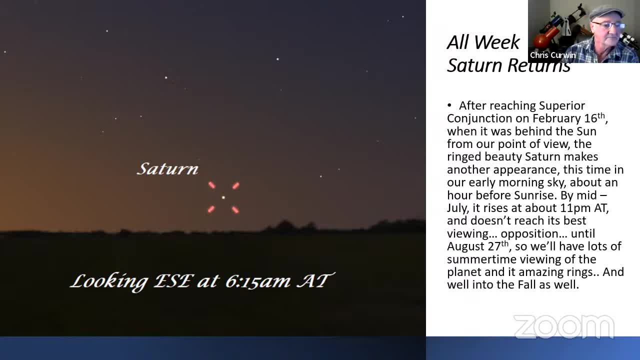 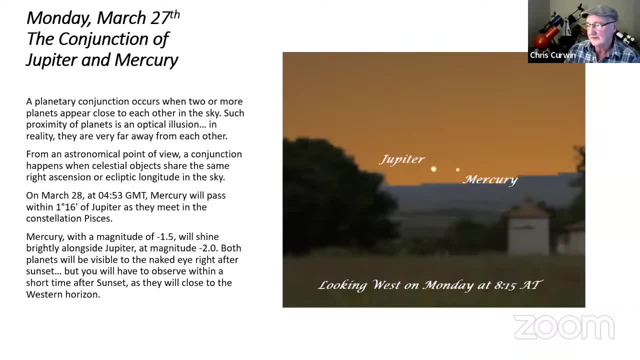 fall as well. so hooray for saturn. we all love saturn, one of them, one of the one of the wow elements at the telescope, for sure. yeah, peace, uh. monday, march 27th, uh, the conjunction of jupiter and mercury, now planetary conjunction, occurs when two or more planets appear close to each other in 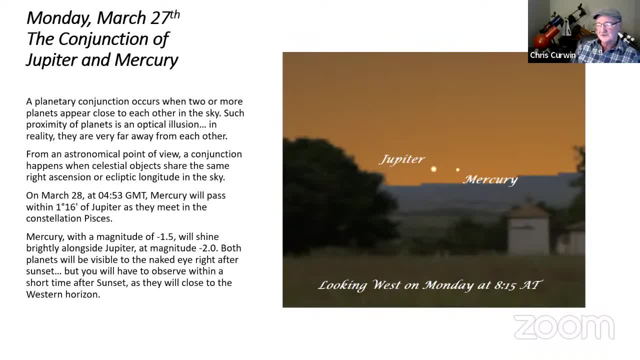 the sky. such proximity of planets is an optical illusion, of course. in reality, they are very far away from each other: jupiter, mercury, for example. from an astronomical point of view, a conjunction happens when celestial objects share the same relationship with each other, and the conjunction happens when celestial objects share the same. 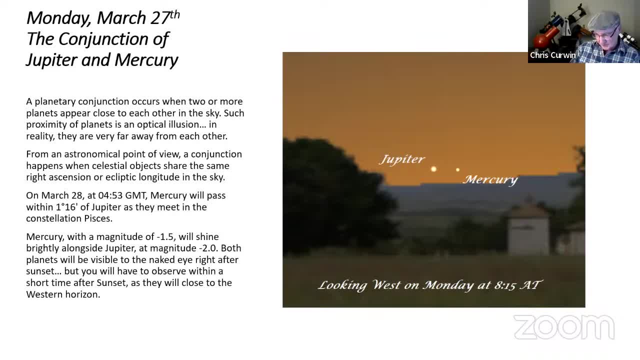 relationship with each other and the conjunction happens when celestial objects share the same ascension or clip or ecliptic long longitude in the sky. on march the 28th, at 4: 33 gmt. uh mercury will pass within 1 degree and 16 arc seconds of jupiter as they meet in the constellation of. 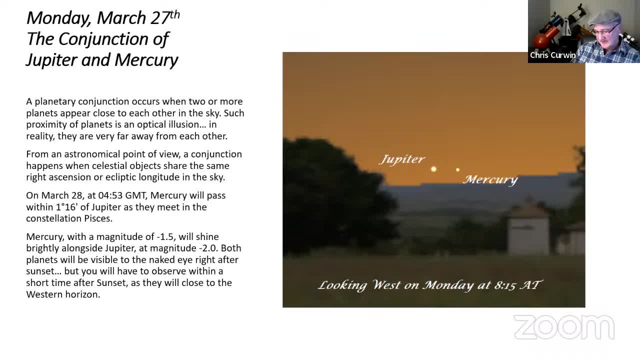 pisces. mercury with magnitude of minus 1.5 will shine brightly alongside jupiter at magnitude minus 2.0. both planets will be visible to naked eye right after sunset, but you'll have to observe within a short time after sunset, as it will be visible to naked eye right after sunset. 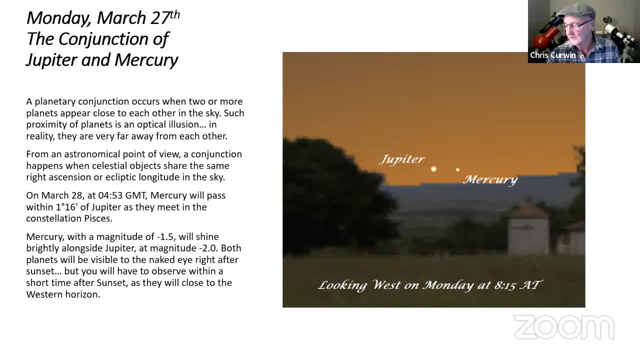 both planets will be visible to naked eye right after sunset, but you'll have to observe closing uh on the western horizon very quickly. so, uh, nice view. um, mercury should start. mercury will be climbing in our evening sky. actually, jupiter is going to get settling close to the horizon. 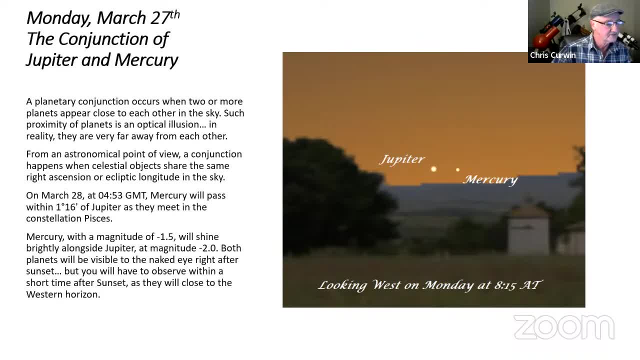 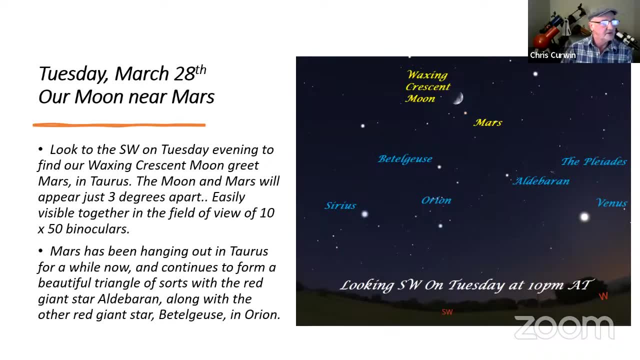 closer and closer every day now, uh, as it disappears for a little while on tuesday, uh, our moon near mars. uh, look to the southwest on tuesday evening to find a waxing crescent moon. greet mars and taurus. the moon and mars will be appear just three degrees apart, easily visible together in the field of. 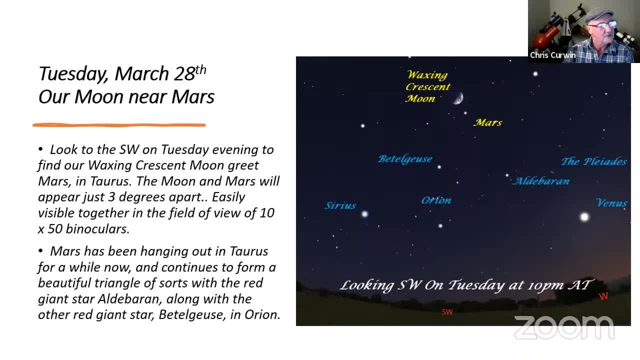 view of 10 by 50 panoptres. mars has been hanging around in taurus for quite a while now and continues to form a beautiful triangle of sorts with red giant star aldebaran and uh in taurus, along with the other red giant star, betelgeuse and orion, so keep an eye out for that on wednesday. 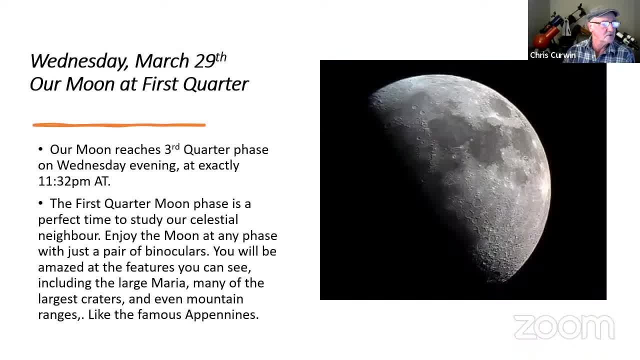 march 29th. our moon is at first quarter. it reaches a third quarter. first should be first quarter phase, not third quarter phase. on wednesday evening at exactly 11: 32 pm, the first quarter moon phase is a perfect time to study our celestial neighbor. enjoy the moon at any phase, really with just a 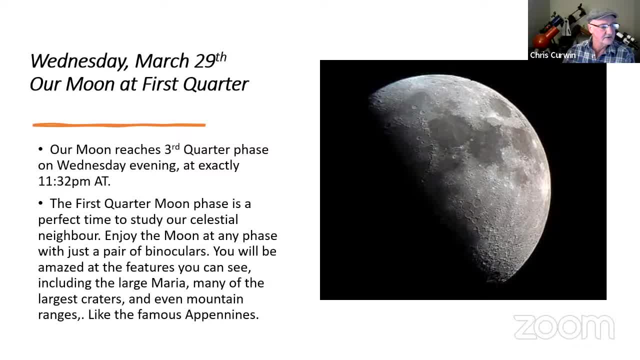 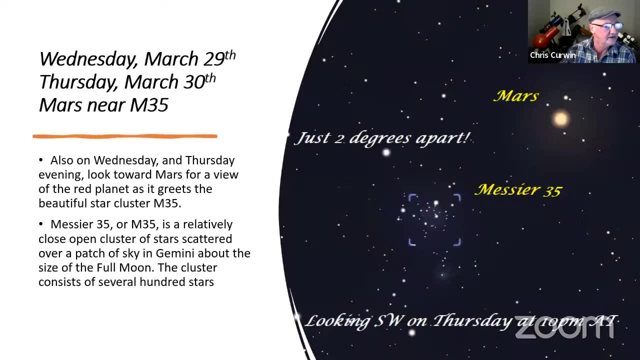 pair of binoculars, you'll be amazed at the features you can see, including the large maria, which are these large dark facets that we see on the moon here, many of the larger craters and even mountain ranges, like the famous apennines, right here on wednesday, march 29th as well, and even thursday, 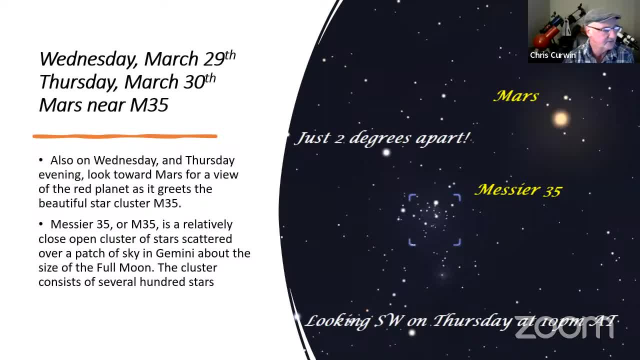 march 30th, mars will be near messier 35 or m35 um. look towards mars for a view of the red planet as it greets the beautiful star cluster and messier 35. messier 35 or m35 is a relatively close, open star cluster. 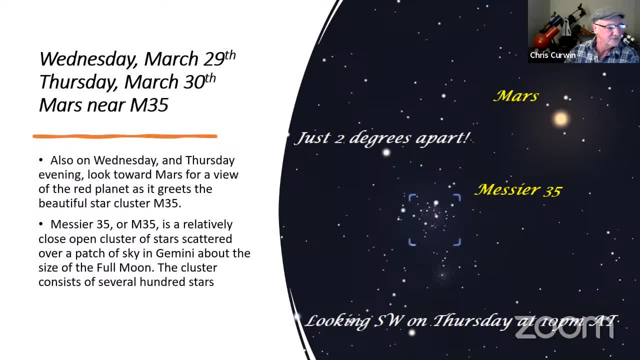 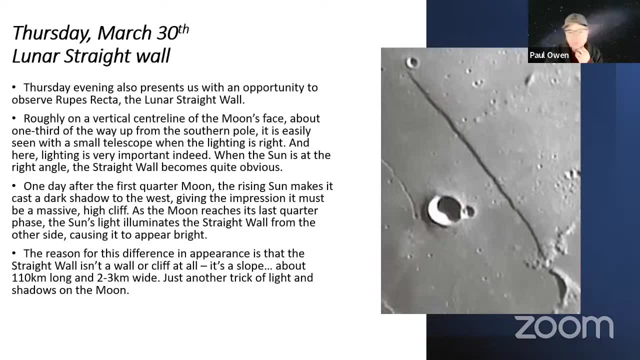 scattered over a patch of sky and gemini about the size of the full moon on. the cluster consists of several hundred stars. always pretty in the doctors, for sure for small scope. uh, also thursday, the lunar straight wall. thursday evening also presents us with an opportunity to see the moon and the stars of the moon. and the stars of the moon. 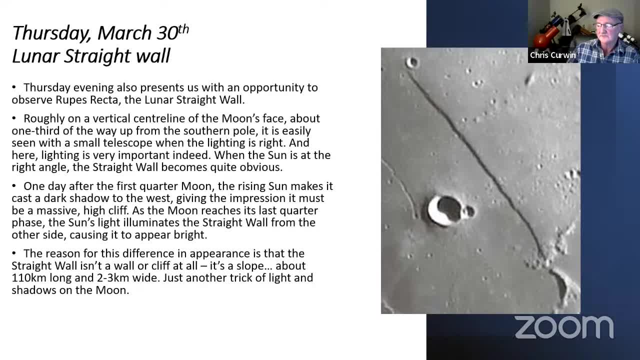 to observe rupes recta, the lunar straight wall, roughly on a vertical center line of the moon's face, about one-third of the way up from the southern pole. it is easily seen with small telescopes when the lighting is just right, and here lighting is very important indeed. when the 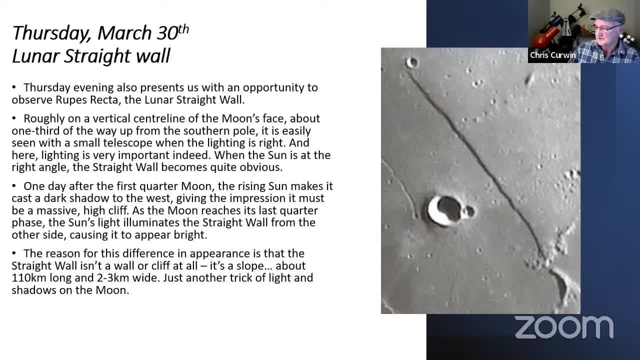 sun is at the right angle, the straight wall becomes quite obvious, almost looks like a cliff. one day after the first quarter moon, the rising sun makes- uh, makes it cast a dark shadow to the west, giving the impression it must be a massive high cliff as the moon reaches its last point in the 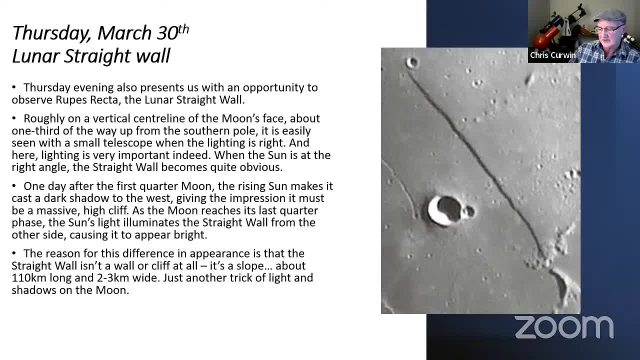 last quarter phase, though, the sunlight illuminates the straight wall from the other side, causing it to appear bright. now, the reason for this difference is in appearance is that the straight wall isn't a wall at all or a cliff. it's actually just a slope about 110 kilometers long and about two to three. 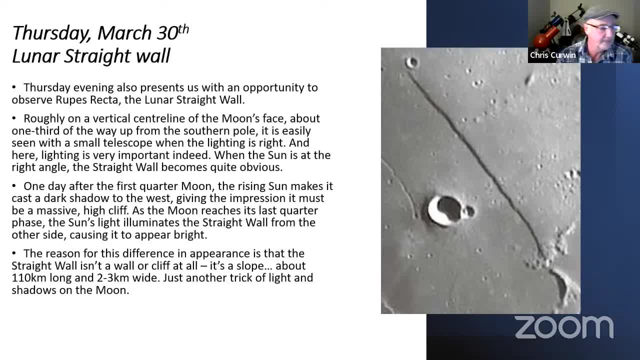 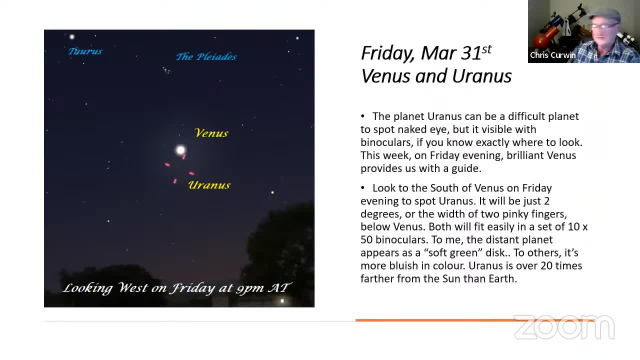 kilometers wide. just another trip of light and shadows on the moon, which happens quite often, especially around the line we call the terminator on friday evening. venus and uranus. planet uranus can be a difficult planet to spot naked eye, but it's a very difficult planet to spot naked eye. 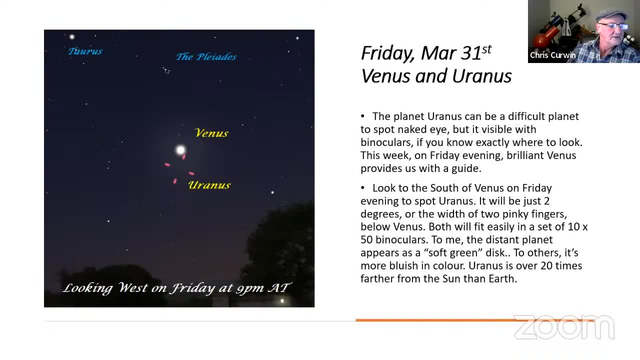 is visible with binoculars. if you know exactly where to look now this week, on friday evening, brilliant venus provides us with a nice guide. look to the south of venus on friday evening to spot uranus. that will be just two degrees, or the width of two pinky fingers, below venus. both will 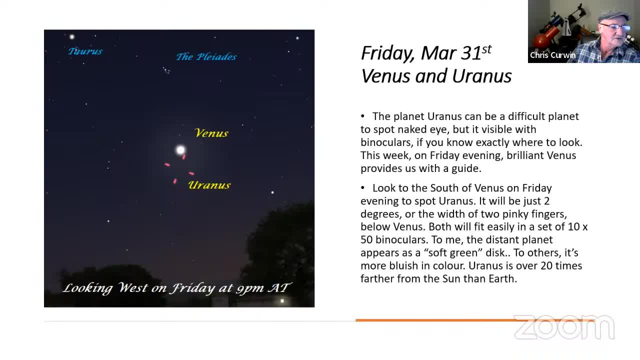 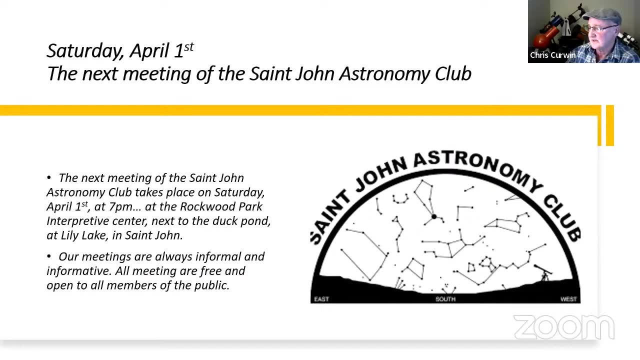 fit easily in a set of 10 by 50 binoculars. again to me, the distant planet appears as a soft green disc. to others it's more bluish in color. uranus is over 20 times farther from the sun than earth is, so it's nice to be able to catch it when you can. next saturday, next meeting of the saint john. 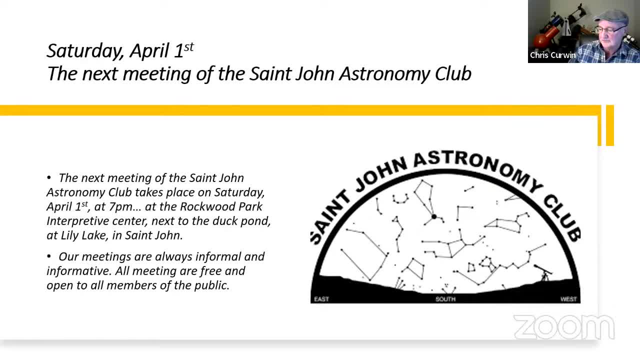 astronomy club. next meeting of the saint john astronomy club takes place on saturday, april 1st, at 7 pm at the rocket park interpretive center, which is next to the duck pond at lily lake in saint john. our meetings are always informal and also informative. all meetings are free and they're 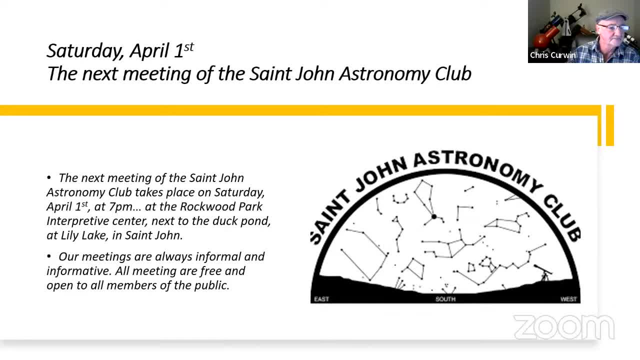 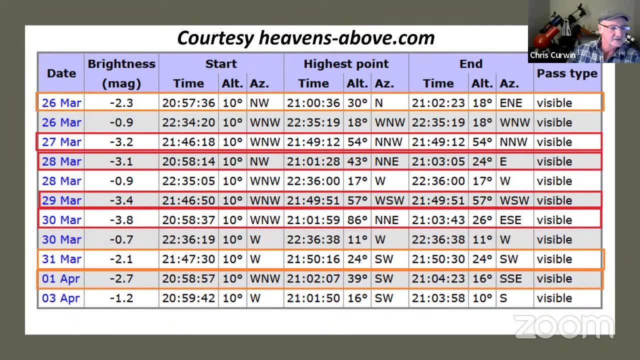 open to all members of the public, so come and join us. um, this chart comes from heavensabovecom. this is the chart for the iss, the international space station that passes over our area quite regularly. this is the evening passes for the next week. um, the ones that are in orange here are the ones that are fairly bright: minus 2.3. 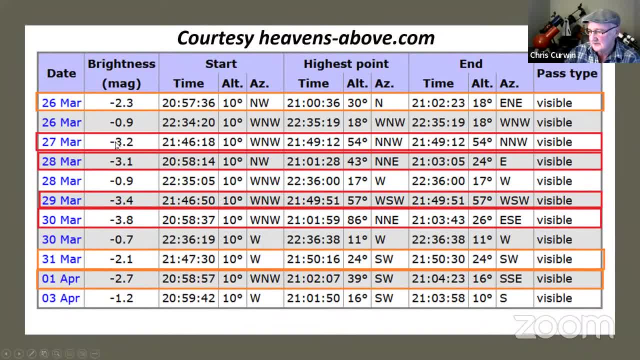 is fairly bright. ones with the red are the brightest ones passes. so we've got a nice pass. actually tonight there was one at 8: 57, um, then there's been a couple. we've got a pass tomorrow night, a couple on tuesday night, wednesday, thursday, right through the week. so, and here's the typical, 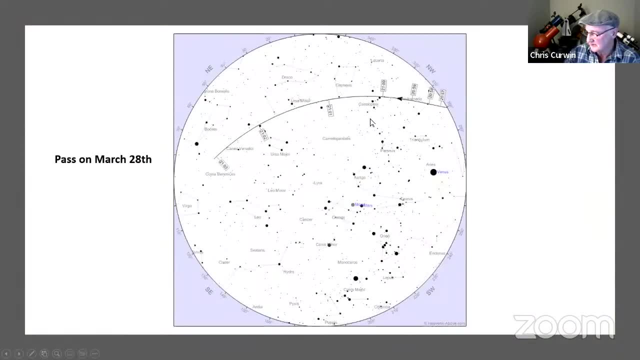 um, the 29th, i believe, right here, a passive minus march 28th. so there's the pass of march 28th. so if you've never seen it, it is pretty interesting to watch. this one's going to go right through cassiopeia, down through the handle of the big dipper, and you won't see quite all the way to. 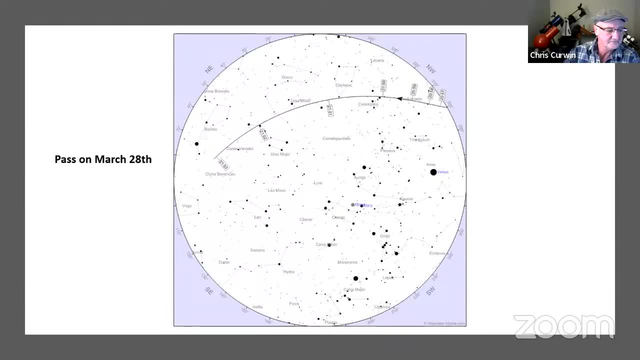 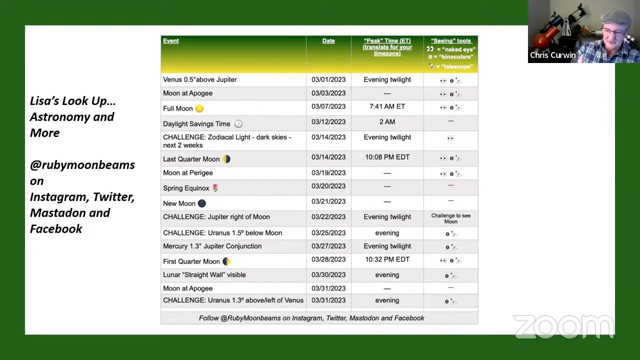 the horizon, but it's still be fairly bright, so quite easy to spot. um, i always refer to this chart. this is a chart from march. i'm waiting for the one from lisa from april. i know it's coming pretty soon. she's going to send it right along. so, uh, this is uh, at least his look up astronomy and 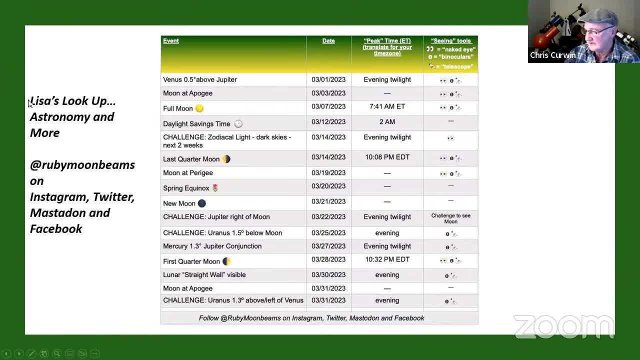 she gives us this chart every month, um, and it provides us with the event that's happening, the date of the event um, the peak time for viewing it and also your scene tools. do you naked eye the doctors or a telescope? you can find lisa's look up at uh ruby moonbeams on astronomy. 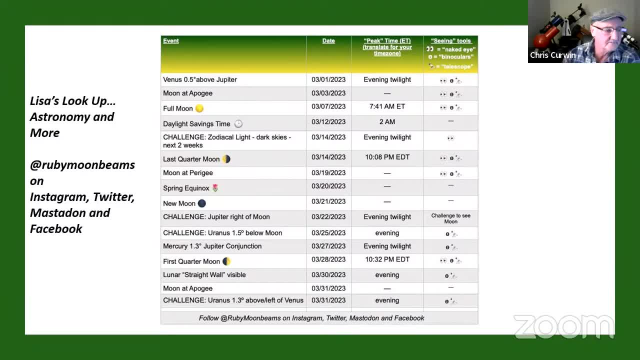 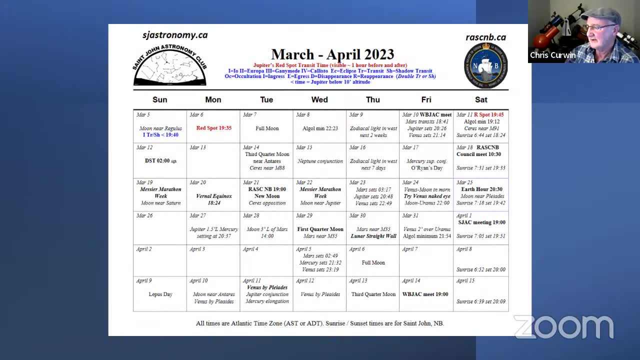 right, i'm sorry- on instagram, twitter, mastodon, facebook- thank you, lisa. and finally, our uh st john astronomy club rask nb calendar was just put up by our veteran kurt nason, with his calendar together for us every uh, every month, and this is actually a six-week calendar and that it lists. 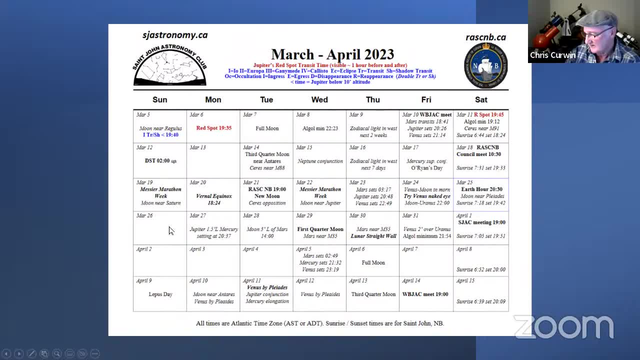 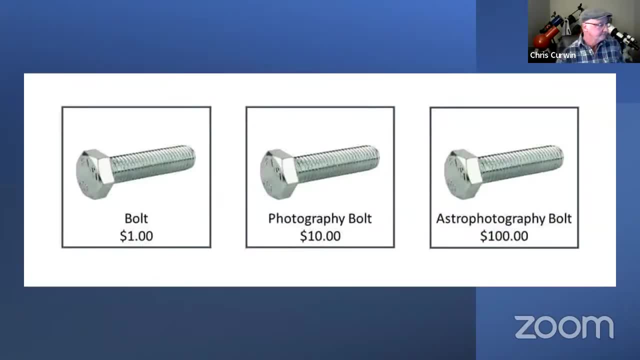 all of the others that are happening throughout the week. so if anything that's uh, any importance at all, it's going to be listed here in the week in the calendar. so that's what we see for, uh, this week coming up. yeah, that's so true, that's what it is. 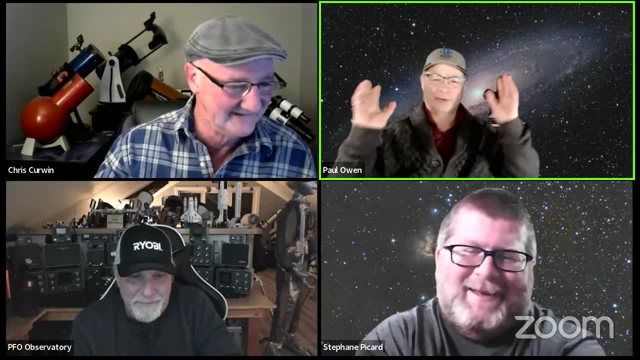 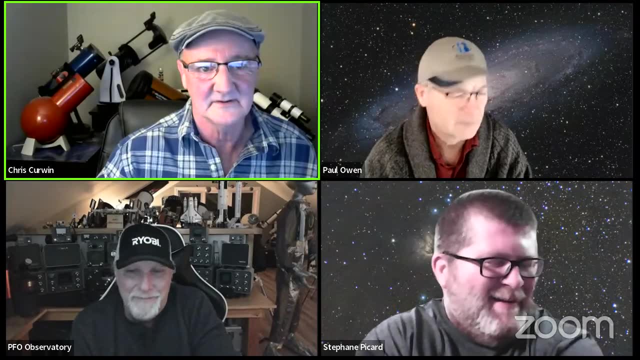 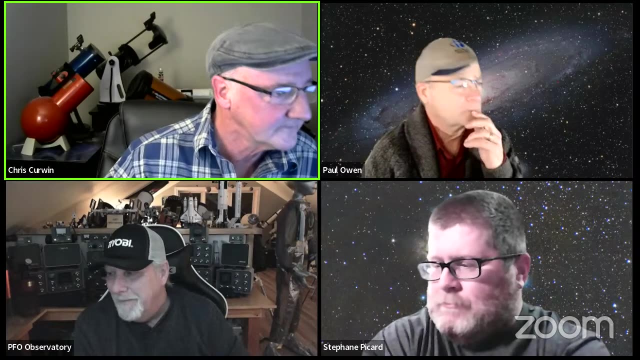 that's where we have mike guyver. you can get all those myths. okay, i'm going to go quickly through some photos that were sent in. um, give me a second here, bring this over to. i want it again. i need to second to set things up, play some music in the background, whatever you like. 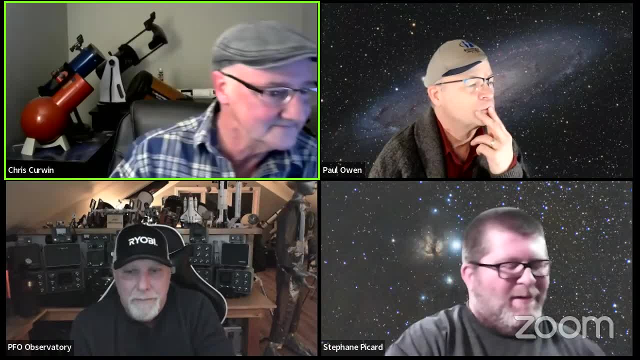 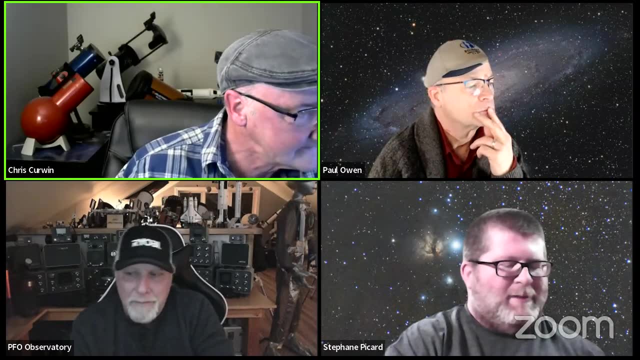 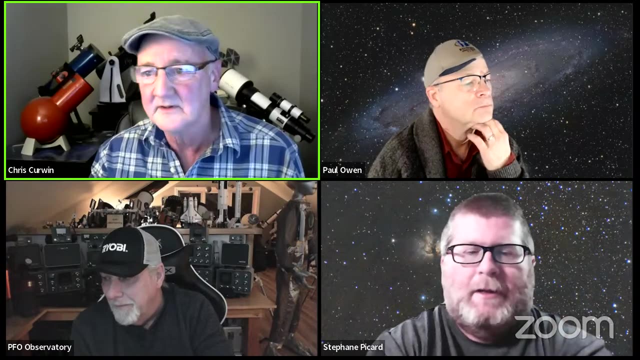 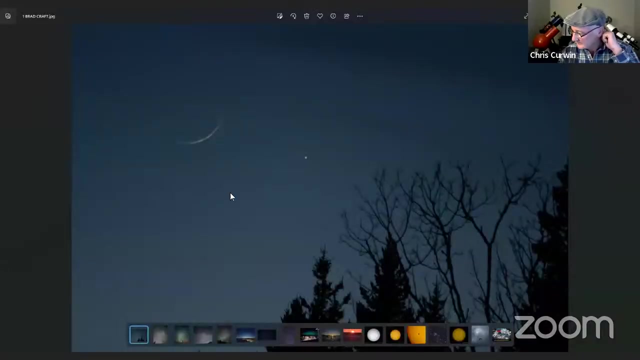 all right, always happens. okay, i just need to get my notes going here now real set. okay, let's get started with uh. i'll share my screen once more. i'm gonna share uh one. that's one there. yeah, there we go here, sir, nice, yeah, so uh, this one comes from brad graft. brad says: hi, chris i. 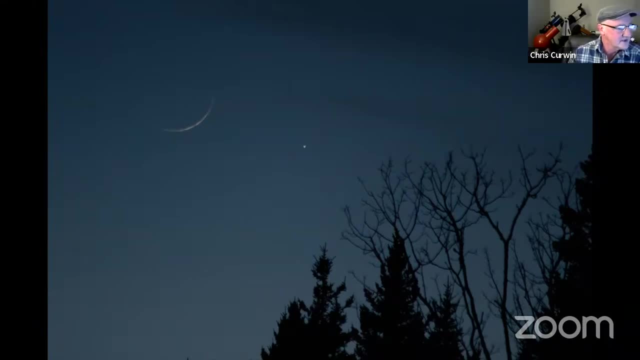 was uh sitting outside, uh, an early summer of the year, um hi, On one of the dome tents in St Martin's on Wednesday evening. I was sure I missed the new moon in the trees, which sat quite high above the horizon. I started packing up all my gear and just happened to turn around in time to see the moon and Jupiter pop into view. 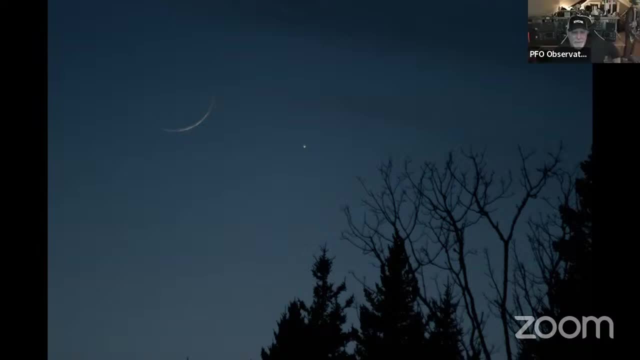 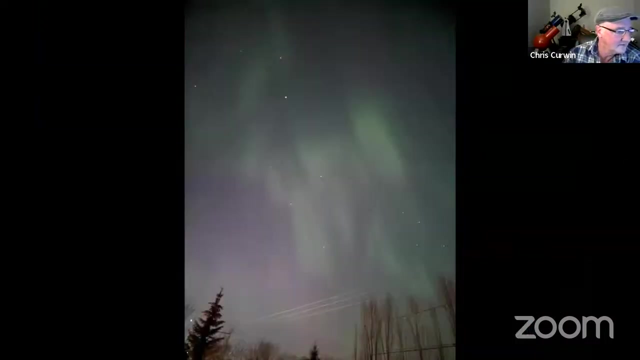 There we go. Yes, sir, 1.9% illuminated moon, taken freehand with a T6i Canon and a 300mm zoom lens, with some post-processing and dark table. Okay, Nice stuff, Here we're coming from Dwayne Schwamm. 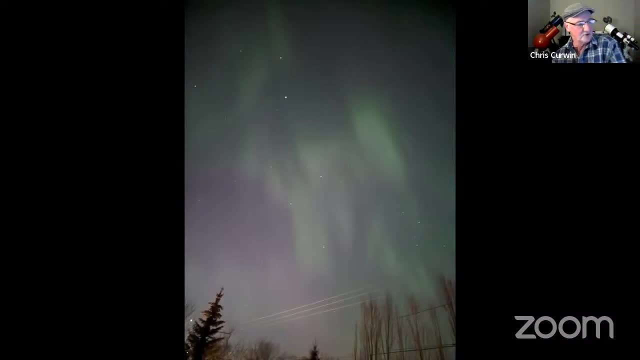 Dwayne says: hi, Chris, Like many parts of Canada, this evening we had an outstanding aurora show. That was the other night, of course. He said he could see aurora 360 degrees, including at Zenith. I've certainly seen brighter aurora, but these were among the most active and in every direction. 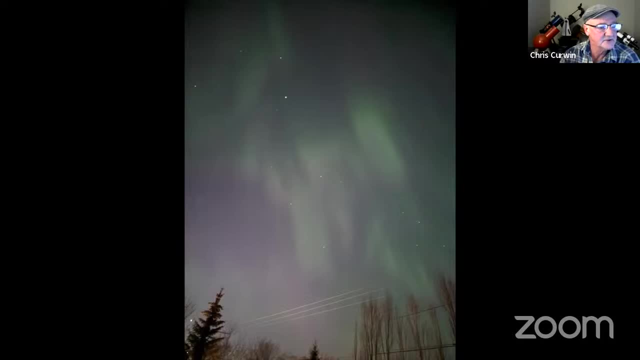 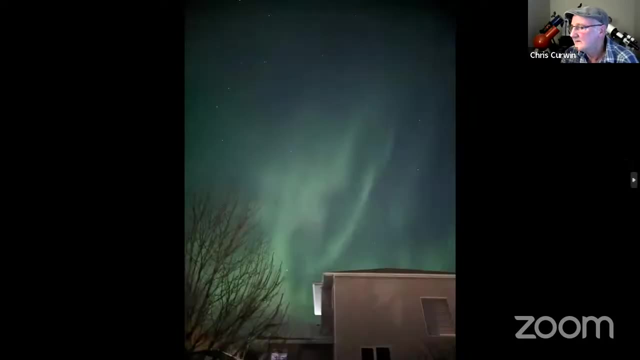 Pretty spectacular, It's worth noting. in the second picture he says you can see aurora and Orion, Everybody. let me show you that in a second There's the Big Dipper really laughing right there. Nice, I think it's making his third theory this evening. 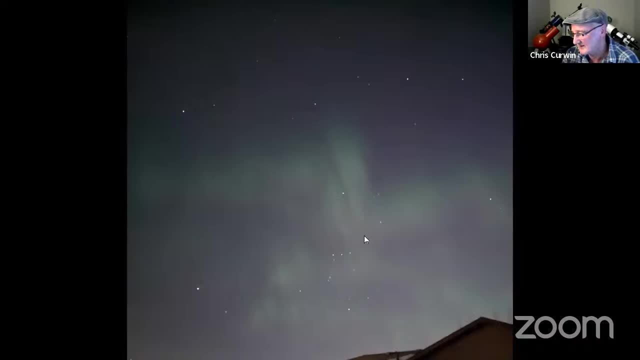 There you go. So you've got Orion in your southwestern part of the sky and look at the aurora. Yeah, I'm not sure I've ever seen both in the same view, Probably so. Yeah, I was able to share this wonder with my son and several kids from the neighborhood. 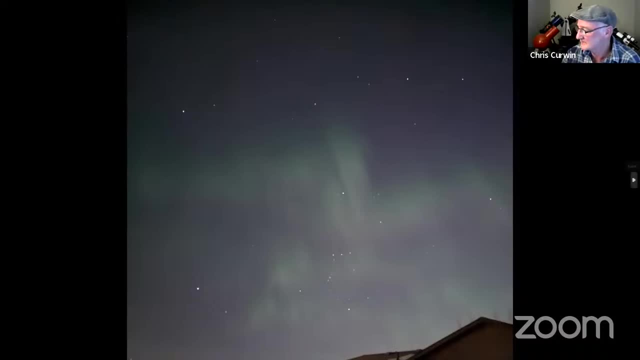 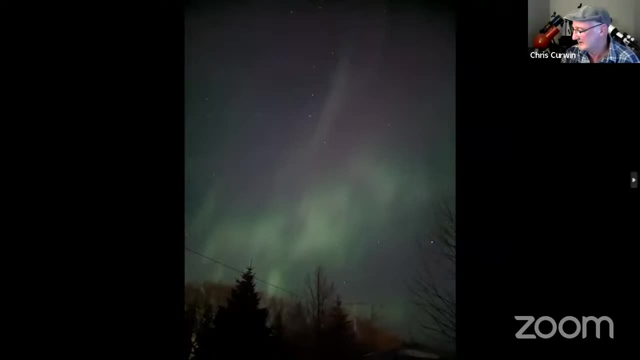 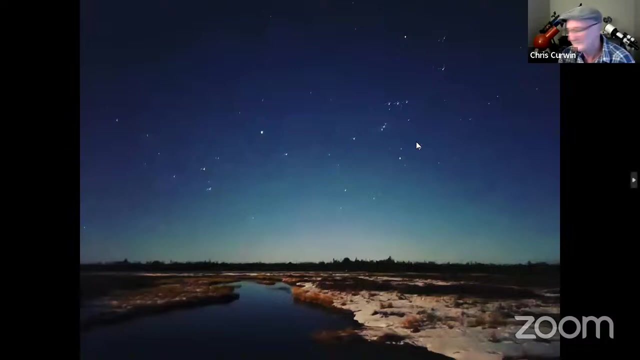 We invited out to view together, and this is from Saskatchewan. Thanks, Dwayne. Beautiful shots, Very nice, Well, awesome, Someday we'll get them here. like that, Matthew Elliott sent this one of Orion. Nice capture, that's nice. 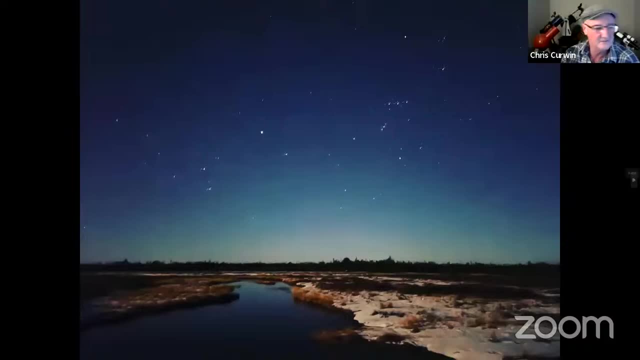 Where is it? I'm not sure. I didn't say where. he just sent it in on my page. I had posted the picture of Orion on my page and then this one was added later on with it. So that was my chance. Nice shot though. 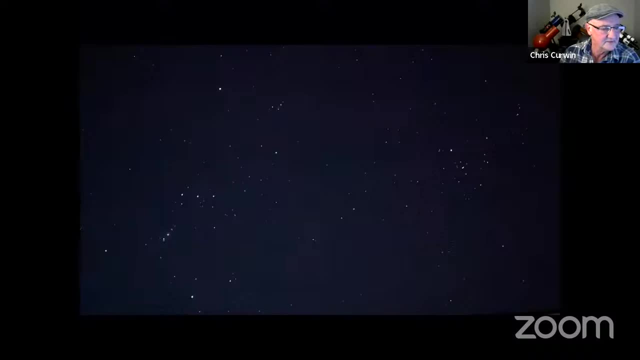 And this one came from Erica James Hemsley. She said it was a good night for pics. I got too cold and only got this one shot on my Pixel 7 Pro. Still good with the chocolate. There's Orion here again. Orion Taurus. 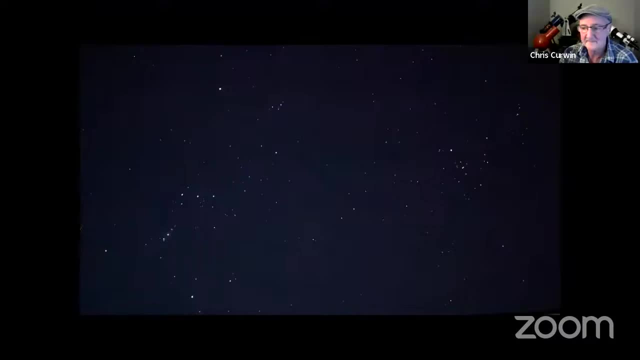 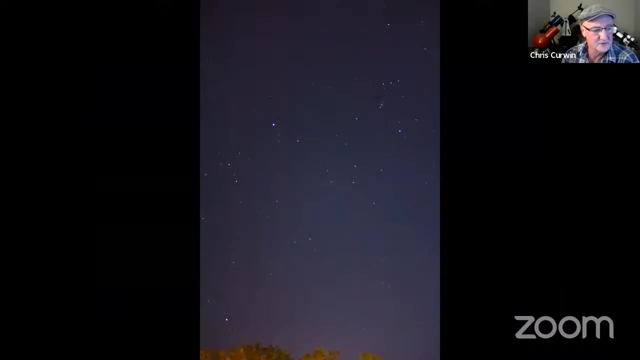 Yeah, Taurus, Nicely done. Thanks, Eric, And Carol Behan sent this one in. She said: here's a view we don't get to see from Canada: Orion, Sirius and Canopus- Canopus, I'm not sure what it's pronounced. 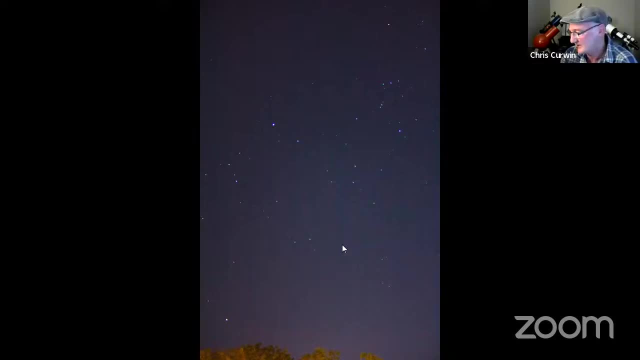 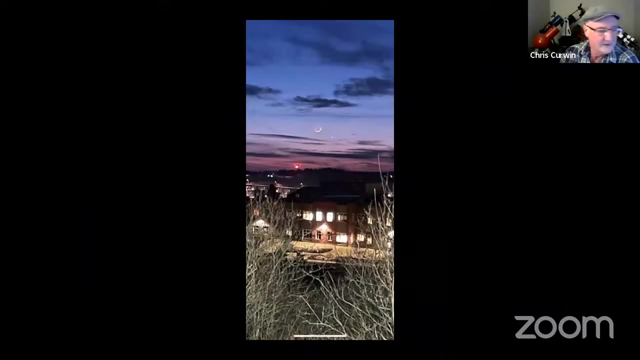 Never rises from the latitude of Canada. She said I took it. I took this in Mexico. Very nice, Nice Thanks, Carol. Kathy Shaw sent this one in the moon and Jupiter together. Wow, Sky, Yeah, Yeah, Beautiful sky. 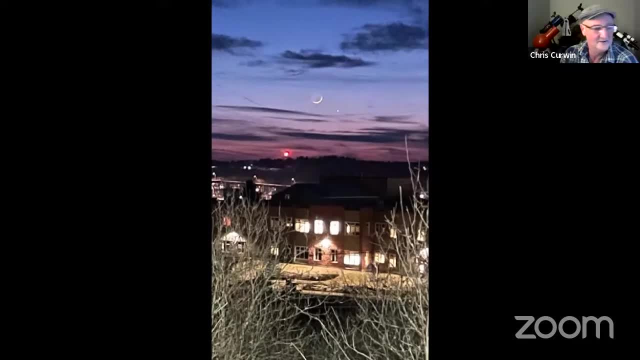 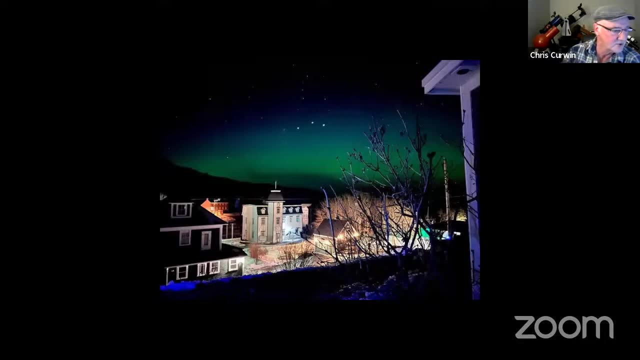 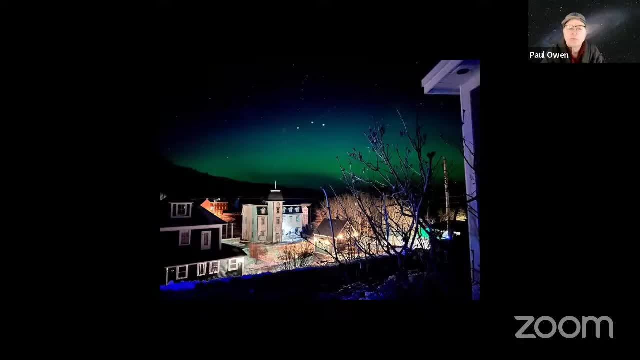 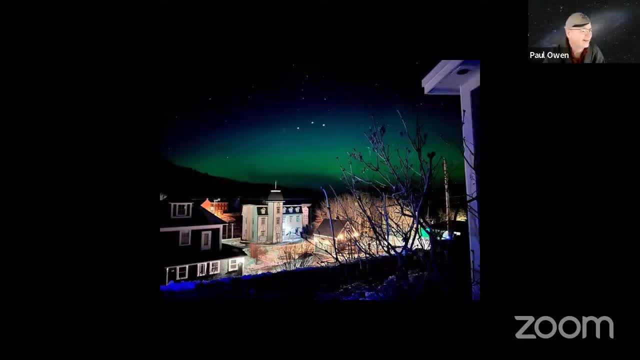 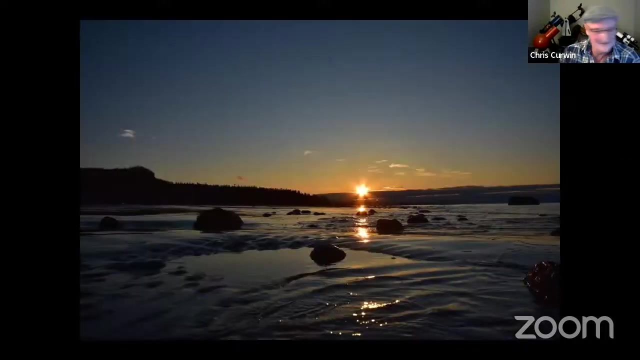 Peter's here from Toronto watching you. I can't get these guys to behave at all. Peter, Thanks for joining us. So we're all in. I don't worry, but here too much anymore. This one came from Clayton Car Sunrise from St 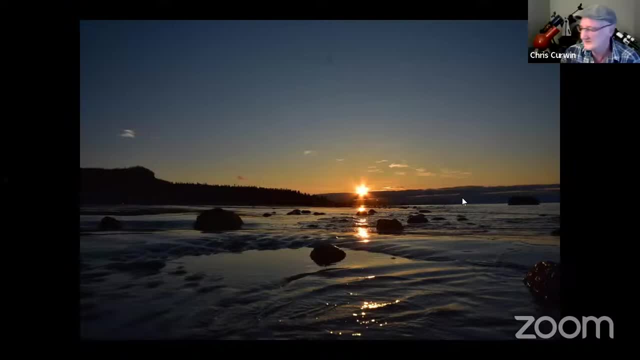 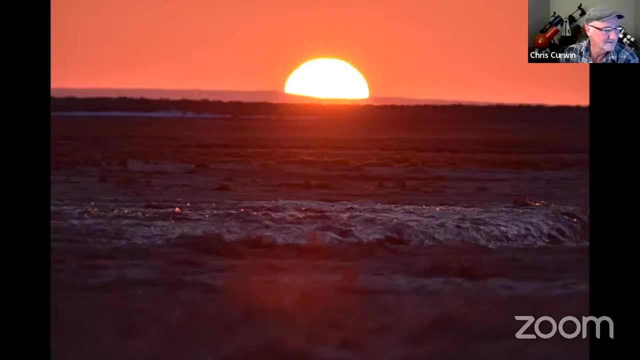 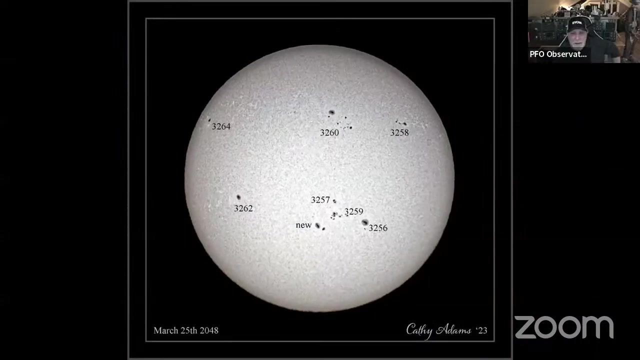 Dressed, Beautiful, Nice shot, Nice play, one he got from saint martin's. oh, it's beautiful, most beautiful sunrises down there. yeah, um, thanks clayton, um jaffee adams, this one here of the sun, yeah, getting active again when i come around the. 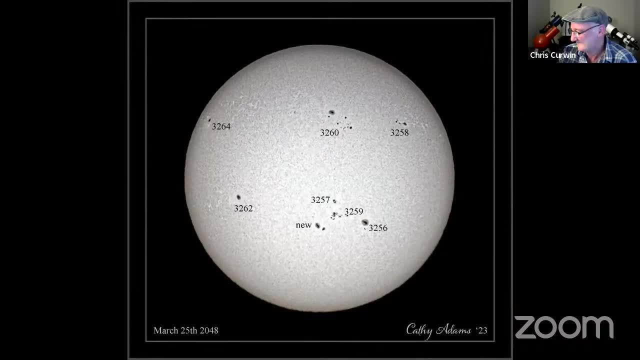 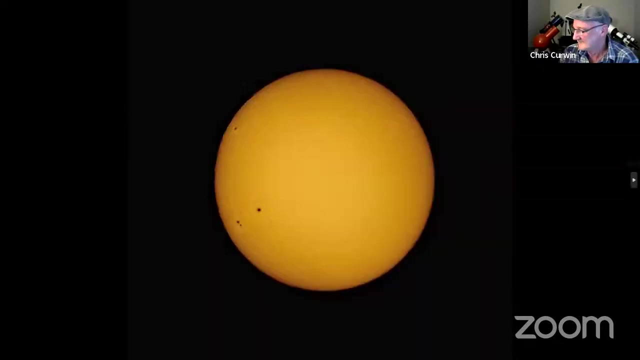 corner there. yeah, what's going on? that's here. where is that? march 25th 2048? i'm not sure what that means. maybe she's fast forwarding a little bit glitch in the matrix. let's ask her about that one. and uh, david hoskins sent this one to the sun. that's there. 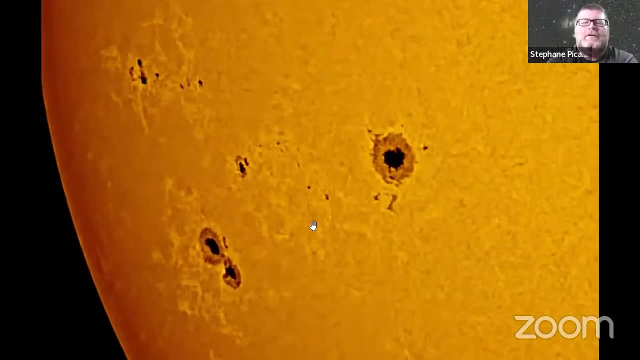 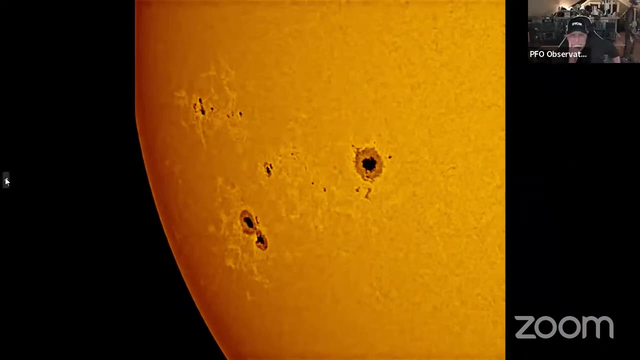 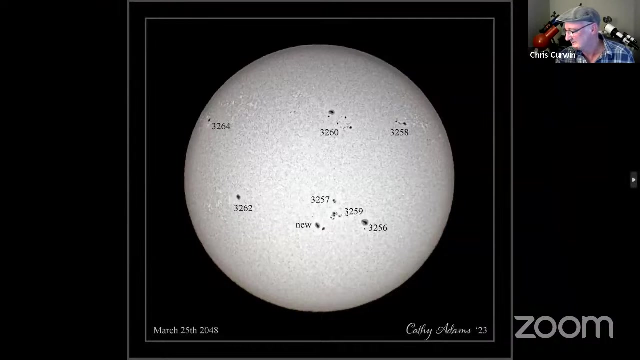 yeah, that's nice, oh yeah, nice popular there and those things are huge, they are right. just goes to show you, which this picture in the last one, how much the sun changes. yeah, hopefully it does. yeah, oh yeah, yeah, absolutely. well, that's 2048 too, so we're gonna see. yeah, that's true, that's true, yeah. 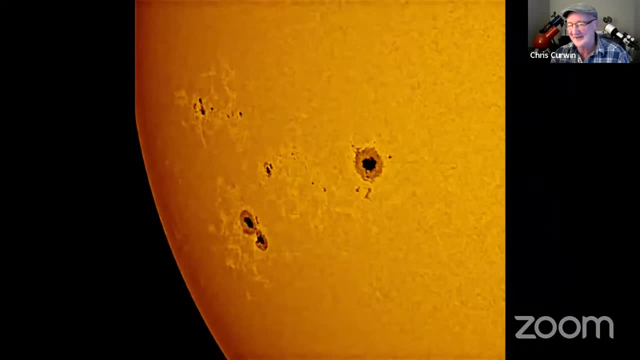 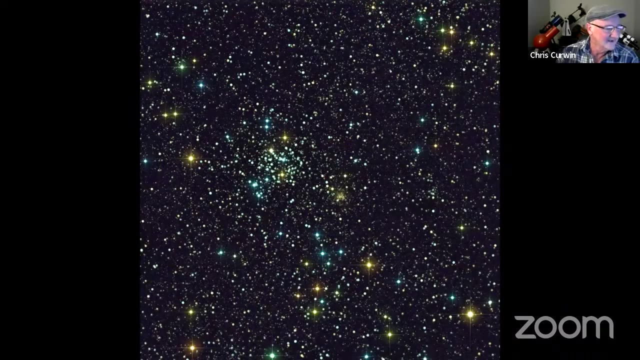 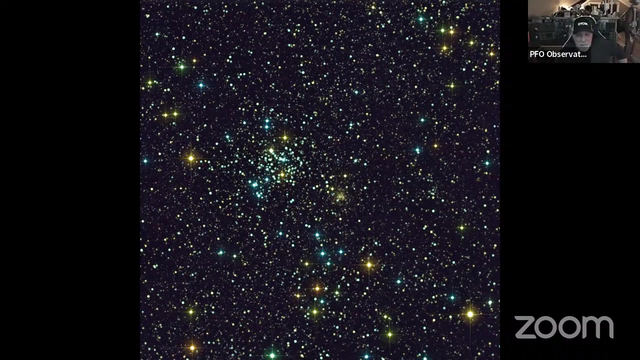 that's the next solar cycle. i think kathy take some ribbon, but that's okay. hey, joey croswell sent this one in last week's sunday night astronomy show, bundy by no buds. target of the week: yeah, and 35 open cluster in constellation gemini, gemini. yeah, that's a nice cluster, okay. 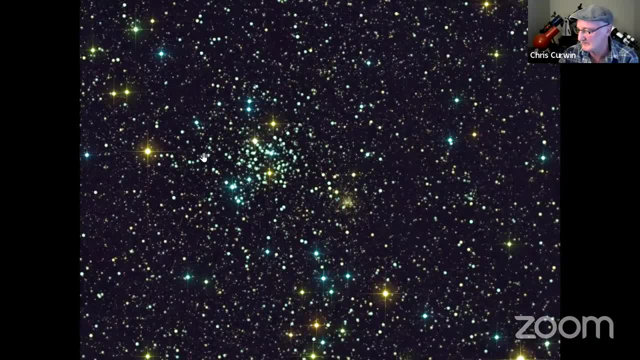 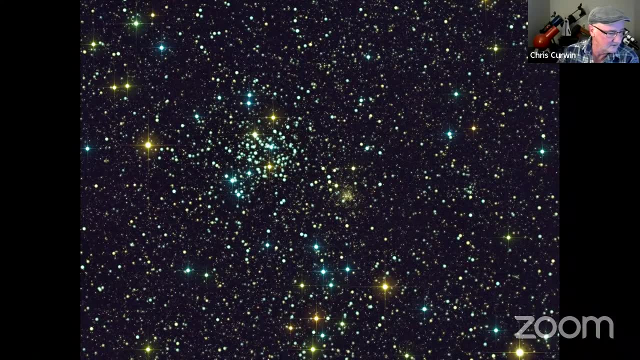 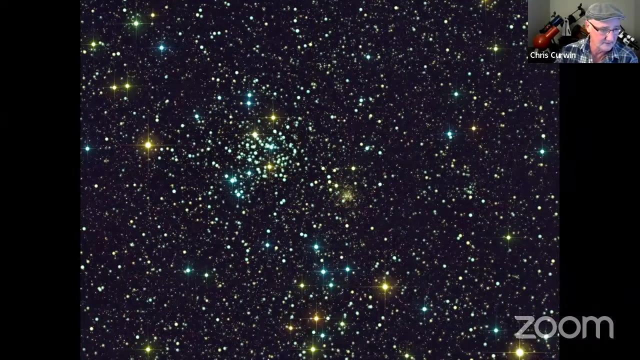 yeah, beautiful, yeah, it's beautiful. mars is going to be near, uh, near this week too. so, yeah, he did a real nice job on that. he said image using the asker fra 4000 or 400 with a 0.7 reducer at 280 millimeter, um 8 by 30 second exposures, stacked in asi air and edited in photoshop. 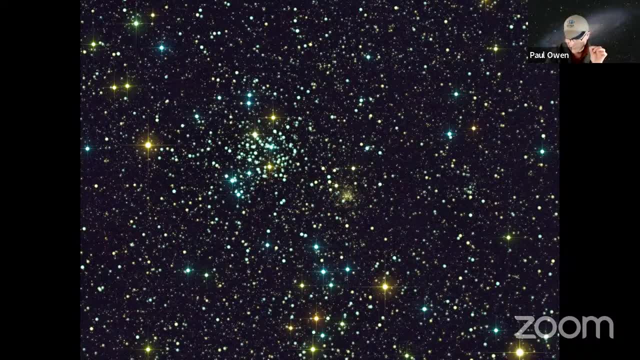 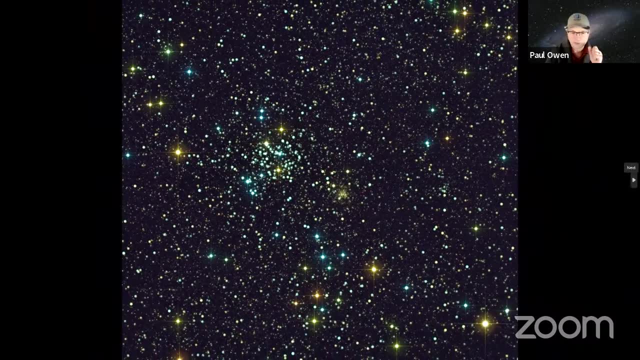 there's a nice little tiny cluster right on the bottom right at the end of it. yeah, yeah, an ngc. okay, i don't know what the number is, though the sheets are getting. see the big cluster. yeah, yeah, right there in the bottom corner, just just just. no, no, go back up to the big cluster, go. 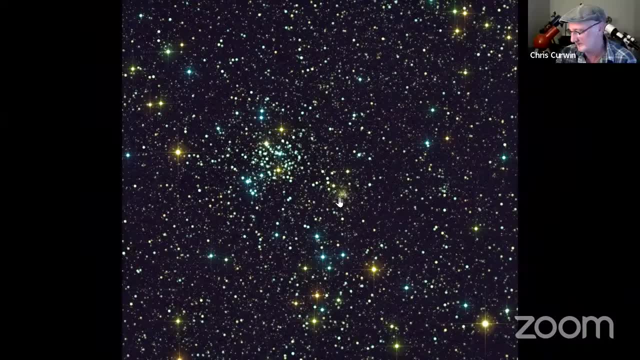 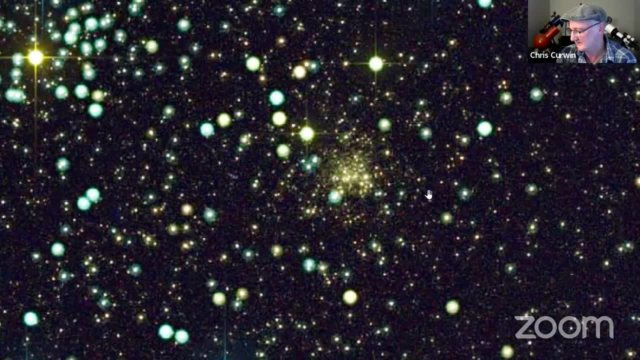 back up just slightly, go to your right slightly. oh, right there. right there, that's it. now zoom in. there's a whole lot of cluster right there. yes, light glow cluster, yeah. yeah, looks like all the same color stars too. yeah, it's beautiful. no, he captured it very well. 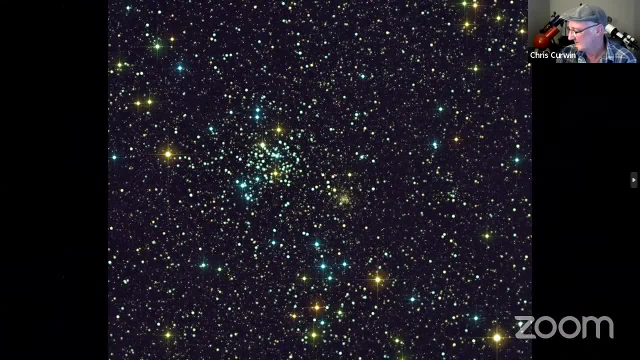 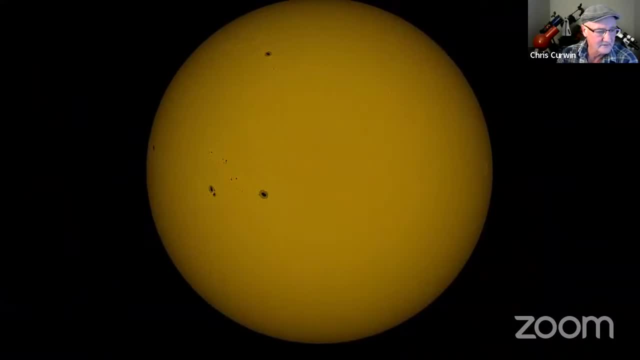 did a great job. yeah, great job, joey. thanks for that. uh, mr powell, put this one in. mr powell, or from the suns: yes, as well, that's an old one, though. last time we had the sun, mr paul owen, like the birds, would have been drawn in by the sun. he says: yeah, there you go. 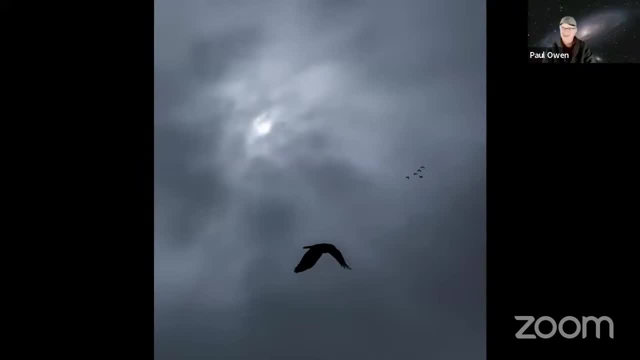 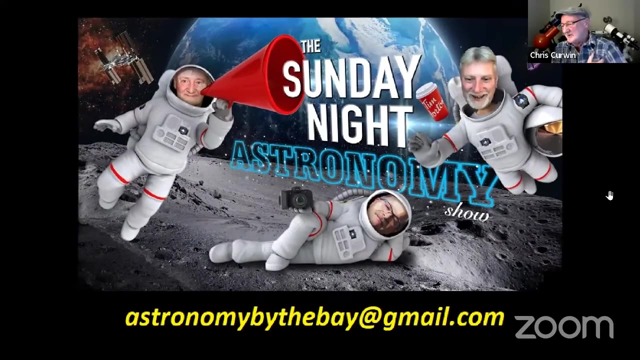 there we go. they're all going up. don't fly too close to the sun. don't look at the sun. that's a nice shot ball. we'd like to send in your photos. we love getting them, of course, here. we can send them into astronomybythebay gmailcom and we'd love to share them. so thanks for sending. 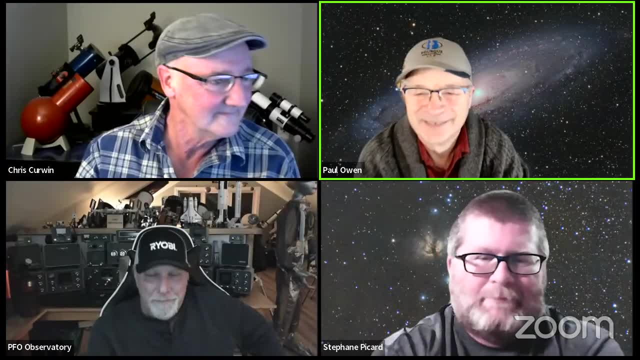 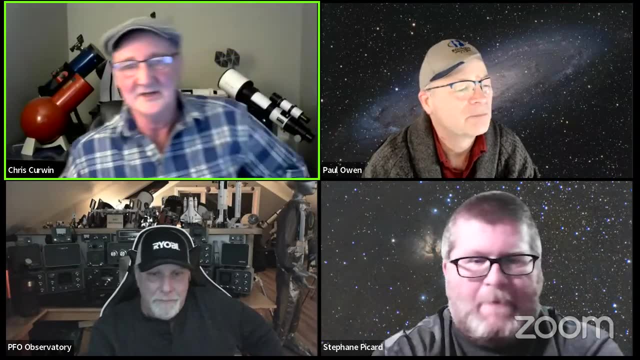 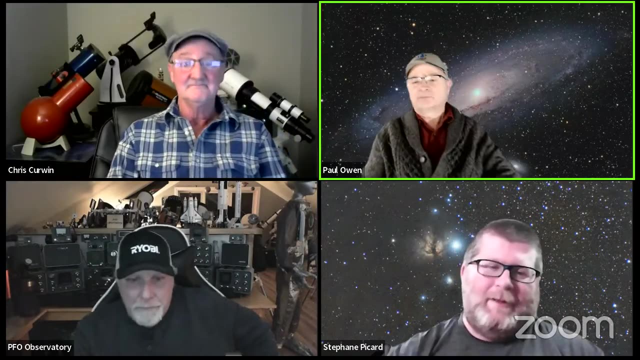 those in everybody. okay, um, just need another second here and i think we can get to our closing. so i guess, um, there, uh, kind of a bit longer show, but we've covered everything. i think pretty nice. so we covered a lot of stuff. we covered a lot of stuff. we really we were like starting to yeah. 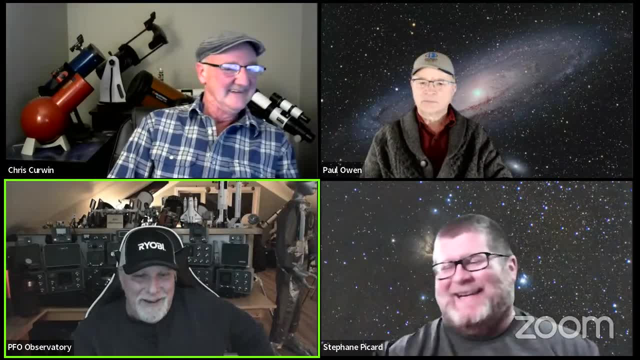 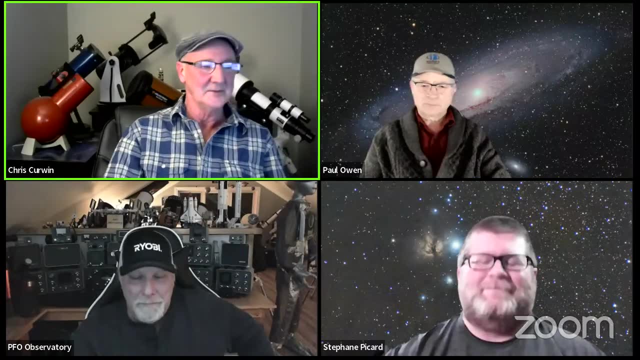 i'll put a queen size to a king size. it's okay tonight, somebody over for a cup of tea? you don't chase them out after an hour, right, right? no, not in ameritimes, anyway, no, sir. thanks again for all your support. uh, also thanks as well. 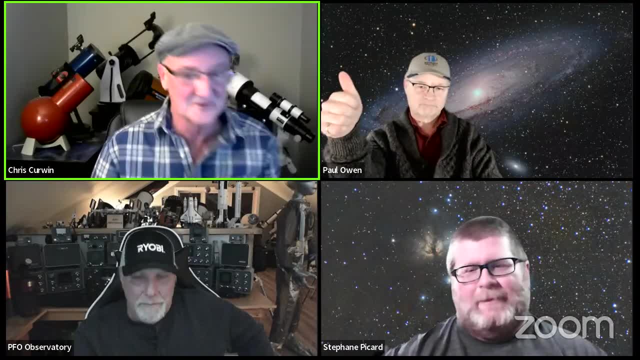 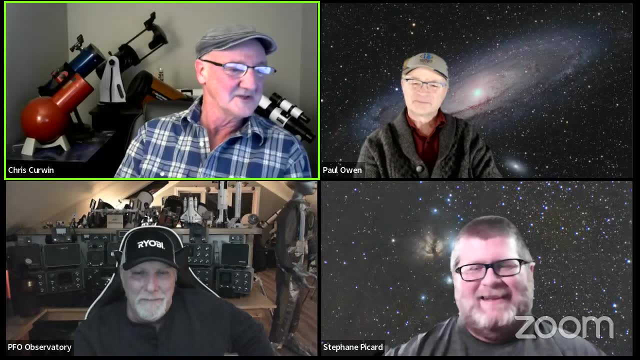 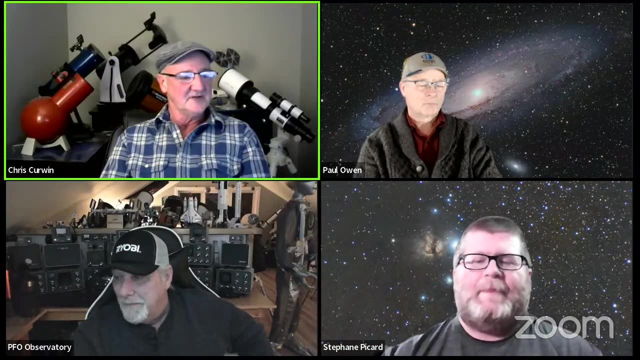 to rosanna for continued contributions to the program and to peter rissima for the music. hey, thanks, buddy. also a special thanks to live, to trudy, of course, and all of you who continually share our program for us. um, if you would like more information about the wonders of the night sky, you can find me at 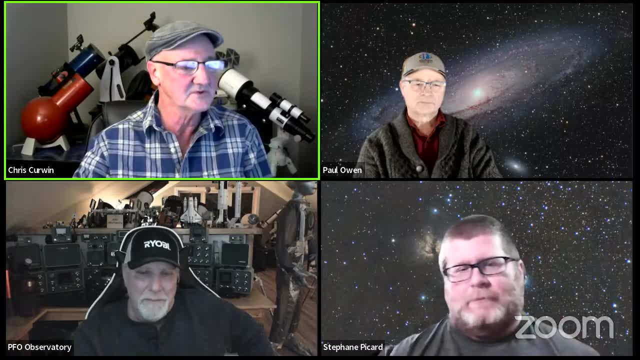 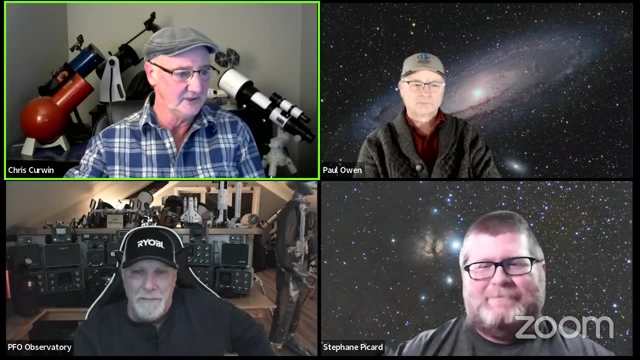 astronomybythebayca, number two. we do love getting your photos, so send them into astronomybythebay gmailcom and we'd love to include them on our next broadcast. and please let your friends and family know as well that we will be back here next sunday night at 8 pm on youtube to entertain you. 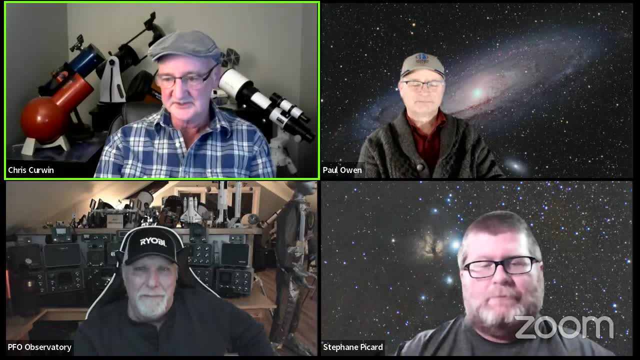 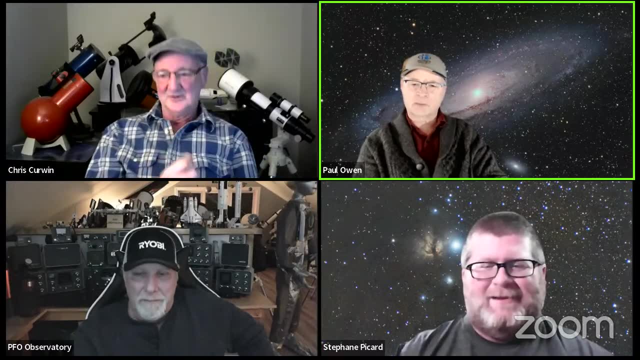 on astronomy in the mornings of the night sky. i want to thank stefan for joining us again this evening as well. so thanks, stefan. thank you, stefan, it's uh working well for you. yeah, thank you. so for now, then, from stefan and mike and